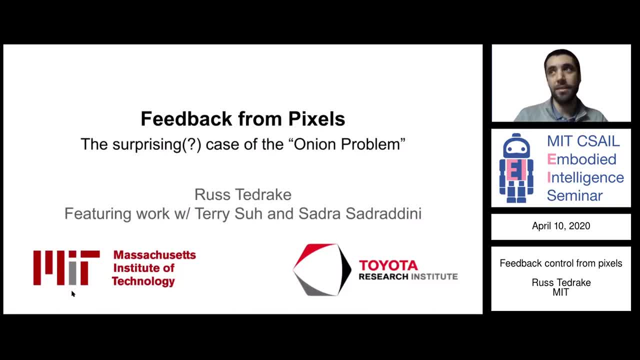 undergraduate teaching, the DARPA Young Faculty Award in Mathematics and the 2012 Ross and Joan Spira Teaching Award. He also was named a Microsoft Research New Faculty Fellow When he studied. he studied computer engineering at Michigan and then he did his PhD. 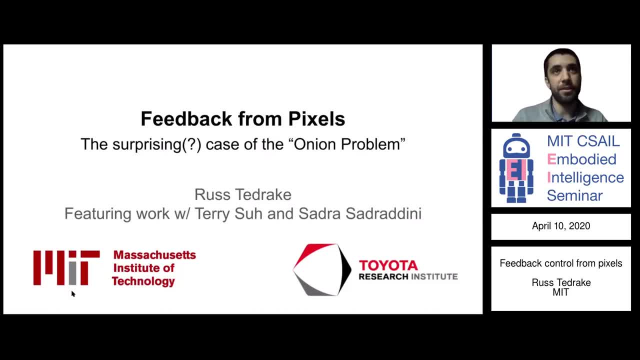 here with us at CECIL in 2004, working with Sebastian Song, And after graduation he did it at BCS, also at MIT to doing his postdoc And finally some of his education has also been at Microsoft and Santa Fe Institute. 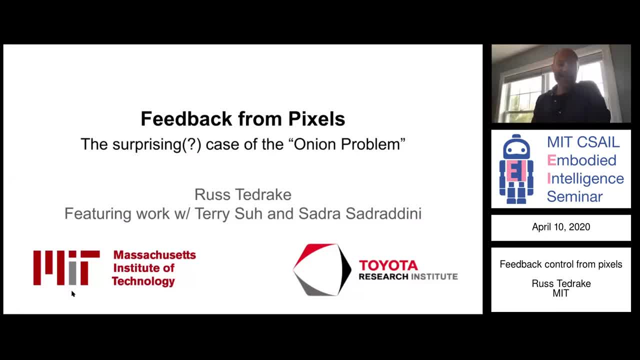 Let's welcome Ross DeDraga. Hi everybody, Thank you for coming And I'm actually more worried about talking to the void than having too many questions. So I appreciate your seminar advice, like I said, but I think you could probably ask questions and I'd be happy, or show your face and you know. 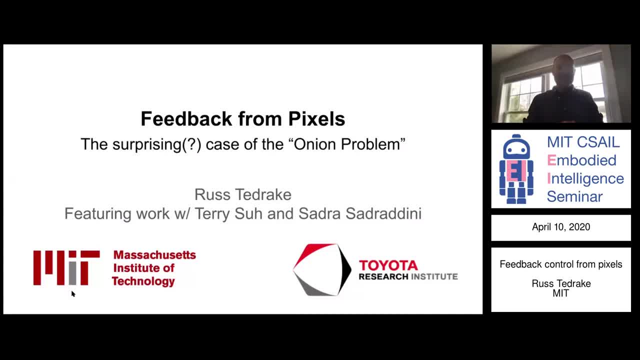 emote and I'd be happy. Okay, so I wanted to talk today about sort of a curious problem and one particular example here of an experiment we've been doing in feedback control from Pixels. But I wanted to actually have a discussion. ideally, if the format works, The original idea. 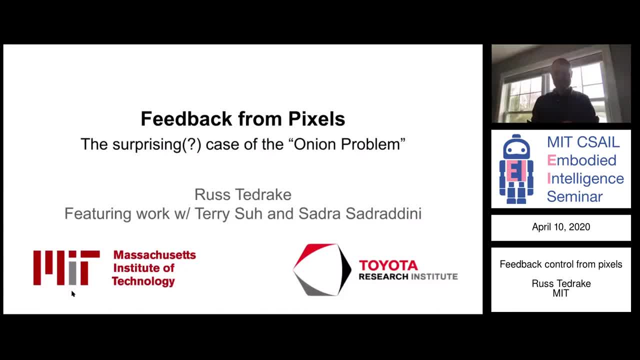 for this was a chalk talk and we just have a few people sitting around and talking it out. But you know we've so far. I feel strongly about the fact that you know we've so far, I feel. 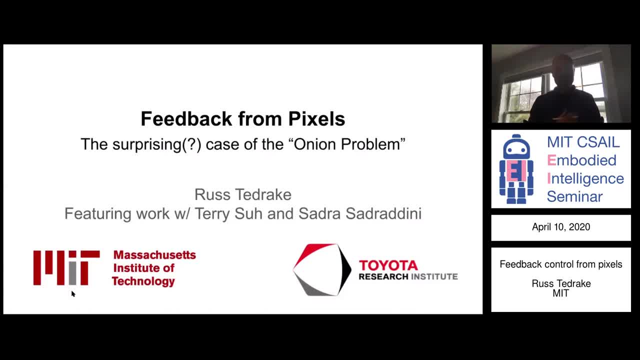 strongly about the fact that you know we've so far. I feel strongly about the fact that we've struggled to do rigorous control from Pixels And I don't know that we really understand why, And so I want to just dig into that a little bit today and talk that out and see if we can start. 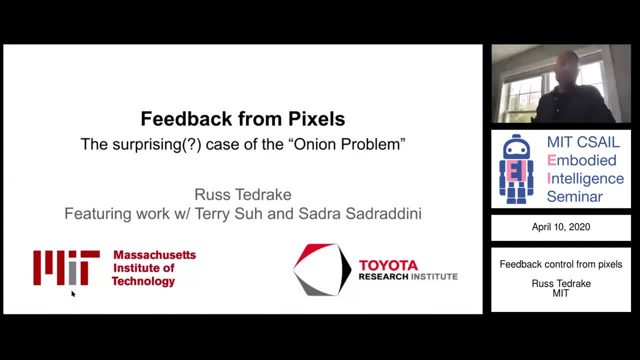 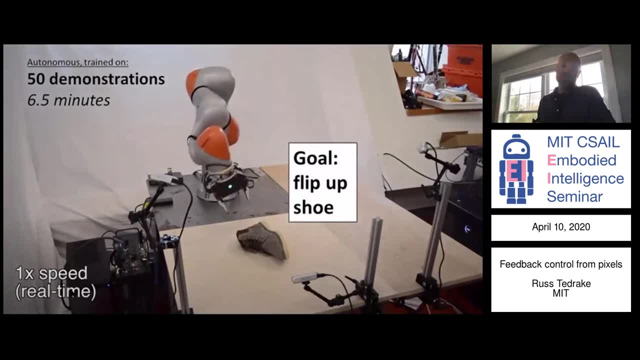 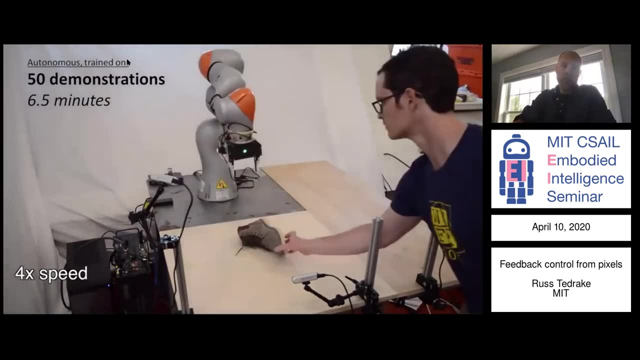 making some progress. Okay, so what do I mean by feedback control from Pixels? Some of you have seen what I hope is starting to play here. Good, This is also an experiment in presentations here. This is Pete and Lucas. This is Pete and Lucas. 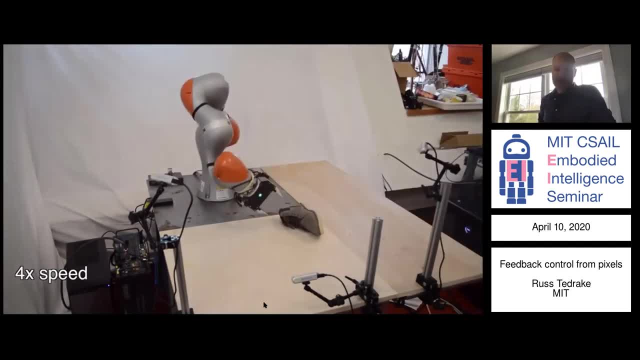 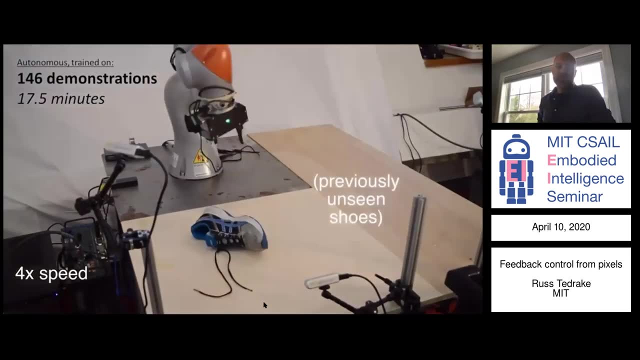 Showing what can be achieved if you actually close a tighter feedback loop with a depth camera. in this case, right Is the ability to sort of interact with- in this case, a variety of objects and have the richness of a perceptual input, but have the 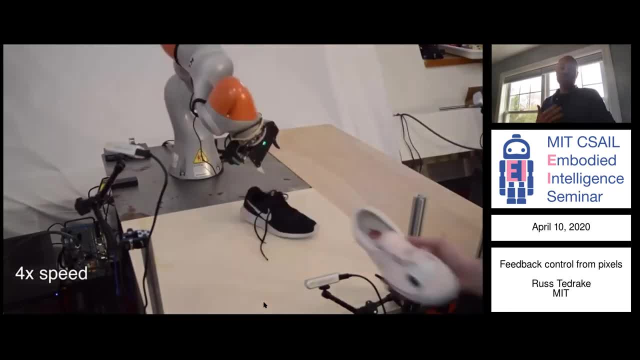 closed loop update rate that you'd expect and you can sort of get much more reactive, much more robust feeling behaviors, And I think this is a really really useful feature that we've developed over the years for, admittedly, a kind of a silly task of just trying to flip up a shoe. 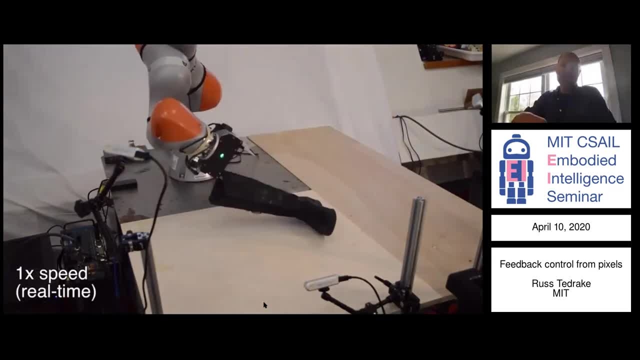 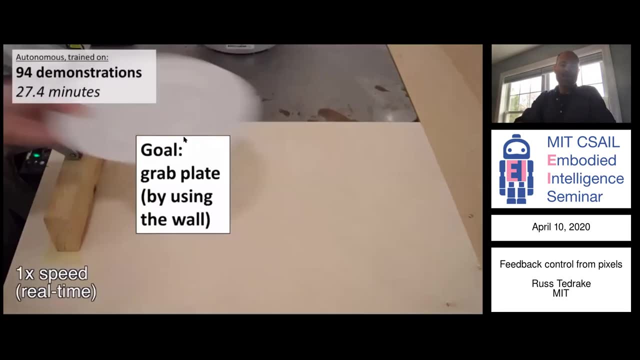 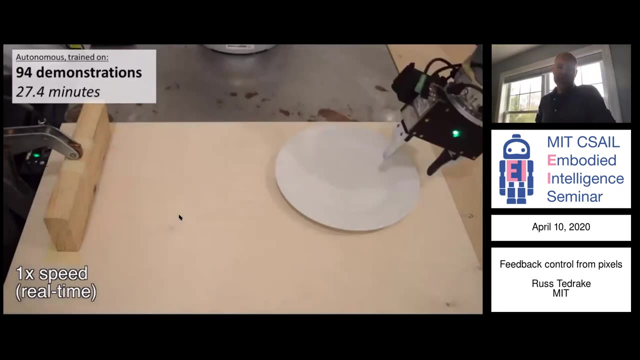 but we wanted to flip up any old shoe. Okay, we did an open house not so long ago. for those of you that came, It works well. It works sort of surprisingly, almost frustratingly- well. This was the, you know, a non-trivial contact task with a policy that was using visual inputs. 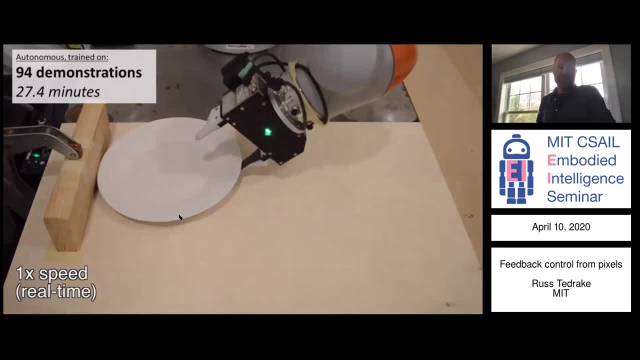 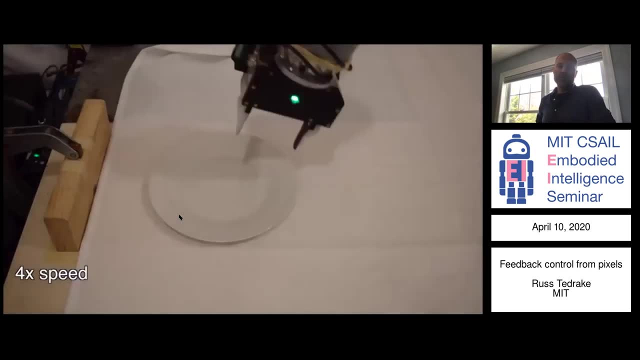 primarily kind of the same thing: Commanding end effector positions and doing non-trivial tasks. This one was trained with imitation learning and we'll talk about that. But boy, once you start getting these things to work, it feels so exciting. 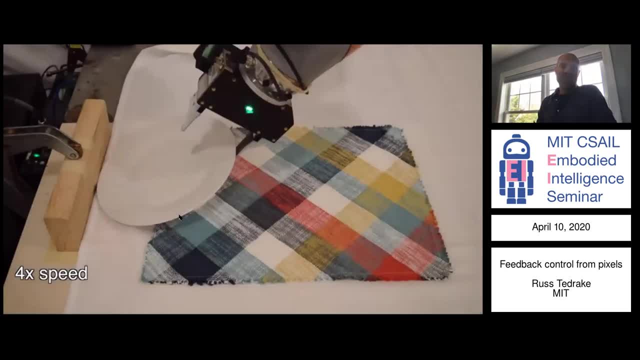 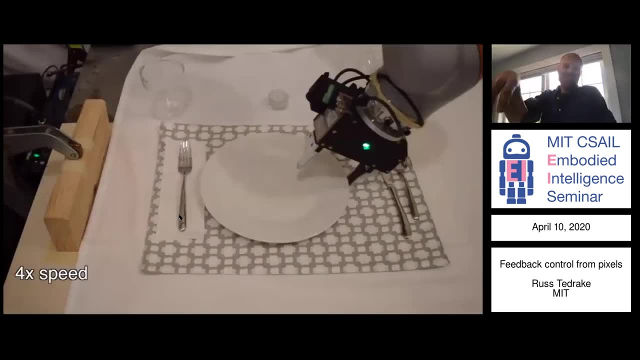 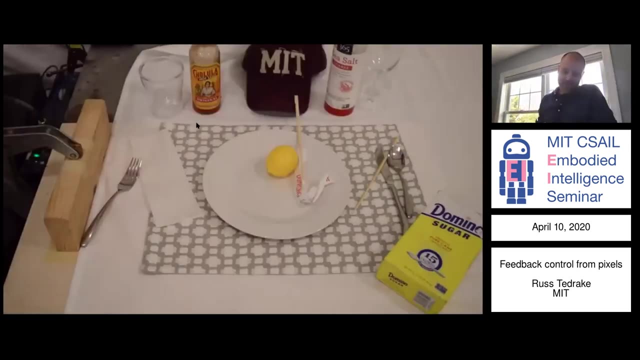 and it's like how could we go back, after something like this, to the, you know, to the times where we had our robots basically sensing, planning, acting and airballing with their hands? My ability to control is somewhat limited here, but this is just a couple of different views of that. 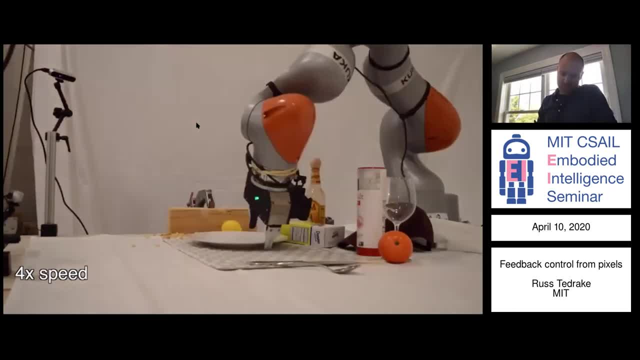 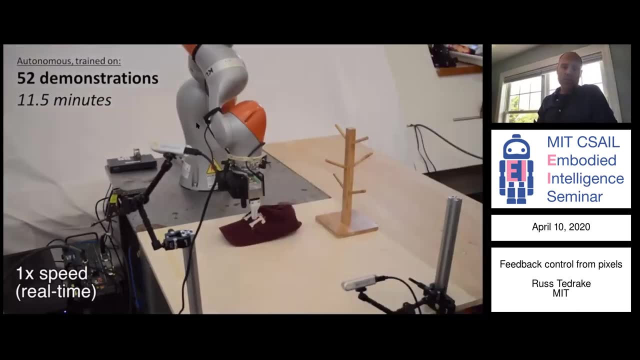 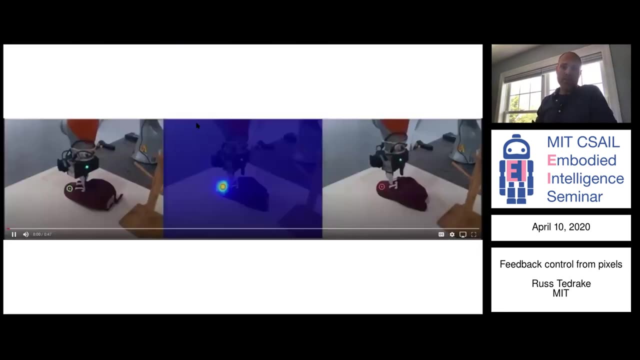 I wonder if I can make it better. Oh, here we go. This is showing that it works for surprisingly deformable objects. Okay, and this is some of the back end of it- was that one of the primary visual effects that we had? 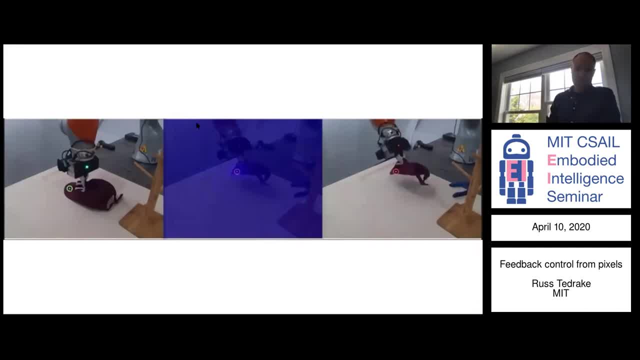 Capabilities that enabled this was this training of correspondences. So if you see, the mouse is sort of over on the left frame, a particular point on the hat and then, despite the hat being in very different configurations before, there's a highlighted area of the network, recognizing the most similar point on the 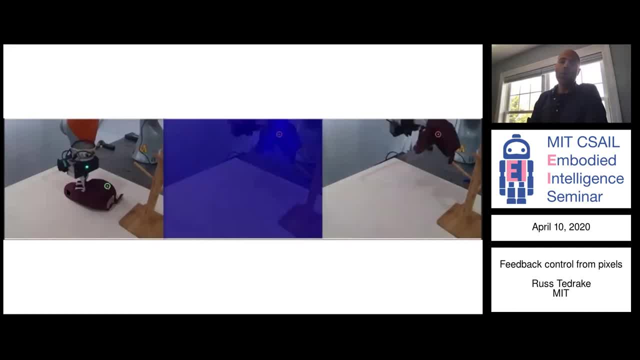 hat in the new image, Okay, and that was the sort of core coordinate system, core framework that we used in order to close the feedback loop, And I'll tell you a little bit more about that, Okay, but actually I won't tell you too much about that because Lucas is going to defend its. 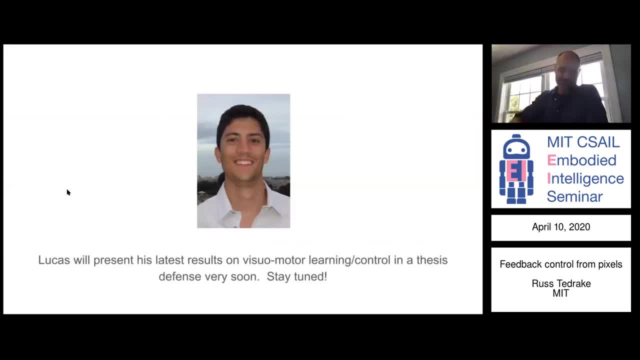 thesis fairly soon And I highly encourage all of you to attend his talk. He's got more results since then and it's going to be a great talk soon to be scheduled And I hope you tune in. But one of the things that I think Lucas would say and that we say together is that it's sort 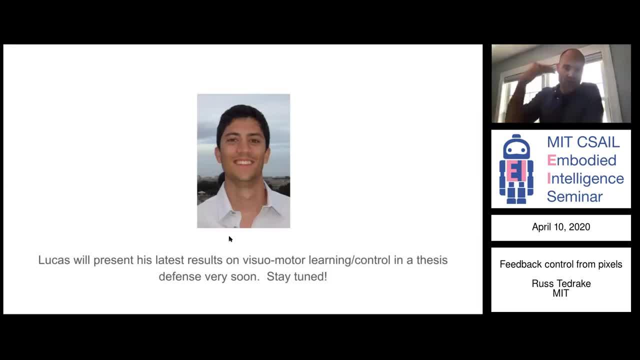 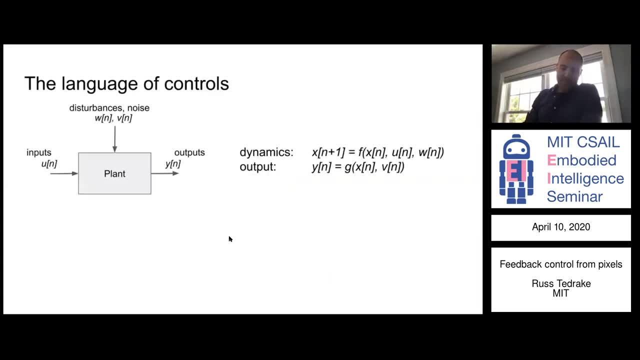 of frustrating that, although that works very well and it's certainly a feedback loop and it's certainly doing dynamic substitution, Okay, Lucas will say and I know Lucas would say, and we say together control kind of things, it's really not built on the fundamental tenets of control in the 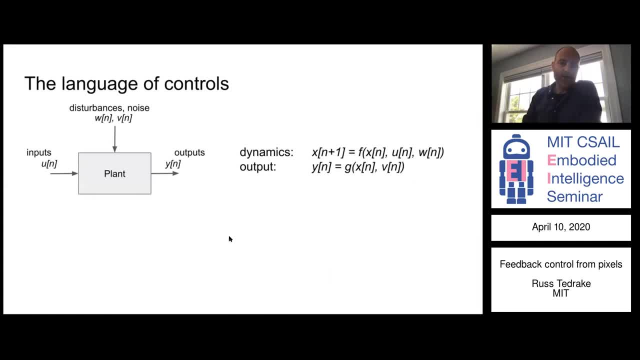 way that we'd like, right. So there is a language of control that goes through models that talks about, for instance, I have a plant with control inputs U, with outputs Y has some internal state X. I'm just putting these down so we can have a common vocabulary through the talk. okay, with disturbances. 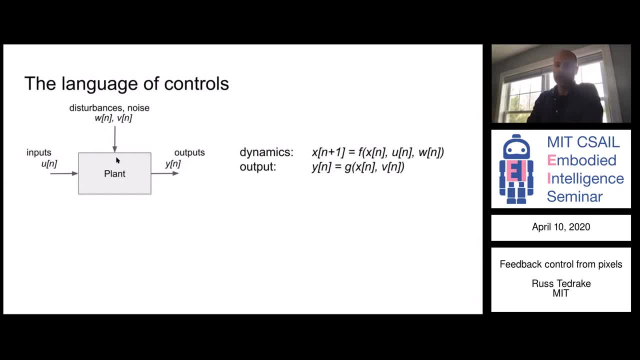 coming in as W and noise coming in as V, okay, And then I've got too many computers here, okay. And then my goal is to try to find a controller, which I'm going to call pi today here, which ultimately is going from a history of observations Y into a control action U. right. 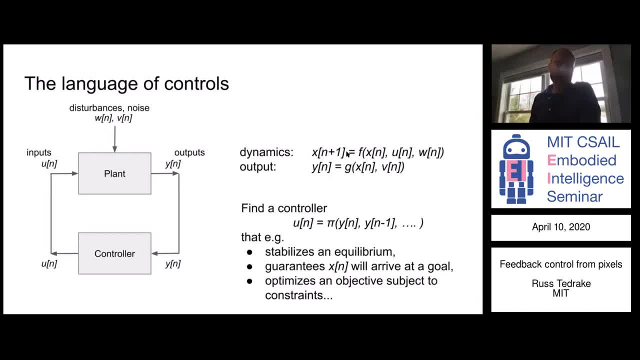 And there's many different ways to try to tell the system which kind of which pi I'd like to find of the many to choose from. Maybe I'm trying to solve it, Maybe I'm trying to stabilize an equilibrium, Maybe I'm trying to guarantee that my state will arrive at some goal. 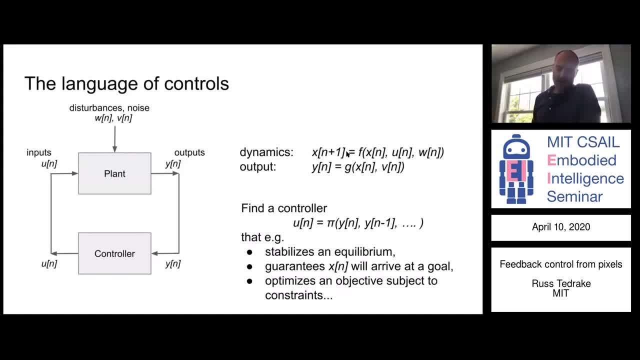 Maybe I've formulated an optimal control problem and I'm trying to optimize some objective subject to constraints, right, Lots of different ways to think about that, all in the service of trying to find some policy pi okay, but I've never, ever seen any proofs that sort of say: if G happens, 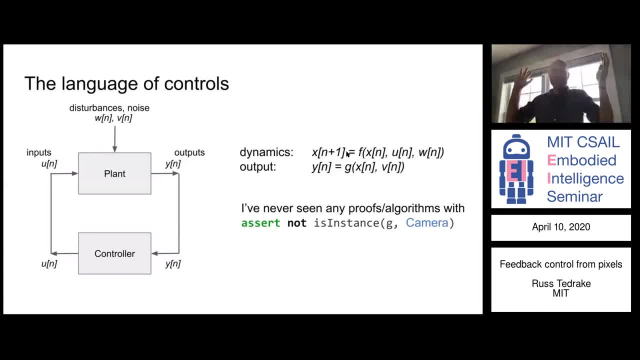 to be a camera right then. then pff, stop. Nothing works right. In fact, one of the things that drew me to controls in the first place. I remember when I came to MIT I had been doing a lot of reinforcement learning and as I joined the faculty I started. 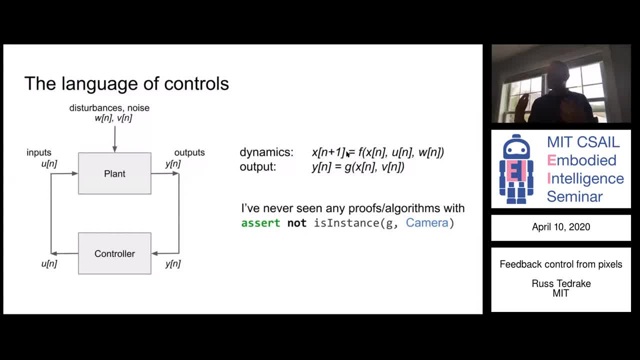 interacting with the controls faculty even more, and it was so compelling to me that I felt like every question I had. you know they could view almost anything as a systems theoretical problem And they almost always had thought deeply about the systems theory enough to apply it. 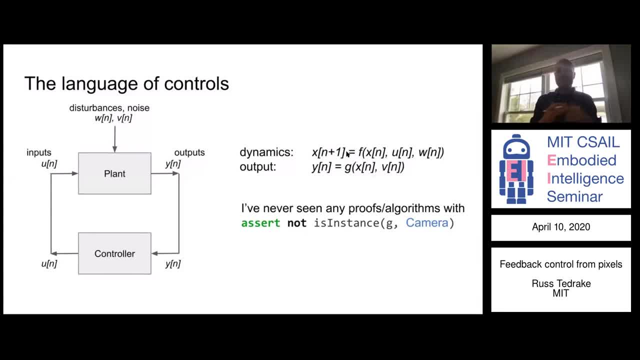 in a way, to the problem, Yeah, To a new problem. So pretty much everything you could take to Sasha Magretsky or Pablo or somebody- they've already thought about that in some deep way, right, And that's like that had a major impact on what I wanted to do. 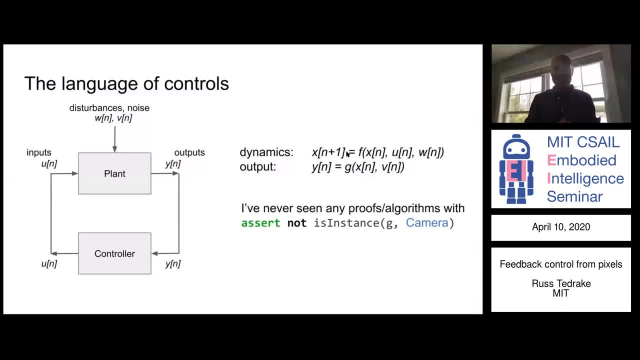 Except cameras, Like as soon as you say cameras or computer vision, there's kind of like whoa, whoa, whoa, you know, controls doesn't do cameras, That's a whole. that's like go to the other department for that. 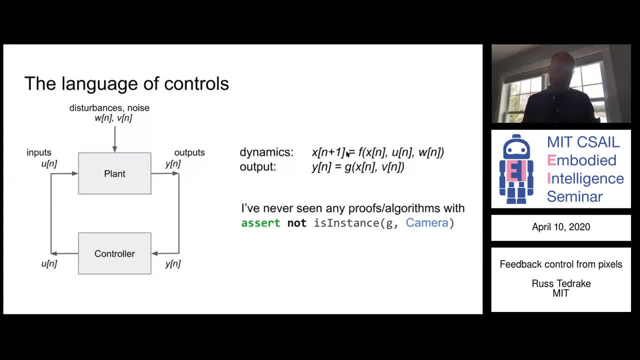 So why is that? I want to dig into that a little bit today. right, You could argue that maybe it's because once we have a camera, we start trying to do more ambitious problems, and maybe we're in situations where we don't even know what F is. 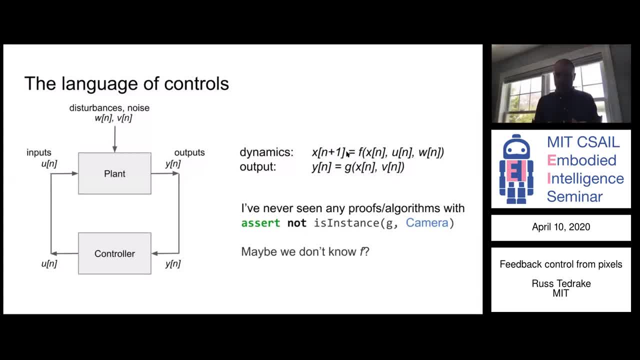 And maybe that's the fundamental thing that happens. But I think there's plenty of places where we know F okay, where I know the dynamics. But even if I give you a perfect simulator- let's say, Michelle's working on a robot trying to tie shoelaces, for instance- 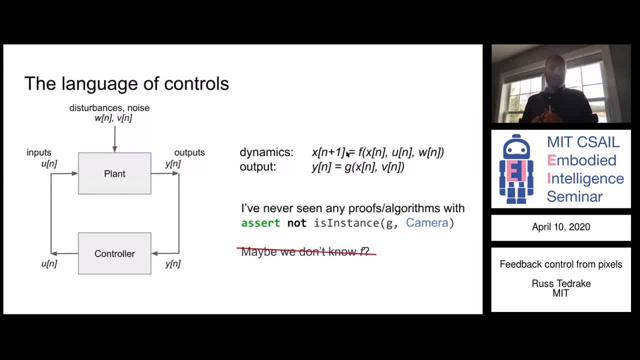 I think we can build a simulator that is high fidelity enough of tying shoelaces. It's not easy. I think if we can get things to work with a simulated camera on a simulated system over a variety of shoes and simulation, that I'd have confidence it's going to transition to reality. 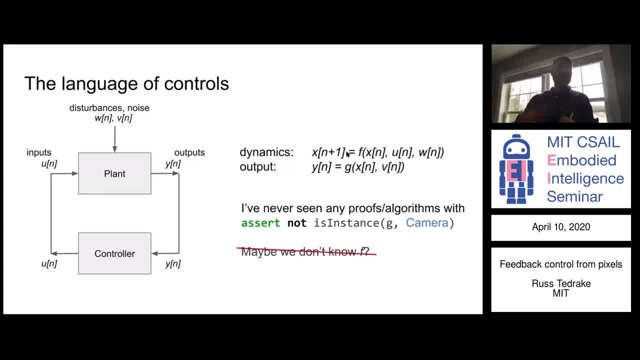 so, although there are certainly some problems where the model is unknown, I think there's enough problems that you know that I'm willing to give you f and you still can't solve the problem if the, if the feedback control has to be closed through a camera. so let's talk today. I'm not saying that's. 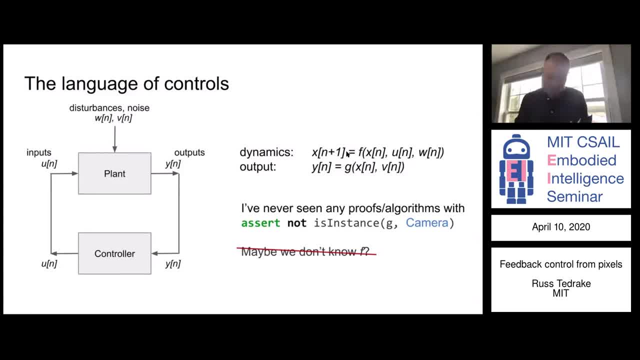 not a good problem, but let's today assume that f is given, okay. so so what is it then about g? and or, you know, if I'm willing to give you f, I'm willing to tell you g, I'm giving you a model for perfect model for g. what is it about g that makes- if it's a camera, makes- things so hard. 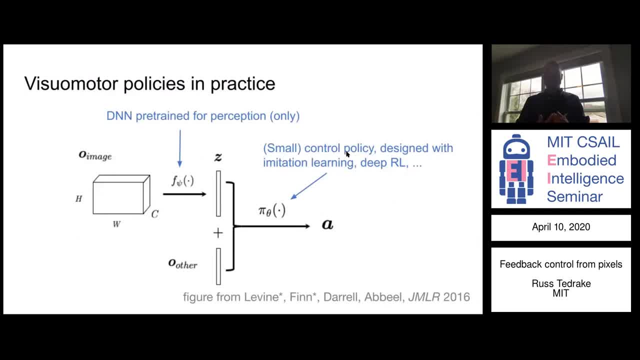 right. in practice we're not using the full toolkit of control. it's not that we're designing pi in these control theoretic ways. we're often doing things that involve, for instance, separately training a perception system with some you know big, deep network trained for perception only often, and that's often a huge network of resnet. 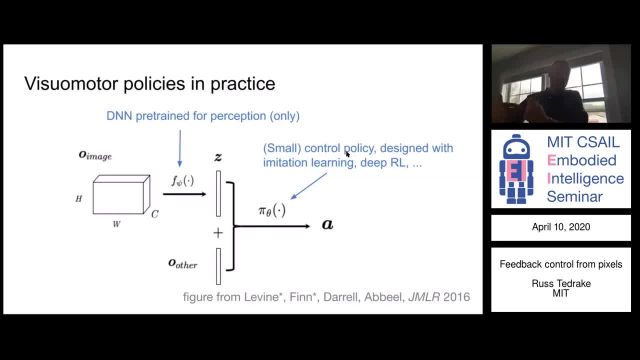 or something like this, and then we're tacking on a small policy that we'll train with either imitation learning or deep rl or something like this afterwards, and in many cases I think they are relatively inefficient, to synthesize. maybe they're hard to trust. you know, it's not. 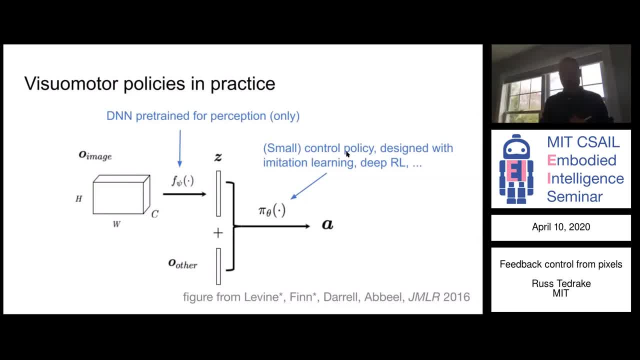 even really clear how well they work right. I would say that about our own work as well as everything. so I think the next few years is that we're gonna see some us being able to do better in this problem and I- and I think the topic you know- I'd like 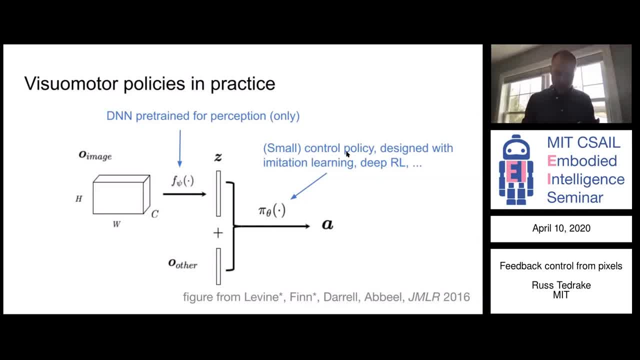 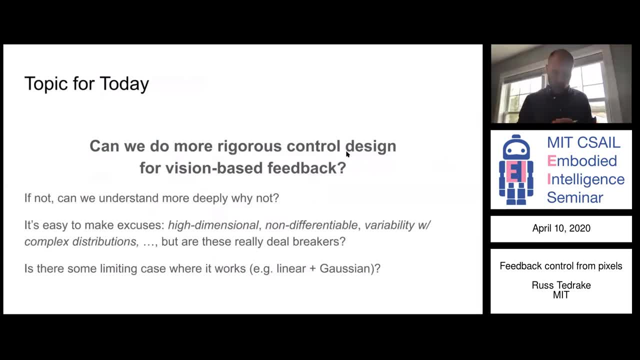 to talk about today is: how do is control theory up to the challenge? can we, can we bring some more tools from rigorous feedback control, division based feedback, okay, or if not, you know that I don't. I hope that if the exploration ends up- and I know you really can't do that, but at least 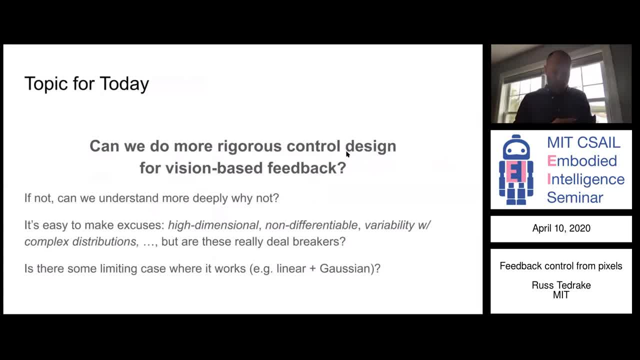 I'll understand in a deeper way why that was. I think there's lots of things that people say. it's like it's relatively easy to make excuses, but as you're excuses right, The image is suddenly very high-dimensional. G is non-differentiable. 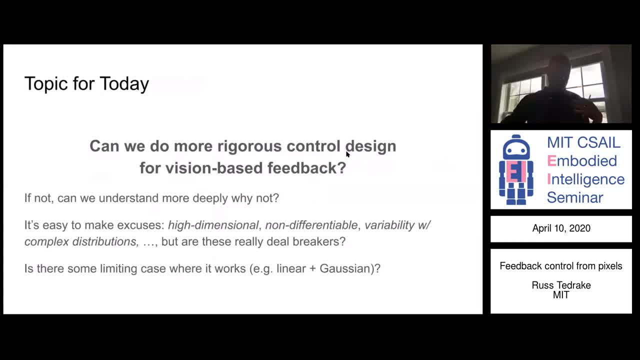 you know the variability in the outputs is. you know there's huge complex distributions over the type of visual environments. Yes, I mean those are all true. maybe, but not always. We can find examples where we want to close a feedback loop from a camera, where those aren't necessarily. 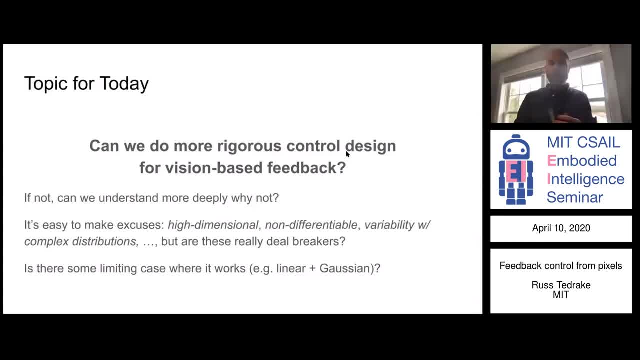 the case, We could isolate those and start asking: are any of them actually deal-breakers? And I don't claim to have any of these answers here. This is a discussion where everybody's muted and you know mostly just me talking. But if anybody wants to talk, that's great. 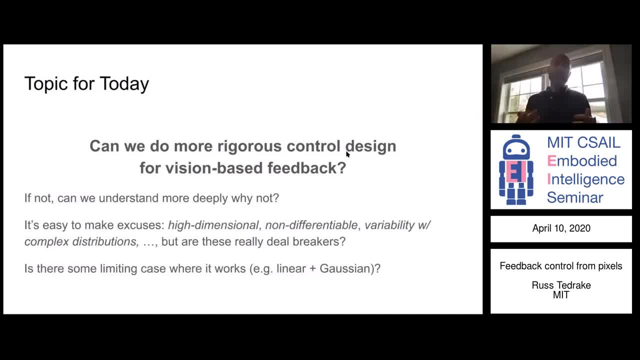 It's a discussion, Okay, and in particular, maybe one thing I will offer. we've been struggling for a while to try to find, like, what's the limiting case, where everything is simple, Like, is there a problem in vision, where you know it's like the linear Gaussian case or the simple tabular. 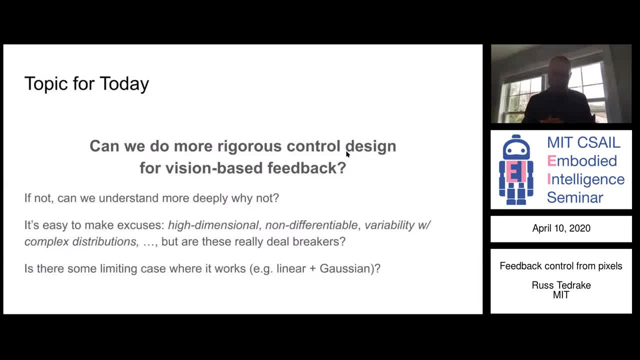 MDP case or something like that, And I think that's a great question. I think it's a great question And I kind of I feel like we found a bit of that in this onion problem, which I'll tell you about in a second. Okay, so let me set it up with a little bit of the framework, If there's. 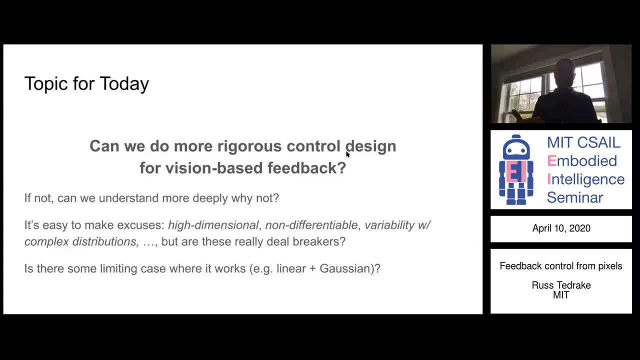 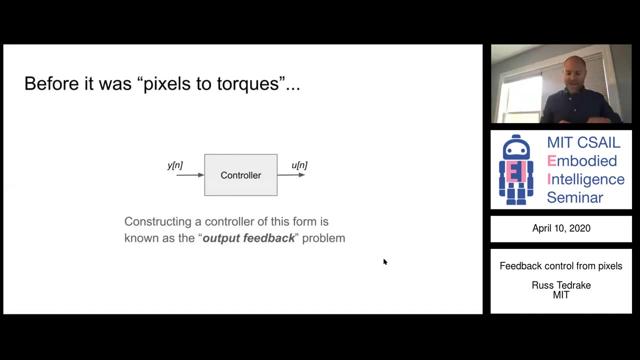 one thing I sort of want to communicate is that there are some tools from controls that we should be trying that may or may not be on your radar, right. So before we called it pixels to torques, did that transition? All right, there we go. Okay, I hope that doesn't have to happen very often. 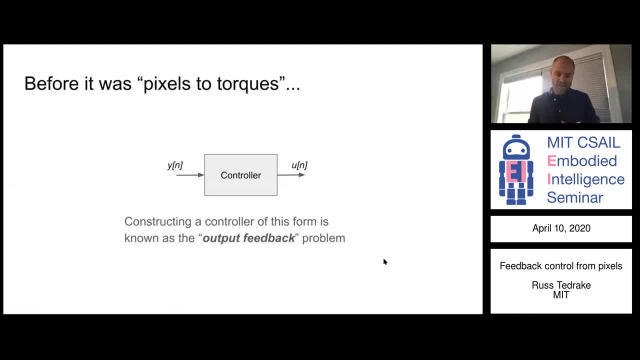 All right, before it was called pixels to torques the problem of designing a controller that goes: takes some observations y and that's a whole sequence of observations in this block diagram. there's a signal y coming in and you're going to put out. your job is to put out a signal. 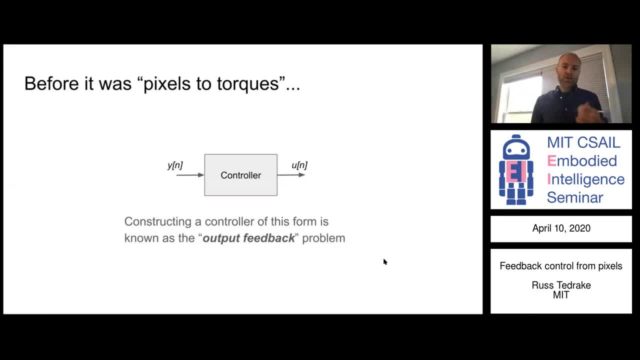 u coming out as a controller and constructing a controller of this form which, potentially, can use all of the information of previous y's. that's called the output feedback problem. okay, And the most common recipe that I think is going to be used is the output feedback problem. 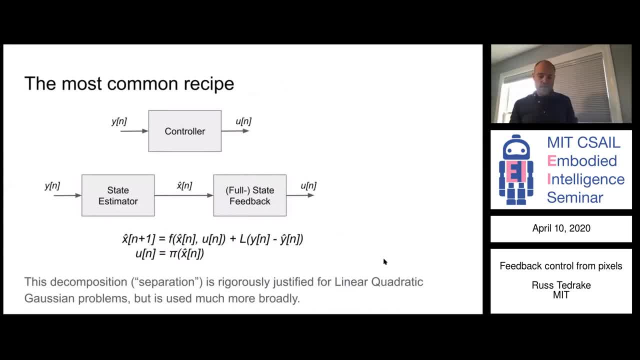 And I think we all know, is this idea of doing state estimation and then feedback, full state feedback, right? So in the particular case, well, in the particular case of linear quadratic Gaussian problems, the separation principle is rigorously justified, but we use 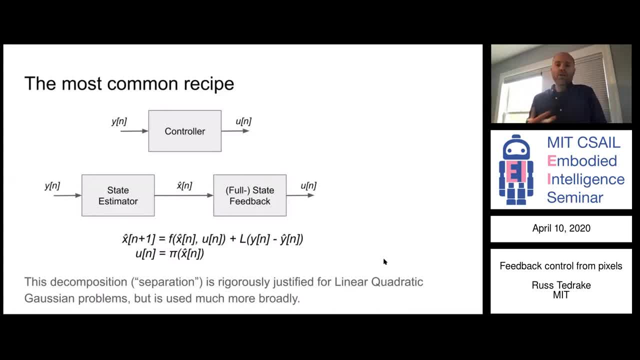 it all the time right, And I would argue that it's almost. it's so compelling and, like in our work on on legged robots, you know, I felt like often we had to stop relying on full state feedback that we weren't able to. you know that the fundamental problems in the in the task were: 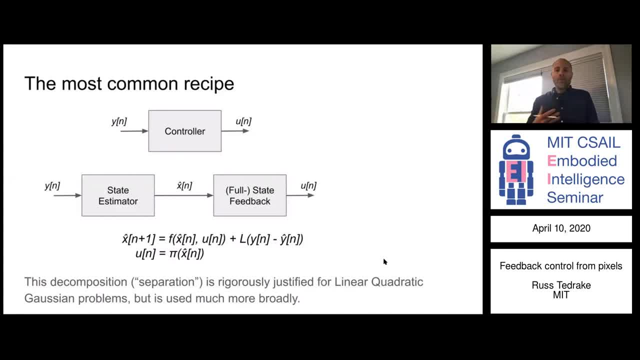 the fact that we were too heavily dependent on our state estimate. but it's just so tempting to build a better state estimator or spend a little bit more money on your IMU or or whatever, and to write these systems in this form where you're writing a state estimate. it is some recursive. 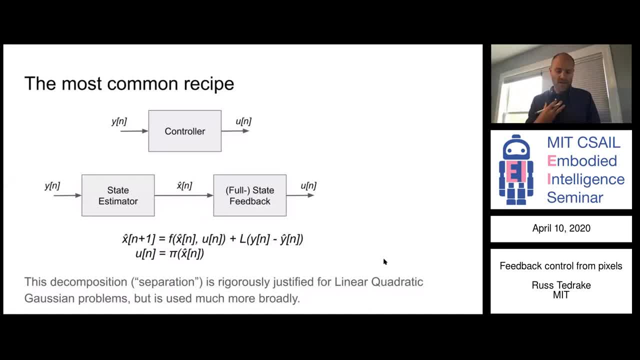 filter of a form like this, and in the case of a linear quadratic Gaussian, it's the Kalman filter. gains are for L, okay, And then I'm building a controller that's going to be able to do that. that's just as if I had perfect sensing I could. I could build a controller that knows the state X. 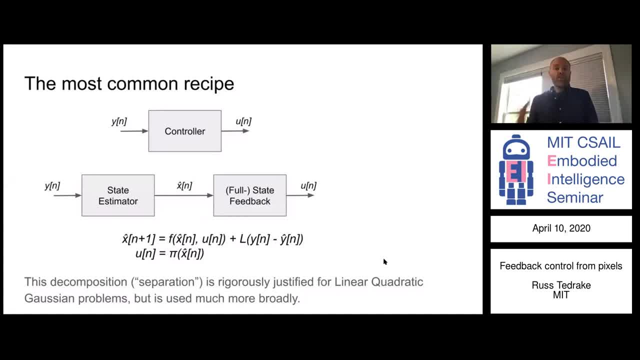 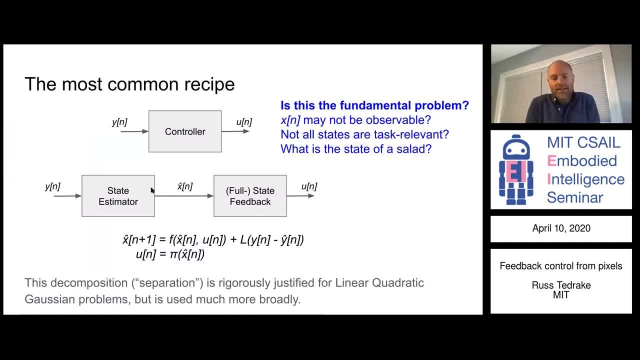 and makes those decisions All right. so is that it? Is that the? did it really not update? Okay, so is this? the fundamental problem Is the reason that we're not good. I- I assume people agree that we're not good at doing feedback control through cameras. we're- we're getting better at it, but 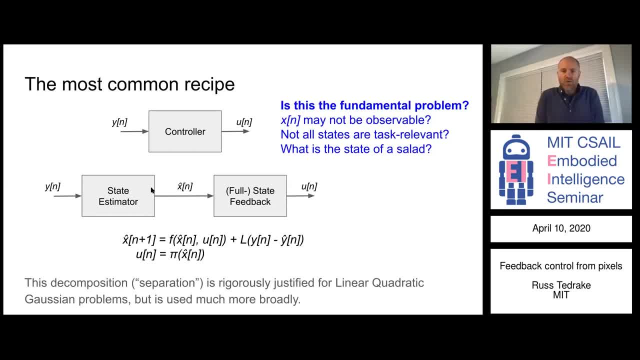 maybe the fundamental problem, the reason that we haven't done it with rigorous control, is that we shouldn't be doing the state estimation step that maybe you know X, N is often not observable in problems like this thing. that we were the visual motor. examples I. 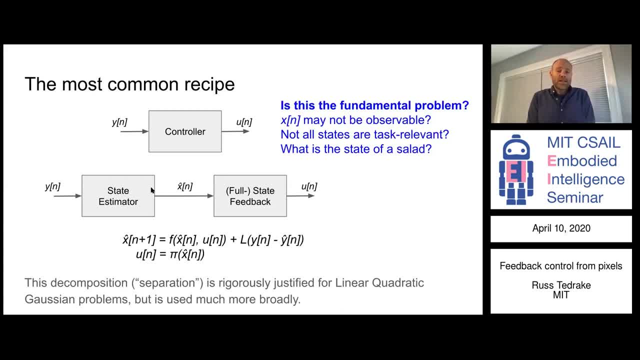 was showing in the first few slides. maybe not all the states are even task relevant, so so observing it could be a false goal. having to having to try to come up with estimates of the entire state vector X right. There's a bunch of state in my image that's just not relevant, For instance like 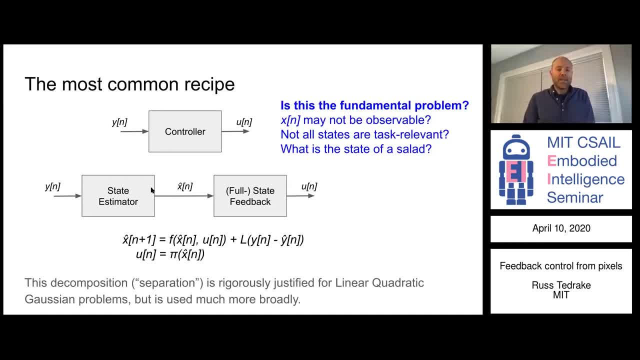 what is the state? if I'm trying to, if I'm trying to program a robot to to make a salad, you know what's the state of the salad. Or my other favorite example here is: you know? let's say: I'm, I'm. 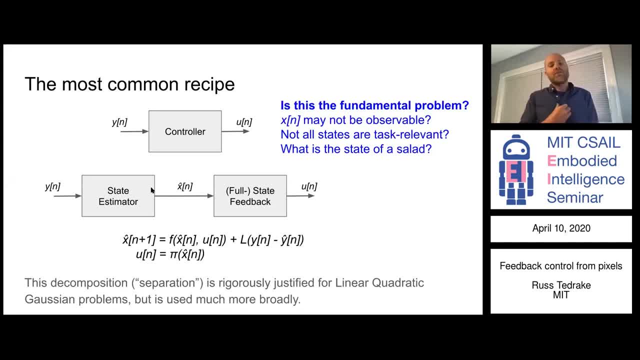 I'm going to button my shirt. I'm going to build a controller that should button my shirt, or button all shirts, right, If state one. step one is to estimate the full state of my shirt. you know, it feels like probably we've gone down a rabbit hole there, So maybe that's the fundamental problem. 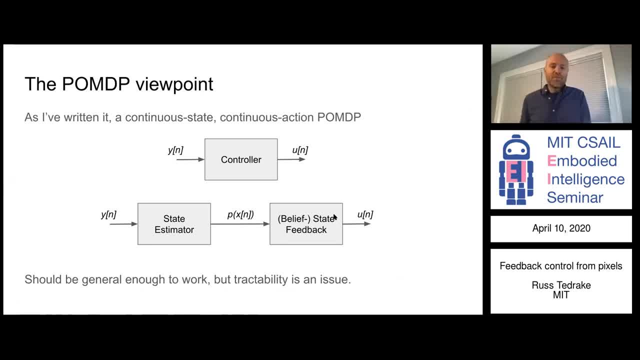 Okay. so of course many people on the call will say it's, it's a POMDP. of course we shouldn't be estimating the state. there's a more general framework that can capture this And in fact, maybe in the full glory, we should be actually estimating an entire distribution over. 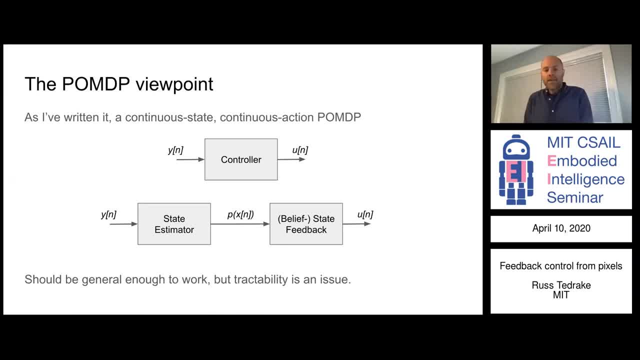 possible states and then be doing feedback that can understand that distribution right, Right. this should be general enough to work, I agree. In fact, I think this has led to lots of insights about what the optimal controllers could be in these more complicated setting. 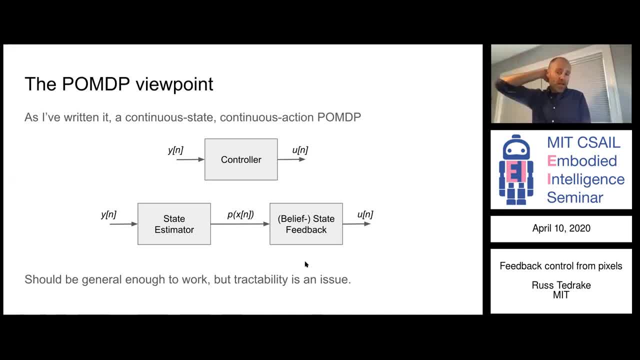 but it's hard to get tractable results, especially in in the forms I'm writing here, and the problems we're talking about they're relatively high dimensional, continuous state, continuous action and POMDP, So that's maybe hard going. 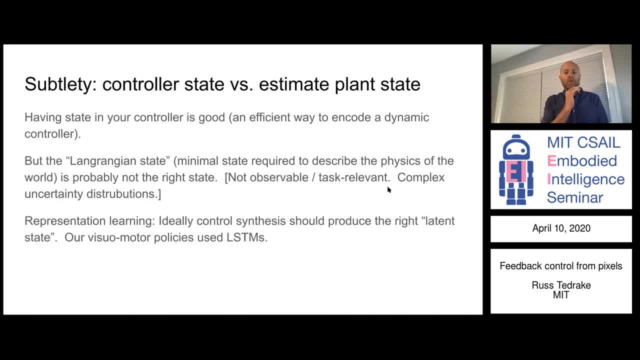 So there's a subtle difference I want to make. I want to make sure we're pointing out here which I think people know and talk about this in slightly different language, but let me use it in my language, right? So there's a difference between the controller state and the estimated. 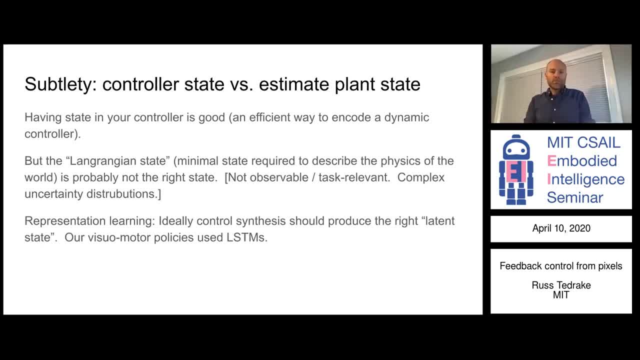 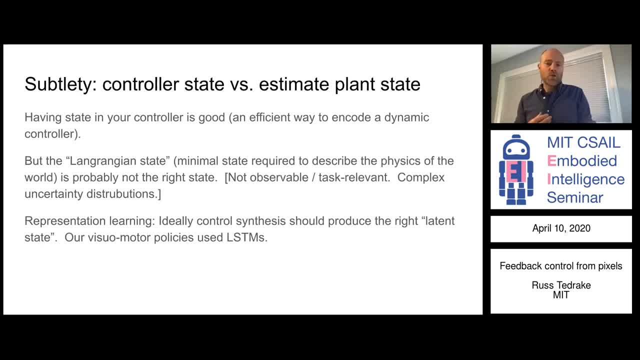 world as it would be parameterized in. for instance, to write the equations of motion for simulation right- I'll call that the Lagrangian state right- Is probably not the right state space for us to do to have in our controller If I'm trying to program a robot to to make pasta. 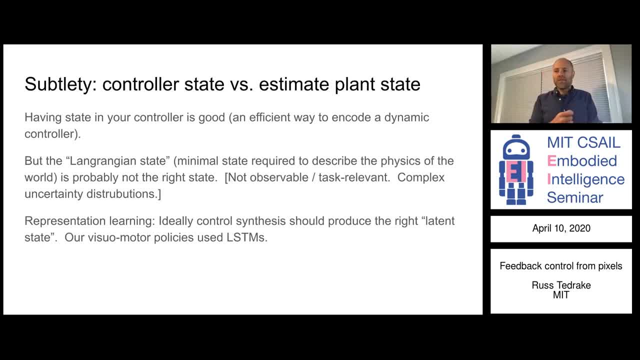 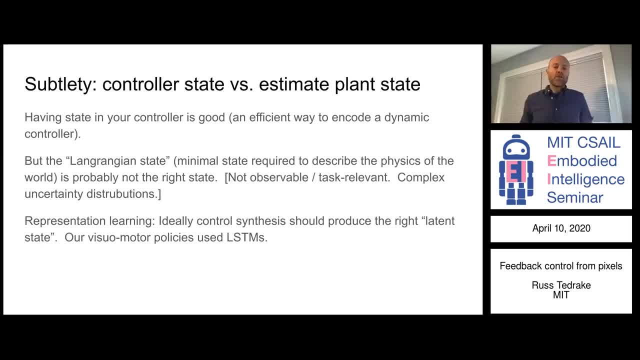 basically in the bowl or they're basically in the pot, right? So that's the question of state representation, learning and other things that we we talk a lot about. that Philip talked about when in the first EI seminar, I guess. Now here's maybe a more- you know- optimistic view. I think that 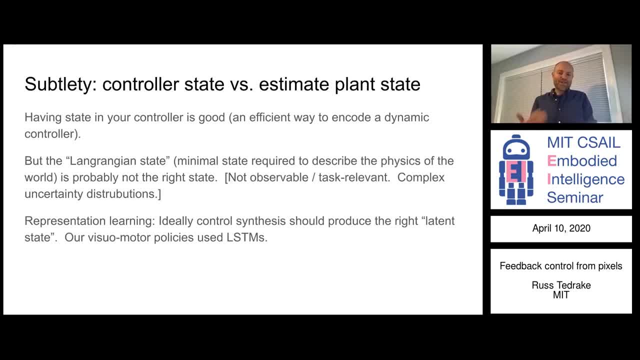 should just be a control problem, right So? so ideally, perception should just be the output of my controller synthesis. If I've got strong enough control synthesis, then the idea of what's the right latent state should be what I'm trying to do. So I think that's a good question. 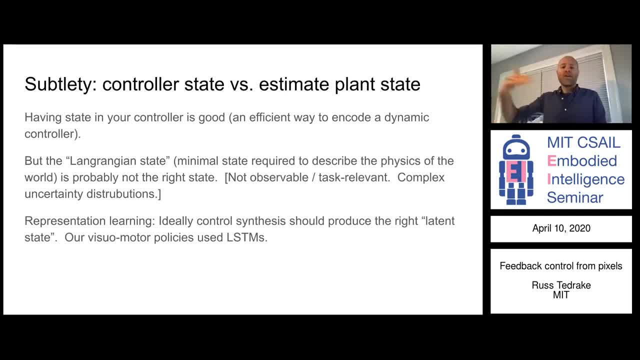 I think that's a good question. So I think that's a good question. So I think that's a good question. Whatever it's, whatever it's required to find this transition from Y all the way to U right. You know, we've- and we're doing this already a little bit in practice- Our visual motor policies. 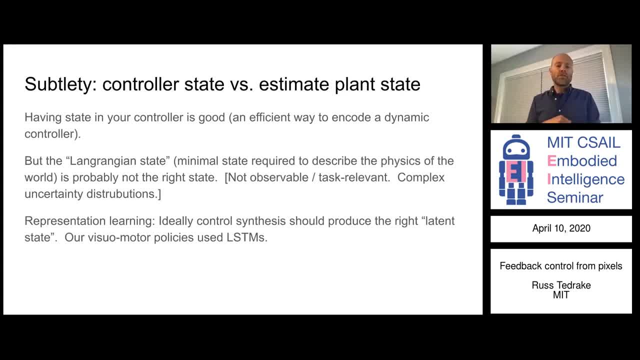 did have internal state. You know, we we trained via imitation learning, LSTM networks in order to do this. Pete and Lucas did, and they were encoding some internal state and you could sort of watch and try to guess what those states were meant. You know after the fact, like there's some, that 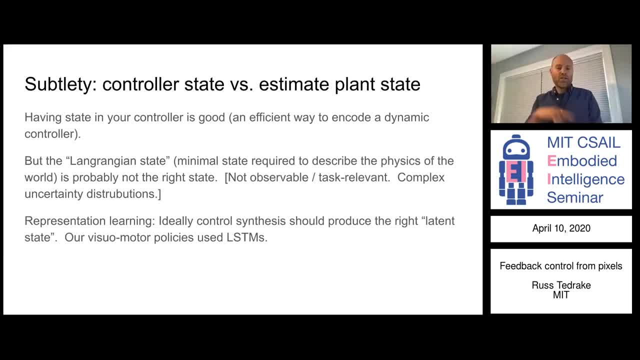 seem to be one, just seemed to be time, which was ridiculous, but you know another one that was indicating that you're in a different phase of emotions. they would sort of turn on and turn off. Okay, So having internal state in your controller is a good thing, I think, but expecting the 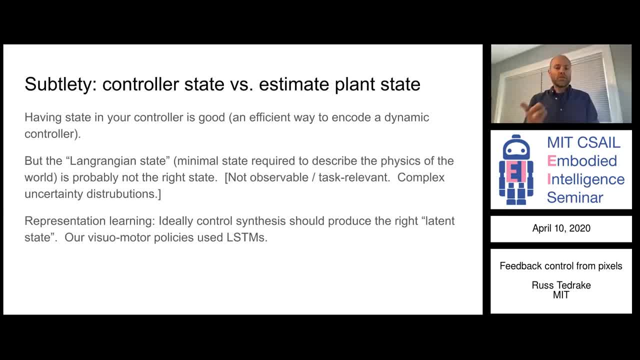 internal state of your controller to be the full state of the mechanics of the world is probably not a good goal And I think the you know the problems in computer of using you know that had come up. when you have the opportunity to do crazy things with a camera, maybe show those off. 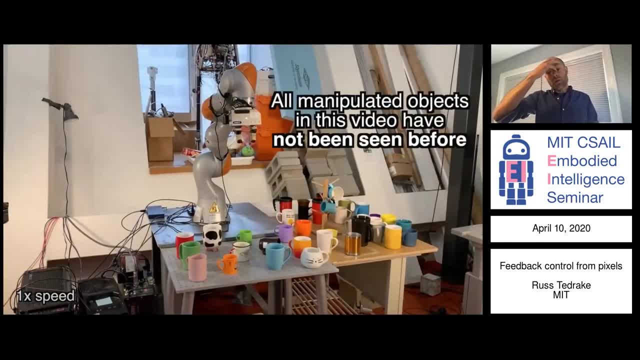 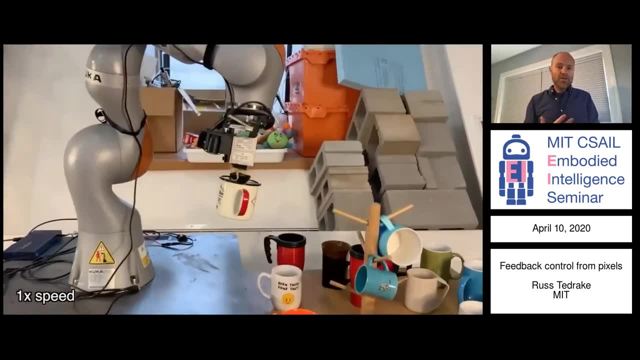 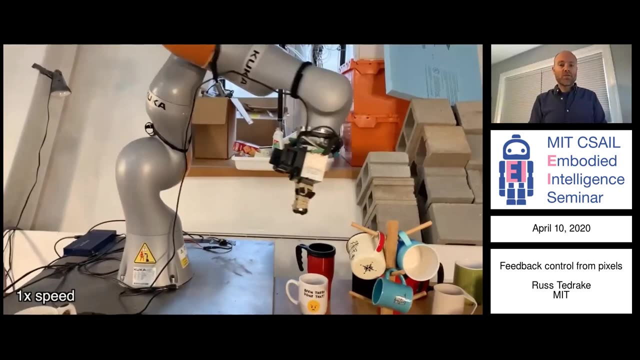 Okay. So we have done things which use you know, which try to do good control with less with you know, with less, just to show off that even hand designed or hand labeled and then trained in a deep network features can do non-trivial tasks over a variety of objects. So 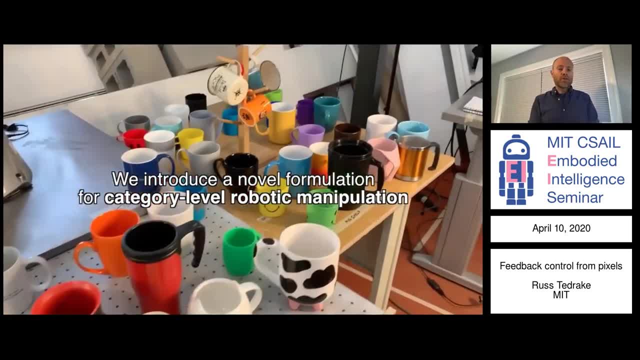 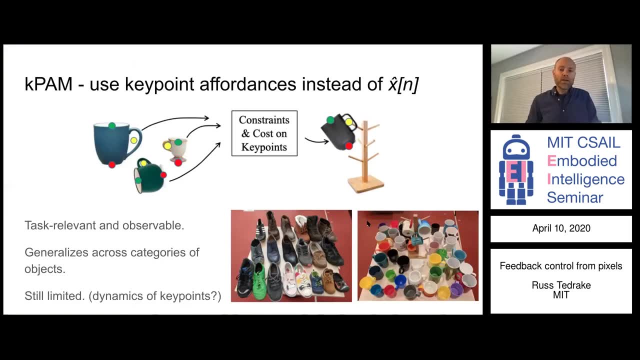 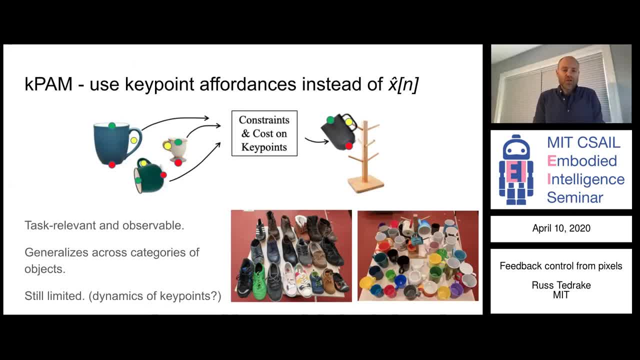 you don't need to know the full state of the world, You don't need to know the state of the shoe in order to program a lot of meaningful tasks. Or if you wanted to do something like put a mug on the rack, then actually just knowing a few key points right, And then it turns out key points are: 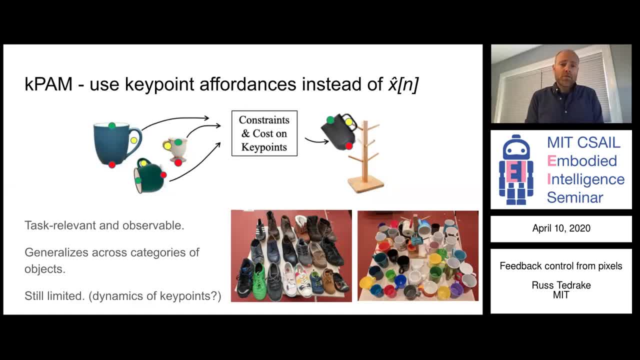 exactly the in the same way that people use in in perception right In computer vision training, a network to. to put out a few key points which are somehow the affordances of the task. They don't necessarily have to, they certainly don't have to completely specify the geometry of. 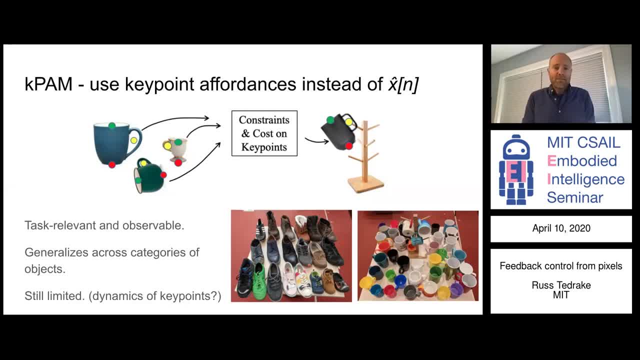 the problem. They don't necessarily say anything about the dynamics of the problem, but they're enough for me to say I'd like. the goal is to find key points in the current image, transform them through some rigid transformation, which I can do with an end effector command on my robot in order to make that. 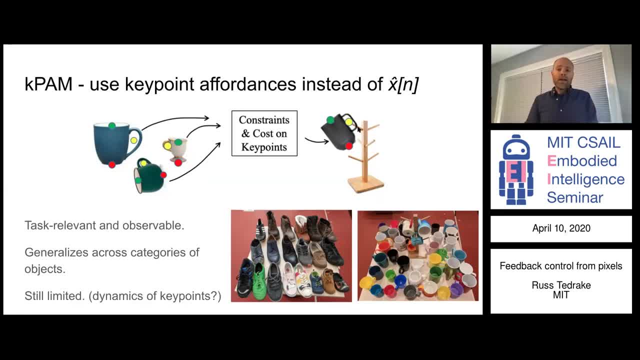 yellow key point end up on that, you know, on that rack, And that actually turns out to be one hand designed intermediate representation which is not the full Lagrangian state. And of course people have lots of other proposals for this about latent state variables and state representations. 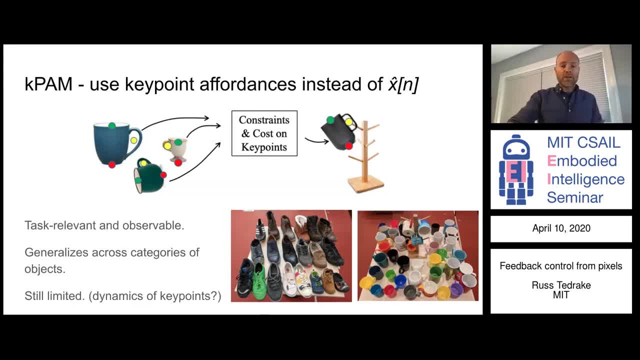 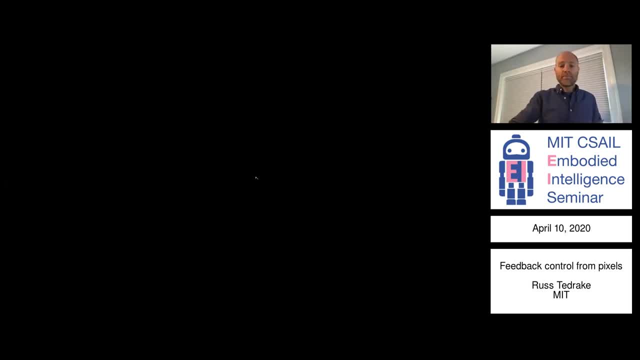 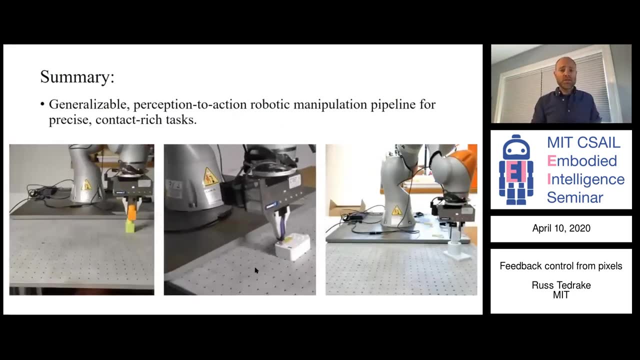 that could potentially work. Um, you know that particular work was still quite limited because we didn't have any model of the, the dynamics of the key point, how those would go forward. but way continues to surprise. Um, he can make now, uh, just with the key point based affordances thinking about end of you know. 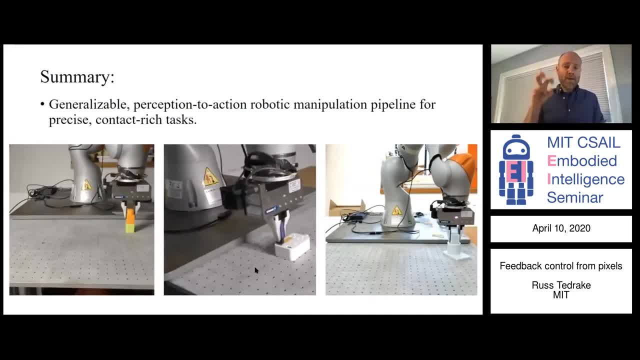 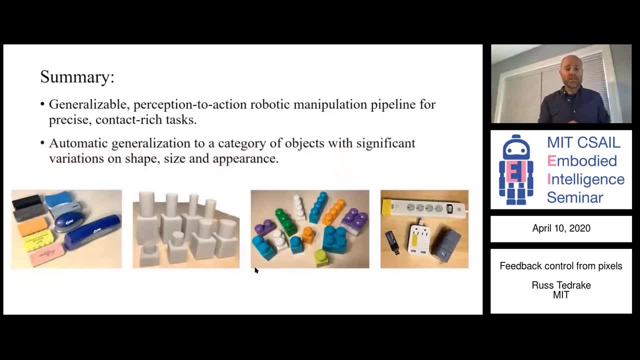 forces at the key points. he's actually able to make K-PAM uh, do pretty dynamic tasks with contact, rich assembly of of Legos and plugs and erasers and everything like this. So, um, you know, there's no, there's no really anything that can make it work the way that he can do So for the places. 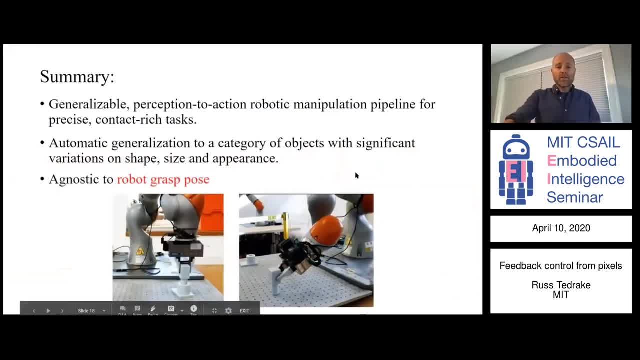 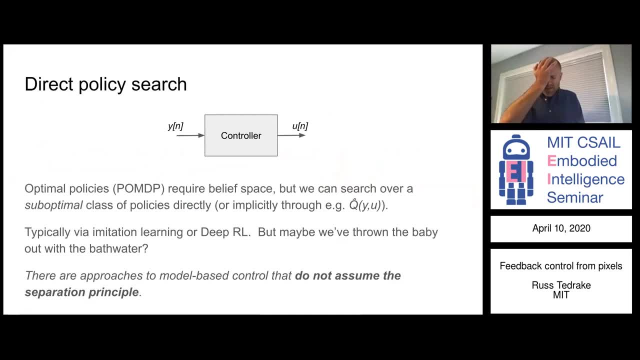 where the dynamics are relatively easy or they can be rigidly attached to a, to a hand. you can actually do a surprising amount of- uh, cool things with that. Okay, So, um. So state estimation is bad. you know, full state estimation is bad. Belief space planning seems hard. Um so people are sort of 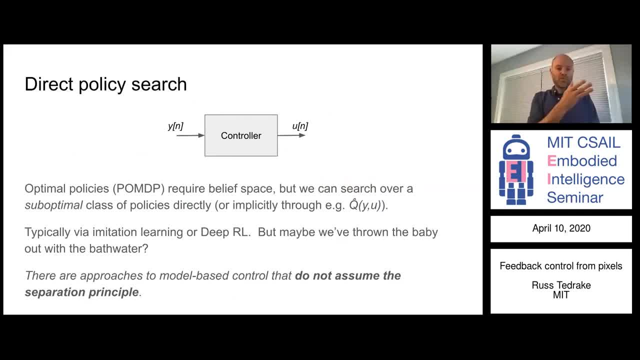 saying, well, let's do less, or, you know, maybe I'll just take the direct approach, right, I'm going to just learn a map from Y to U, right, And so maybe an alternative that avoids the complexity of naming a state. 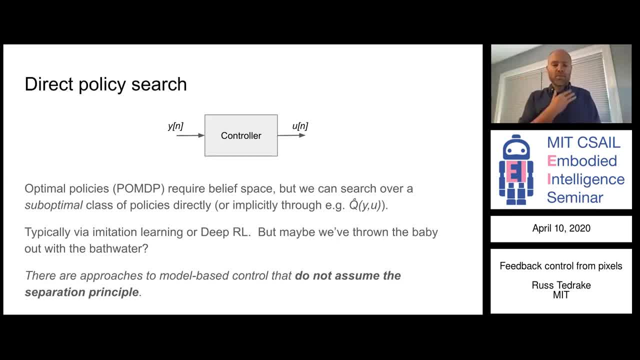 space. it avoids the complexity about reasoning over a complete belief distribution. I think the right way to think about it for today is that we're going to search over a suboptimal class of policies. The optimal policies for most of these problems are full belief space plans. 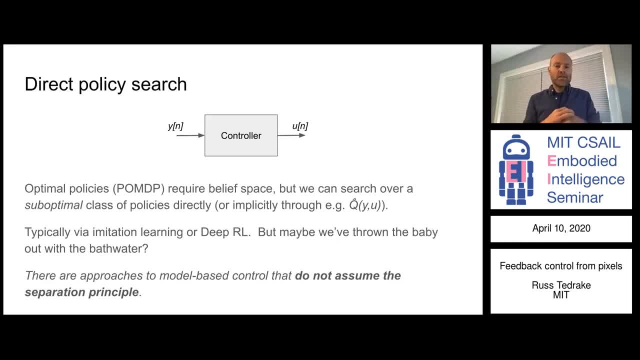 okay, But if I write down a simpler class of policies and can search over them directly, then maybe that's a way to get around this right. And we've seen a lot of success, including the first slides, a lot of good work out in the world of deep RL and imitation learning. 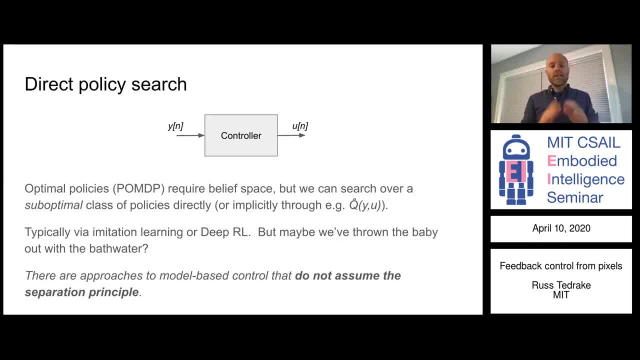 But I want to stop for a second and say: so that's a good idea. I think that's an interesting idea to do policy search directly. But all too quickly people say, okay, we're going to do policy search, And then they say: the only way we can do this is by either imitation learning or 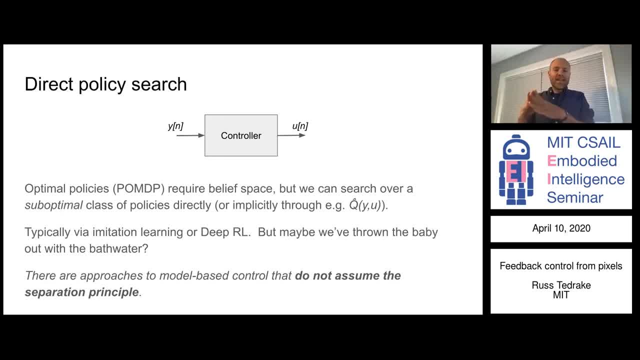 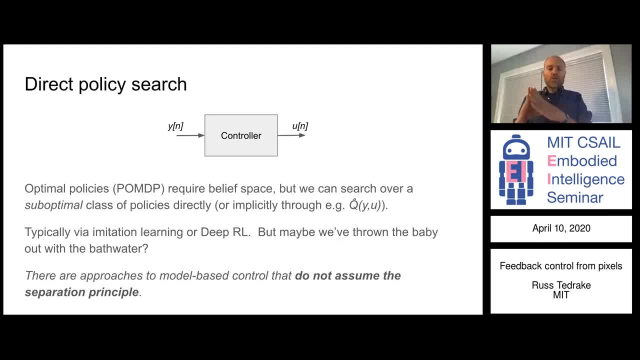 I agree that an interesting formulation is to just search over a simpler restricted class of policies, even if that restriction is a deep neural network, okay. But that doesn't mean you have to give up on the fact that you might know the equations of motion, You might know the renderer. 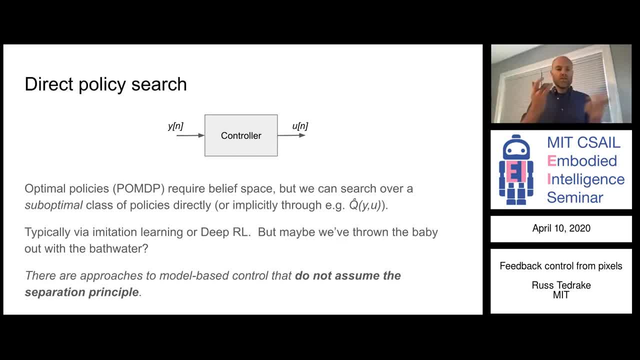 for instance, You might be able to do lots more things than we would traditionally do with black box optimization, And there are approaches to model-based control that do not assume the separation principle. Okay, so if you take away one thing, maybe two things- This will be the first of two- 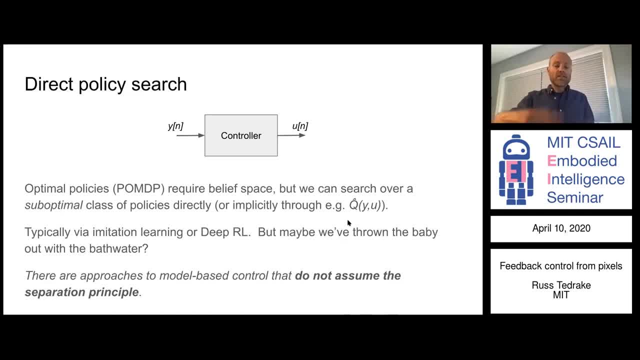 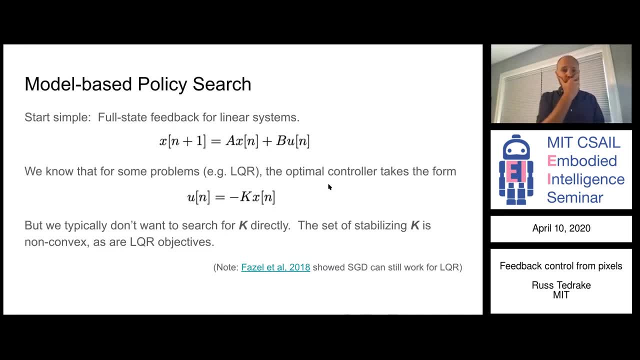 things I really want you to take away from the talk is that there are ideas of doing joint, you know, integrated perception and control from control, and we should be trying these, okay. So what does it mean to do? model-based policy search? Okay. so a warm-up example here is: 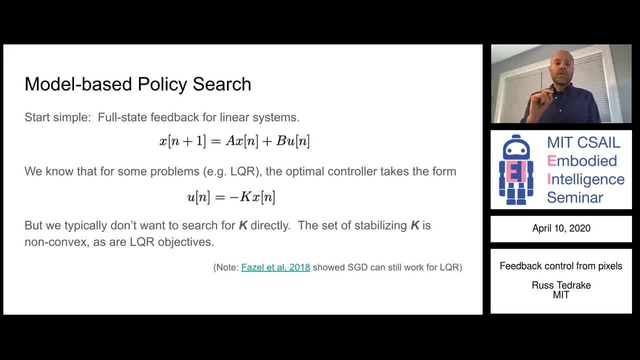 if I have a linear system and I want to do linear feedback control, okay. for instance, when we're writing a problem like a linear quadratic regulator, the optimal controller we know takes this form: u equals negative kx. okay, But we typically don't. 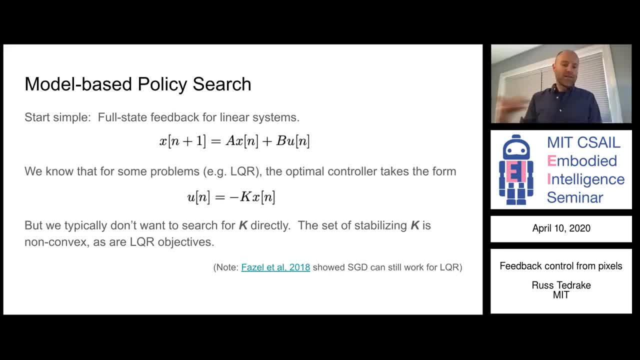 get k by policy search. right, We get it by calling LQR in MATLAB, which is solving a Riccati equation, an algebraic Riccati equation. It's indirectly, it's computing the cost to go, and then it's. 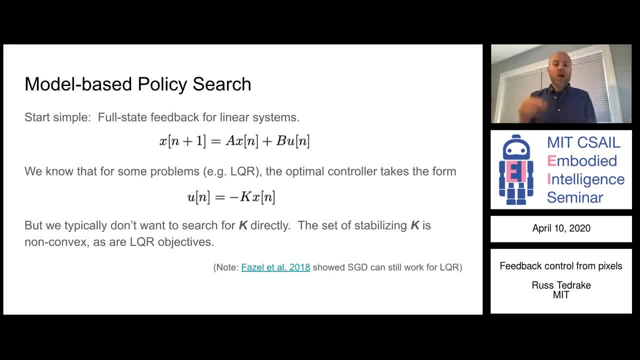 computing k from that And in fact we sort of know that the set of stabilized that k is a you know as parameterized like this is a bad set to search over. okay, In the sense that, regardless of your objective, I haven't even named an objective. this is, of course, related to LQR. 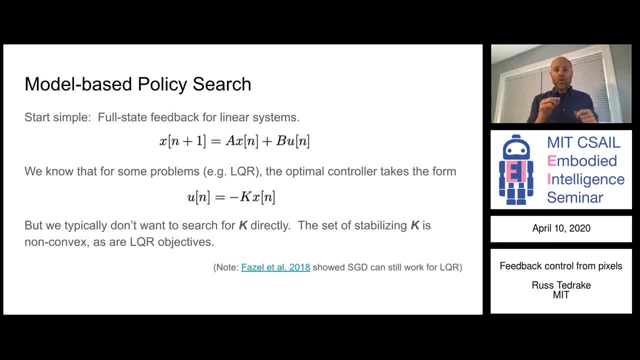 but even if you just look at the set of k, which stabilizes this system right, then that is actually a non-convex set. So almost any objective you put on top of that, you're going to have a non-convex optimization. Now there's some cool work that just you know fairly recent by 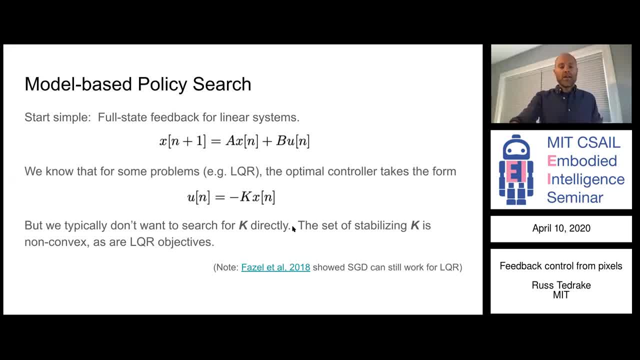 L. you know that showed, for instance, that you can still find with direct gradient descent on the parameters k the optimal policy in many cases with probability one. but I don't think that holds in a more general. I mean we're not sure how far that holds. That was a recent result. 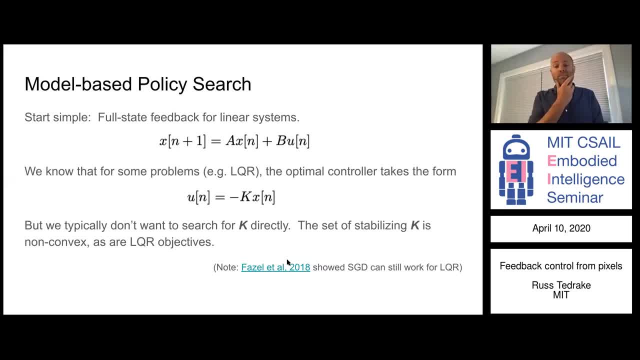 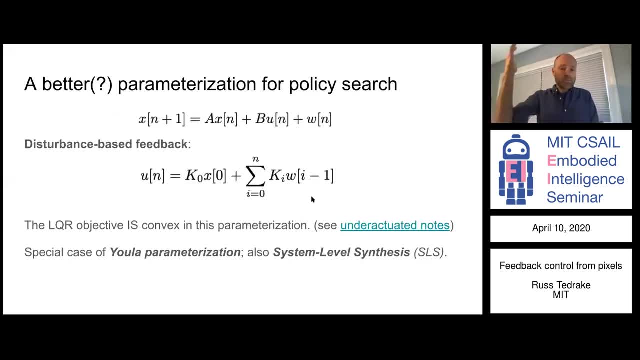 of an old idea. so I think we have reason to be a little suspicious of this, of searching directly in k. And we don't have to search directly in k because we actually know better parameterizations and control has known these for a long time. okay, So if you have a system that is, I've added in disturbances here. 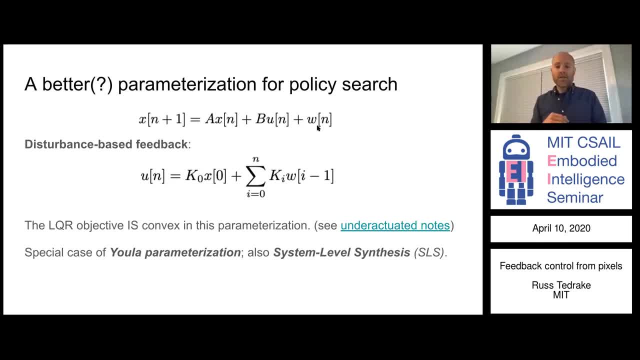 because that's going to be useful in our parameterization, but basically the same system that we had before. instead of writing u equals negative k, un equals negative k, xn, I'm going to prefer to write it actually as disturbance-based feedback, So I'll do a k based on the initial. 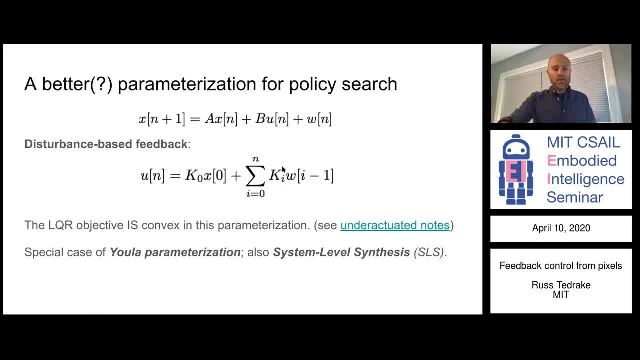 condition x, but otherwise I'm going to just multiply- look for k matrices that are multiplied by this- and then I'm going to add in an additive input w, And the idea is, if you think about it, that the nominal you know from any one initial x0, I could actually have the rolled out solution if there. 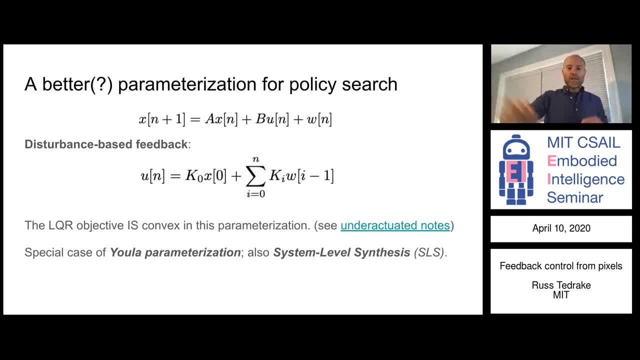 was really no disturbances that I could encode what u should be for the rest of time just in this k matrix. right, It's a time-varying k matrix that goes out, but I could just basically have my entire solution into this one k matrix. The only way that that has to change is by responding to. 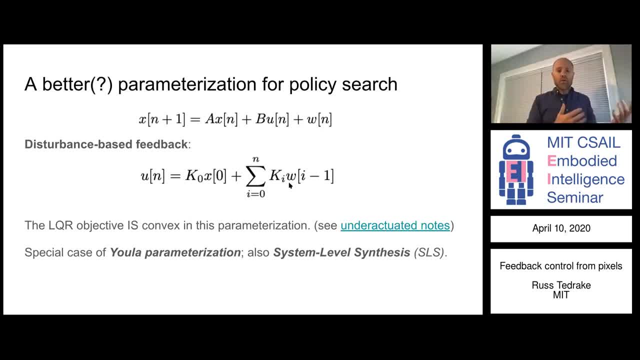 these disturbances. So this is a complete parameterization. it can perfectly, you know, recover the original parameterization, but the big difference here is, while multiplying by xn puts a recursion back in and you get k times k times k times k for anything like this. 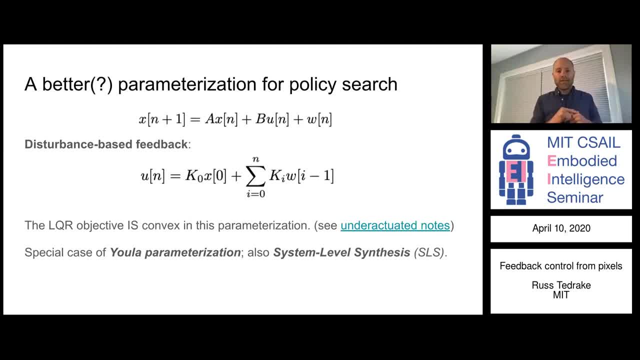 and makes it non-convex. this is additive in k and the most of the objectives we like you know- L1 objectives, LQR objectives, all the things they are- they are convex in this parameterization. okay, This is. you know, it's a special case of the Euler parameterization. it's also an 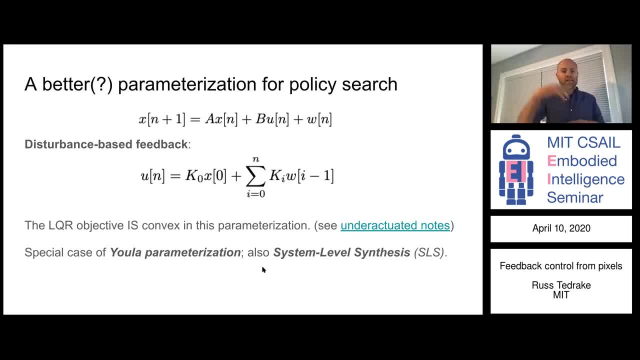 unknown as system. it's also used in system-level synthesis, which adds an additional. system-level synthesis is kind of like the direct transcription versus shooting approach to this. if, for those of you that have heard, you know taken under actuated, for instance, okay it's, they're very related. 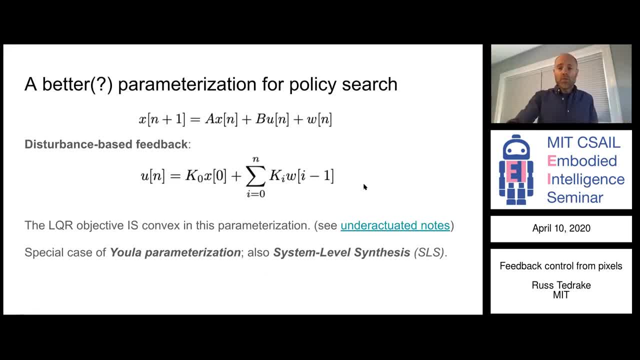 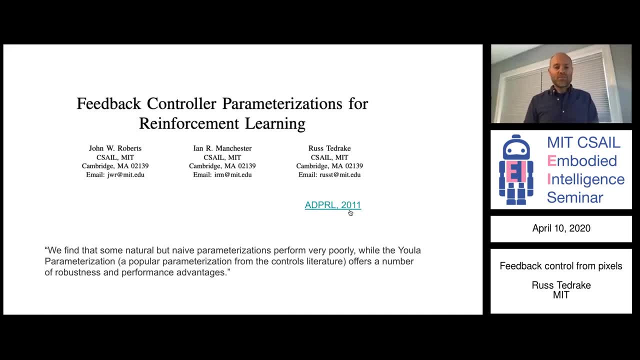 Okay, so there's a better parameterization and actually, you know, we should probably be using that in reinforcement learning too. I feel like we've known this for a while. maybe this was, this was April 2011, and it was maybe after it was. 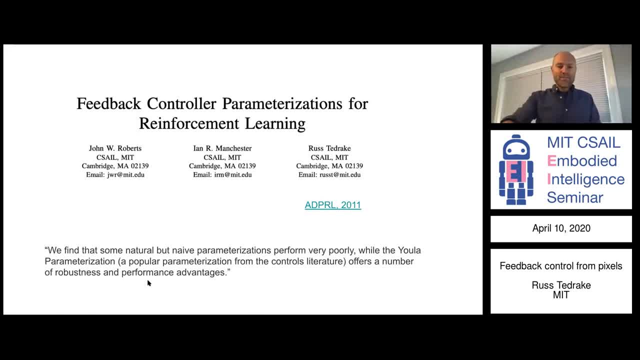 it was cool and before it was cool, so poorly timed. but but you know, we thought we, we showed that. you know, Euler parameters are just obviously a better parameterization for, for reinforcement, learning tools too, and I think they, I, we did mostly the linear case in that paper too. 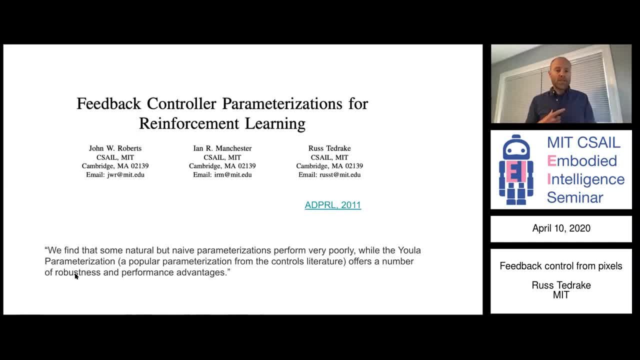 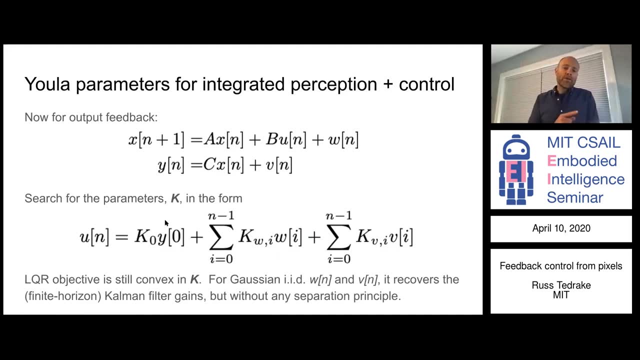 but actually the Euler parameters are a nice choice for even non-linear plants, and I I think there's just some core lessons from controls that we should be using in RL. okay, It turns out for the purposes here. it turns out that the Euler parameters also allow you to. 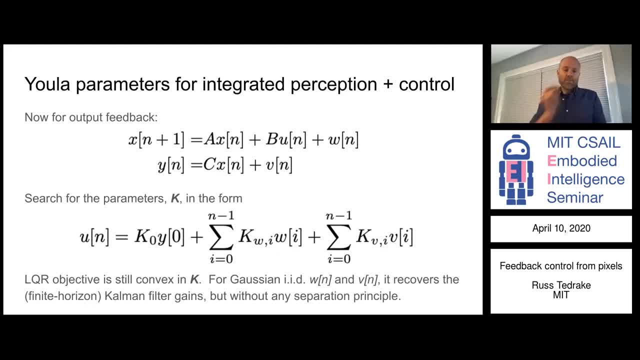 formulate a policy search that does integrated perception and control. and I- I'm almost embarrassed to say this because I I feel like it's been hiding in plain sight and- and I did, we should have been working on this for years, but, but, but here we go. So, so for the output. 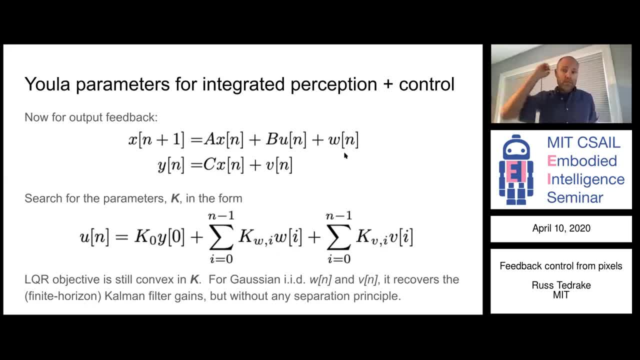 feedback case here, and let's think about it for the linear systems to begin with. okay, if you write down this same sort of disturbance-based and then you write down this same sort of disturbance-based feedback, which is this? now it's got you. you have feedback both on your disturbances and your. 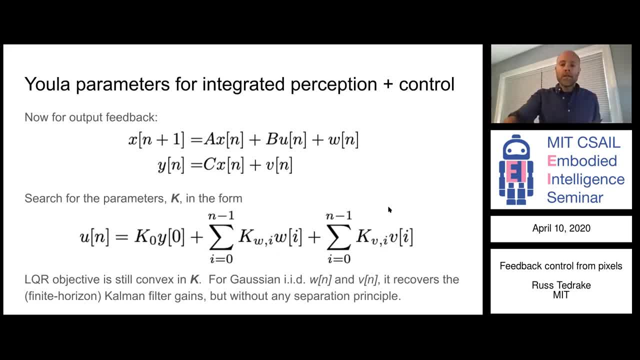 noise here okay, which you can measure after the fact. it's always using, it's always causal on those variables. then actually the objectives, like the LQR objective, are still convex in K. okay, and the cool thing is that this is a. these are finite horizon formulations typically. 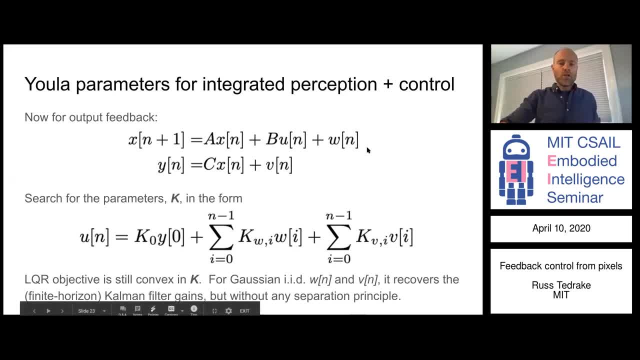 but for if, if you put in you know that the? the Ws come in as a guideline, and then you put in you know the? the Ws come in as a guideline, and then you put in a Gaussian IID and V comes in Gaussian IID, then actually, even though this is jointly, 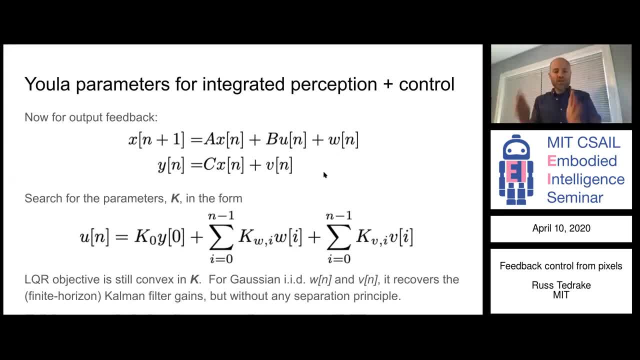 designing the filter gains and the control gains. it's actually recovering the Kalman filter, okay so, but it's applicable in cases where I mean where W might not be Gaussian IID. you can, you can write more rich specifications. Sajra in our group has been 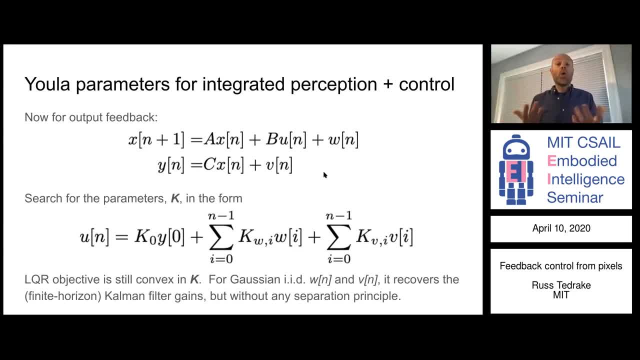 thinking, thinking about lots of different ways that you can leverage that fact and do more with sort of these sort of parameterizations. Okay, so that's observation. one is that there's a lesson to learn from control, I think, which is that there are better parameterizations. 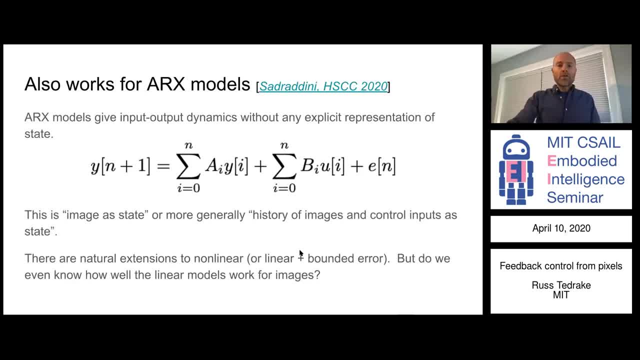 if you're going to do policy search, Okay, Sajra in particular has been pointing out, you know, because the equations I wrote just now still declared that we need to effectively, you know, declare a state right. And I said I don't know what the state of my salad? 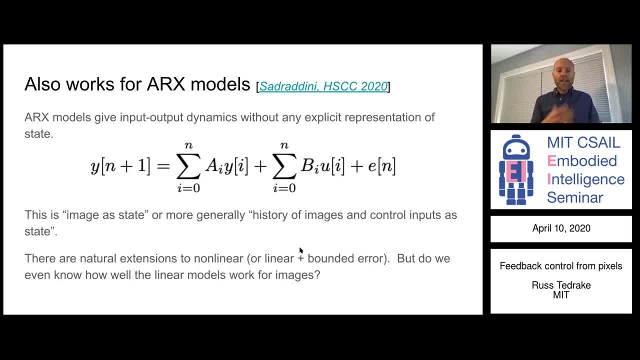 or my shirt is so I don't want to do that. The same kind of disturbance-based feedback parameterizations can also work for ARX models, right? So ARX models- linear ARX models- would being of this form, where you're just predicting your next Y. 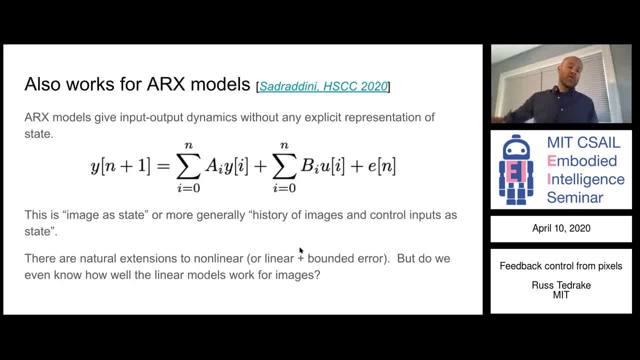 as some combination of your previous Ys and some of your previous Us, plus some error terms, typically called error now instead of noise or disturbances, but it plays the same role. okay, And when people say, okay, my image is my state in RL. 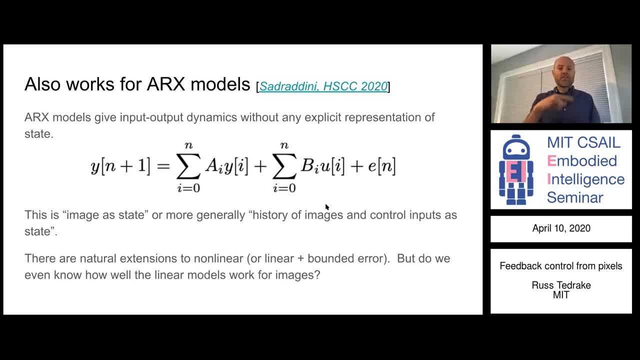 I think this is what I hear when they say, that is, that they're actually just doing a one-step ARX model and that's good and that makes sense, right And more generally, everybody knows we could do a history of images and control inputs as the state. 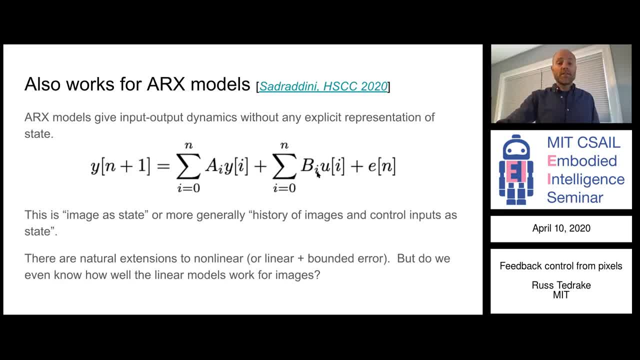 and I think that is justified. but it puts you into a slightly different class of models and I think we should be a little careful calling it state, because you can trip yourself up with that. Okay, there are natural extensions of this. Yeah, there's a question from Luca Carlone. 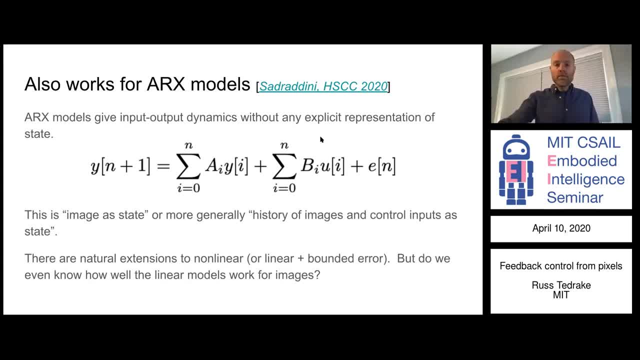 Okay, awesome, Luca. Can I mute myself? Just a quick question. If you go to the previous slide, you said that the noise terms are known a posteriori, but how do you get the noise in the previous one? Yeah, I'm navigating here. 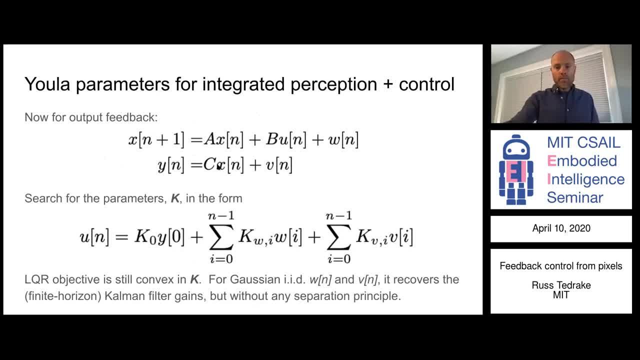 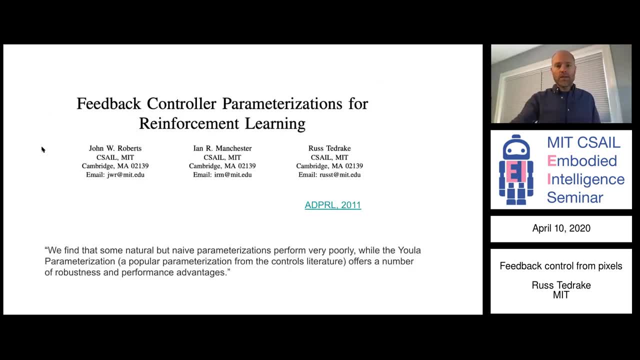 How do you get the noise? Because also a posteriori for retrieving the noise, essentially you need the state to be known, Right, right. So I thought about it more. Do you agree that it's easier in the state feedback case? 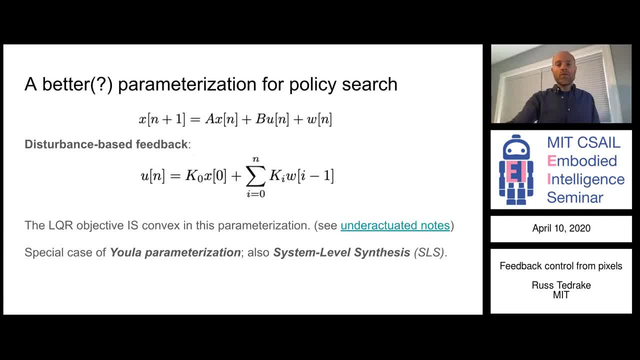 Yeah, if you have an estimate, you can estimate the noise as well. Yes, so afterwards, if you observe your next Xn, then you can just subtract it out in the past and figure out what W was the difference between my repeated measurements. 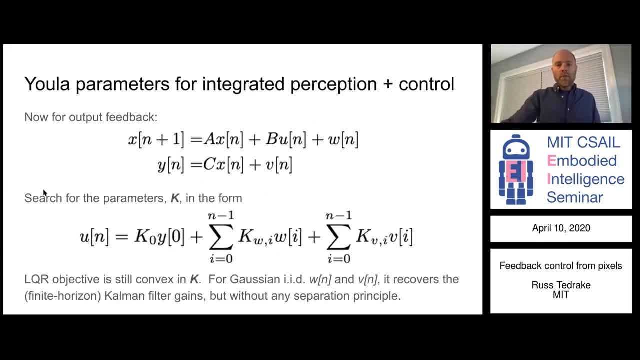 I believe that's all still true in the output case- that you can, after the fact, by using Ys at the next step, you can figure out what V must have been, and then again you can figure out what W must have been. 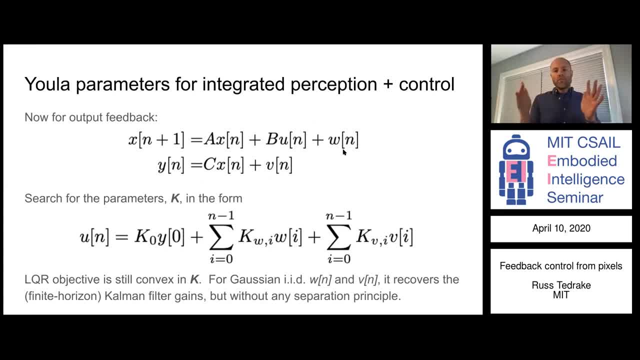 It's all done sort of after the fact. you see the error in your prediction and the error in your observations, But implicitly, I guess my comment is that you are figuring out the state as a byproduct of figuring out the noise. you're figuring out the state as well there. 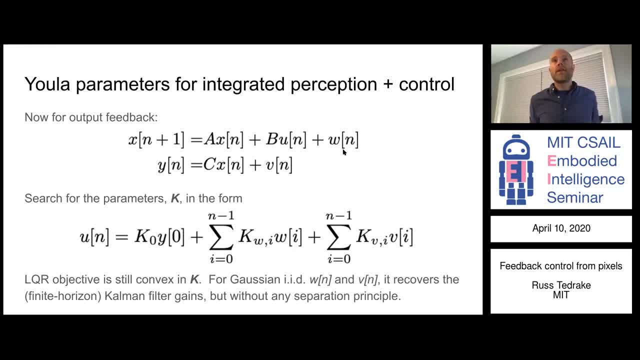 Ah, yes, so absolutely, They are able to do the same things, And this one in this particular slide. we still have to require a state space, which I think is a limitation, But the parameterization is better in this case. 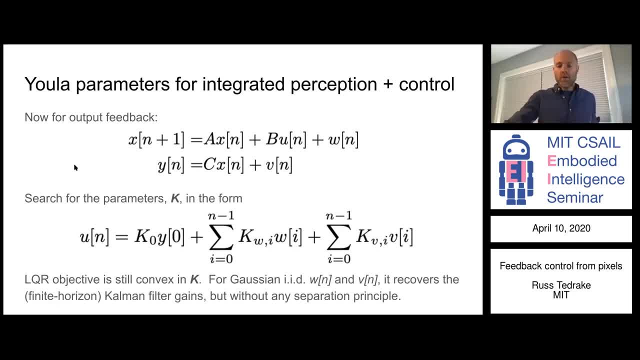 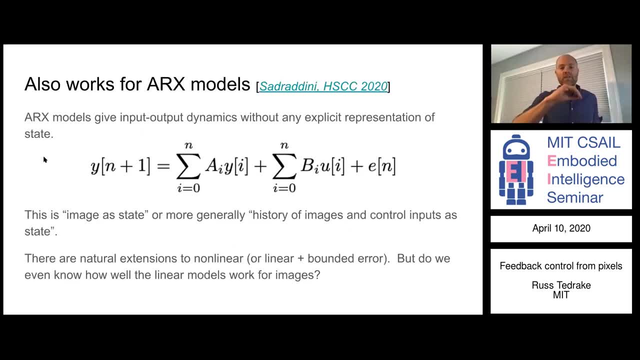 Okay, just wanted to make sure I was not missing anything. Thanks, Oh, I appreciate the question. Interaction is good. Okay, so, and this is the case where we don't need to declare a state and you can just measure in the succeeding measurements. 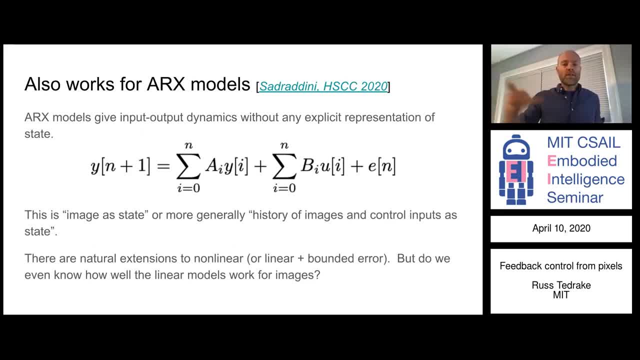 what E must have been based on what I've observed and what my prediction was, and I could figure out what E must have been. If I had had my model exactly, I would have gotten one Y. I measure a different Y. the difference is E. 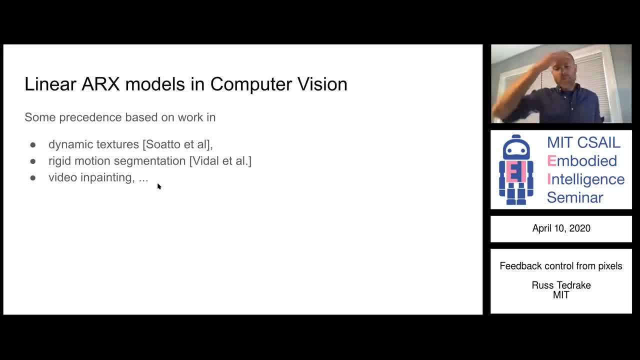 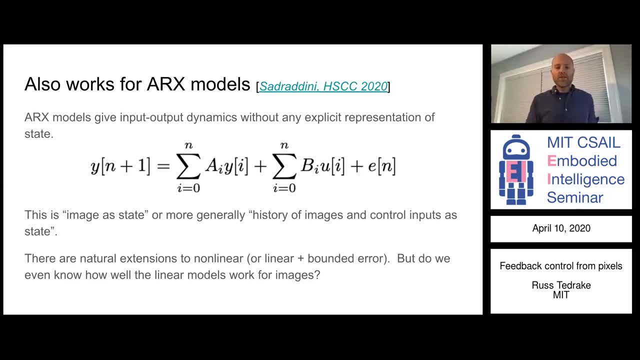 And you move from there. Okay, so. so I guess there are natural ways to apply it. I think the obvious question that should be in your head now is: like okay, this is a linear model. You start talking about cameras. 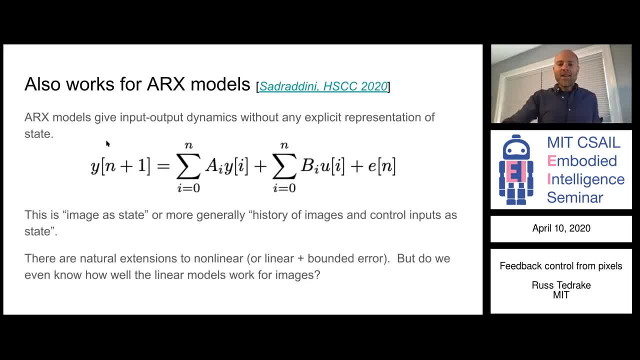 what the heck you know you can't do linear models for cameras, right? Well, it actually. I just want to check that Like step one. let's just make sure we can't do okay with linear models on cameras. 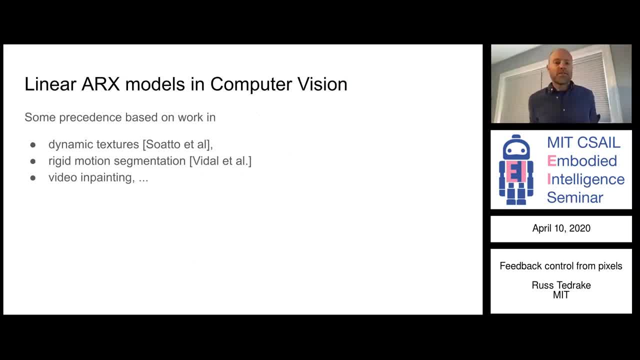 Okay, so there is some history of doing linear ARX models in computer vision, right. There's some precedence based on some work, some older work and dynamic textures and rigid motion segmentation video in painting. There's examples where people actually fit linear ARX models to. 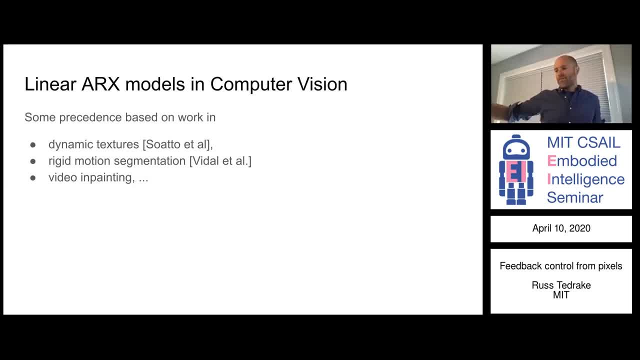 for instance, you know if they, if they want to put a- you know the waves on the ocean in the background, or something you can. there are cases where that has actually already worked. But let's get to a manipulation example here. 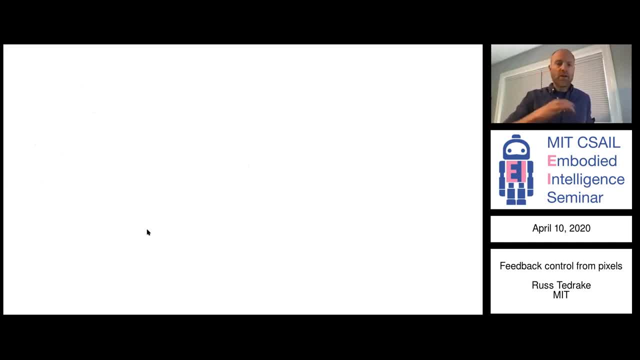 So Terry, who I don't know if he's on the call here, Terry, Sue joined the lab last year And and I was saying, you know, we're too dependent on stated feedback- we got to pick up, you know, a problem right off the bat. you know. 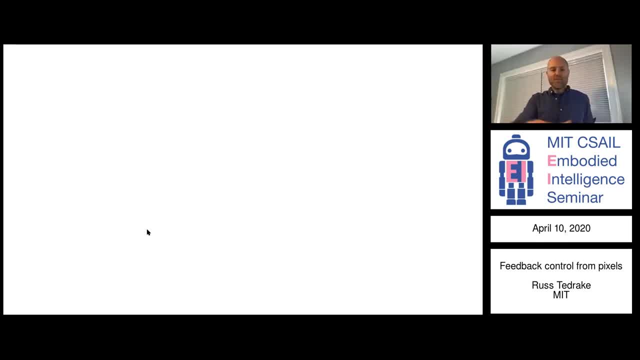 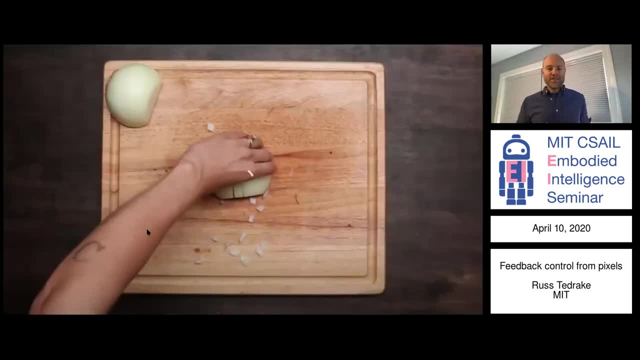 you're, you're, you're fresh, you're not corrupted. yet We're going to start with a new problem where state is not an option, Okay. And so we said, let's, let's think about chopping an onion, Okay. 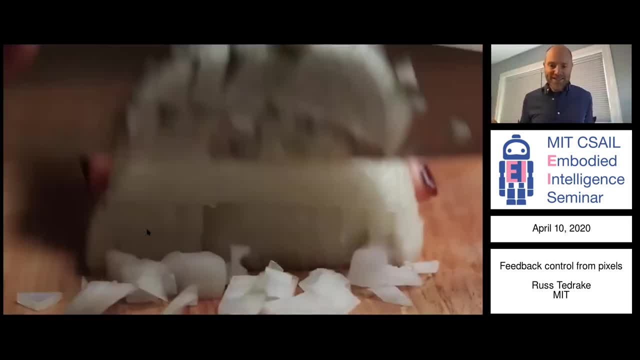 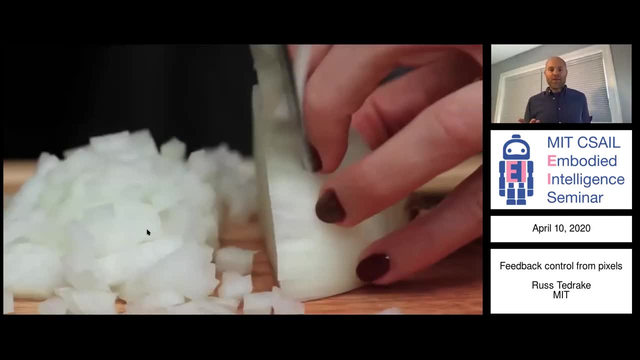 So what's the state space of the onion right And is it changing every time someone makes a cut? Is the number the dimension of my state, like my classical controls approach to this would be. I'm going to write a hybrid model. 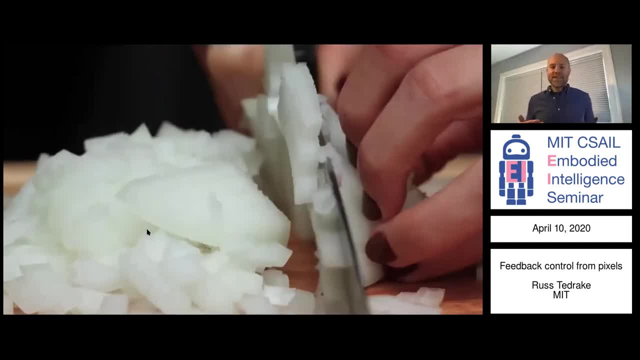 which, every time the knife comes down, it does a jump and a reset, And it does actually does like hundreds of them on every cut, And that means every controller has to be designed separately for every one of those cuts, even though, my God. 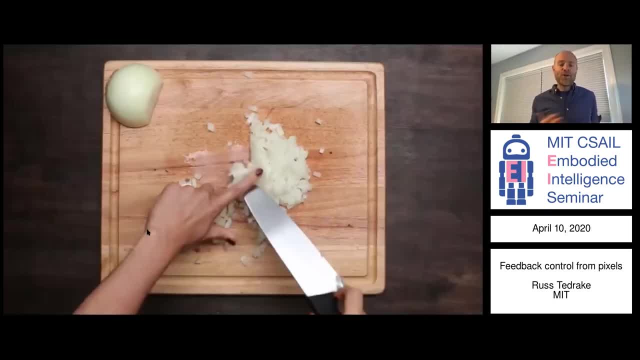 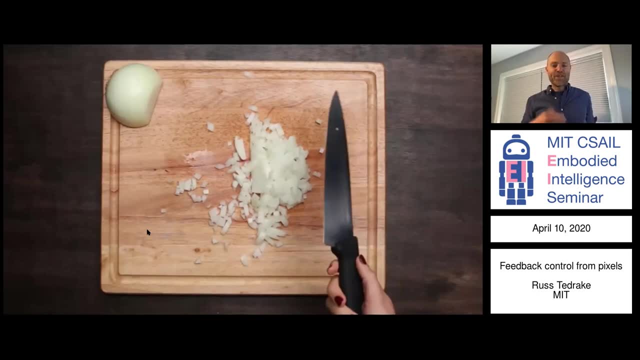 it's the third cut on. the fourth cut must be pretty much the same, right? So this seems like a place where there's no risk of us trying to estimate the full state of the of the Lagrangian state of the world. So we kind of 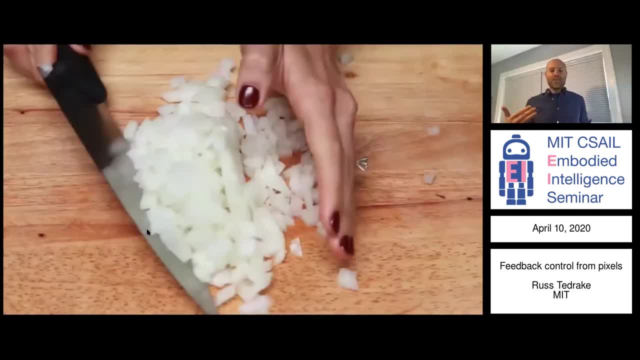 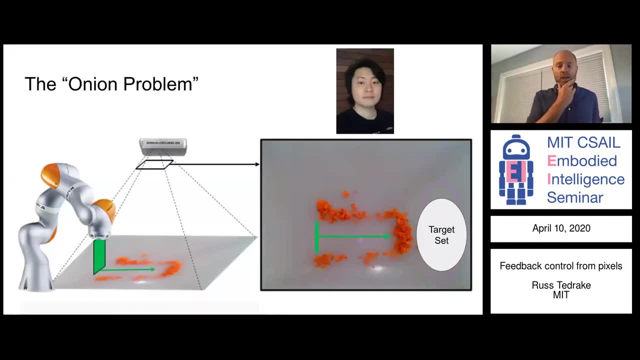 we're not going to get sucked into the state estimation, local minima. Let's try to do image based control on that, Okay, And then so we thought about how to actually turn that into a research problem. And well, so lesson one was that you shouldn't use onions. 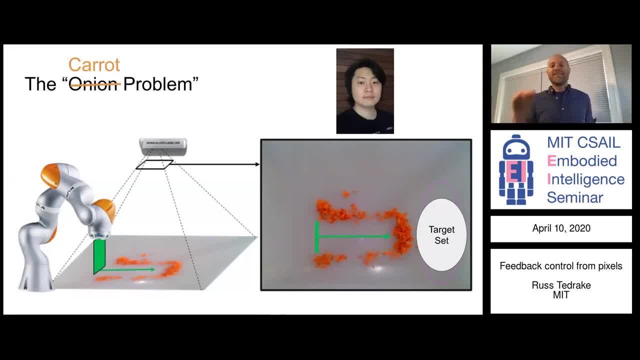 Carrots are way better because, I don't know, the lab smells better. You can see them better on a camera. They like last longer, So so I still like the. I still call it the onion problem. Probably I should update myself. 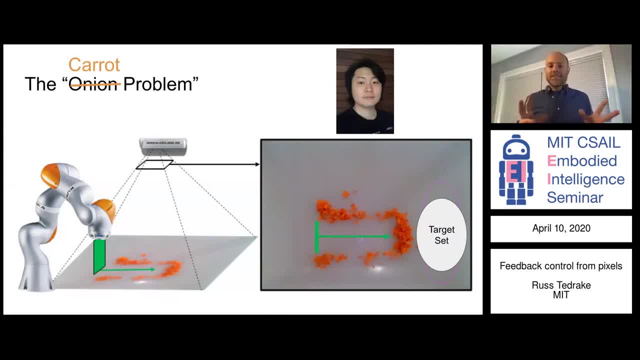 but, but I recommend carrots. Okay, Second step, second idea: probably you know, handing a deep network and a big, sharp knife to a robot. Maybe that's not where we start. Maybe we should start with, like, the second part of that. 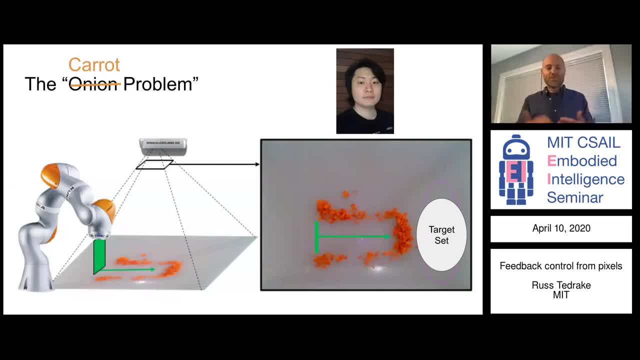 Where are the things have been chopped and we just want to move them around the cutting board. That's already pretty impressive. Let's do that part of it first. Okay, So, so now here's the setup. We've got a Kuka with a soft. 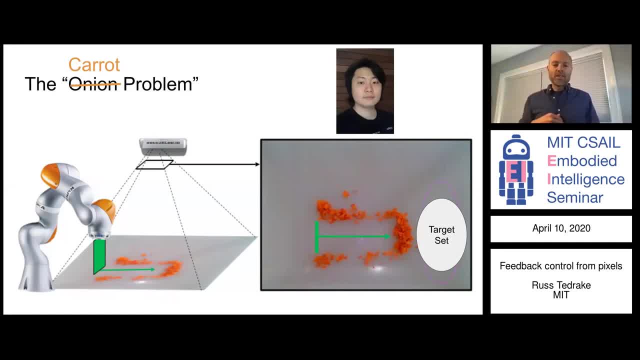 uh, you know um blade that can move around in the in the vertical axis, here with a camera looking down from above taking pictures of bright orange carrots, And the goal is to make it a more of a controls. problem is to 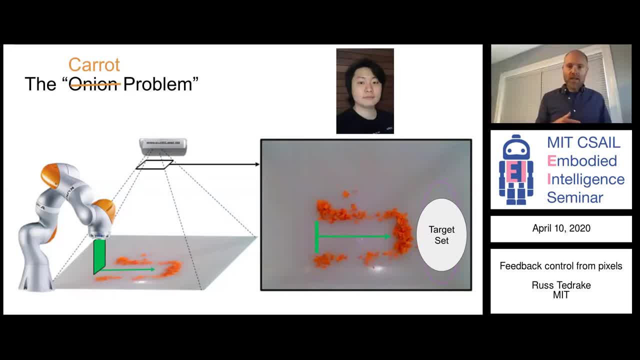 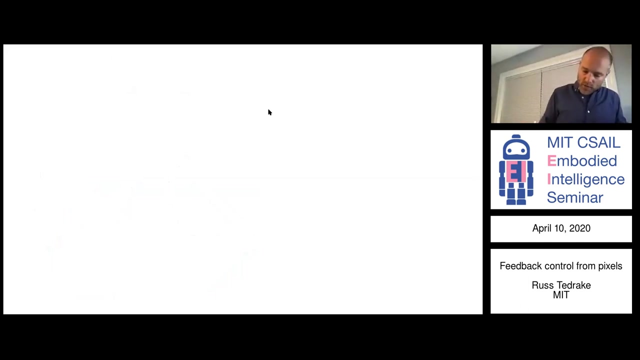 to drive those carrots into some target set. Now, my goal was to actually use the iPad here. let me just try one last experiment on that. Okay, So, um, the objective here. hopefully this is going to work. Objective is to 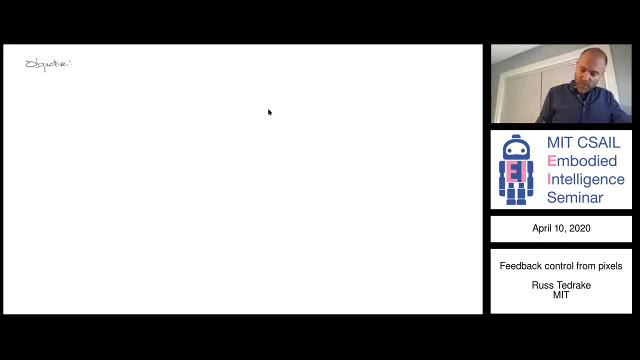 uh, uh, that's really poor writing, but okay, Um, you know, move all carrot pieces into a target set. Okay, I um observations, I, why, right, Why, And which is actually going to be. 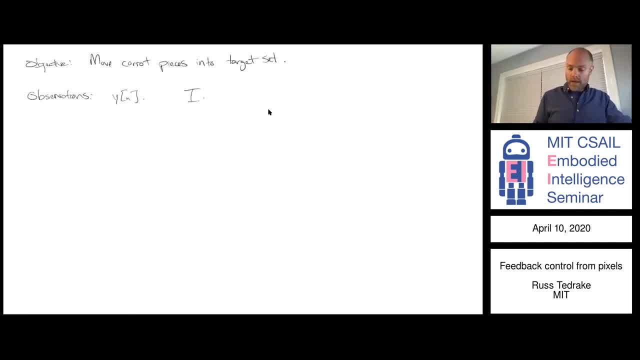 I'm going to use two notations. I'll use the image at time, N image. or sometimes we're actually going to write subscript K, Okay. And then we're also talking about the. why is the vectorized image right? So if I take that whole image and I squish it down into a vector- vectorized- 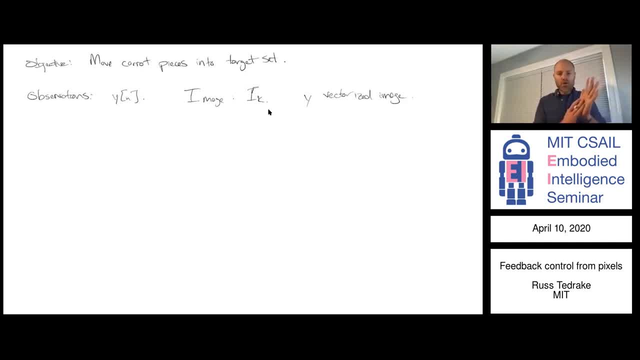 image. Okay, And that's it We're going to take. those are my observations, my control inputs. You then are going to be a push in the on the system, So I'm going to parameterize that in the same way that a lot of the good work on sort of pushing and 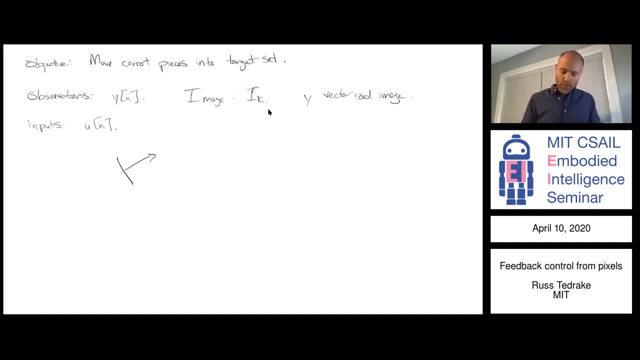 and the light had been have working in robotics. I'm going to just parameterize that with four numbers. This would be like the initial location of the pusher in the in the image and the final location of the pusher in the image. 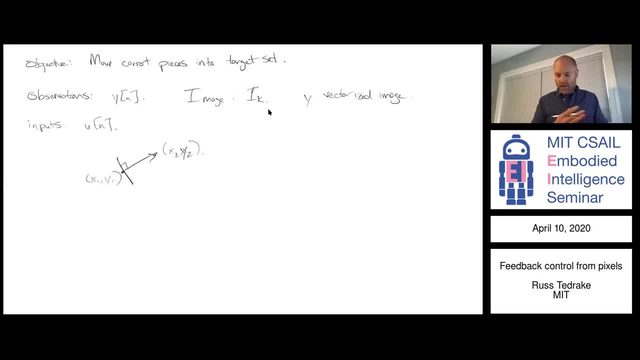 Okay, And I'm going to assume that that's just a constant size paddle and it's going to move along this And I'm going to write the dynamics of the system ultimately in the time of this push. So so, basically, I'm not going to model the dynamics of the push. 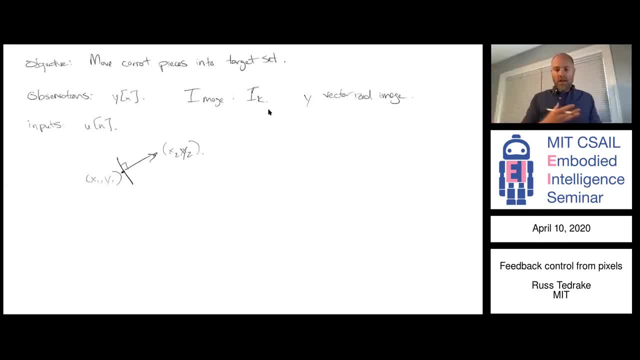 I'm going to say the a single action isn't, it is an entire push of a constant velocity. And I'm going to look at the, the, the image beforehand and the image after hand after, after the fact. Okay, Um, 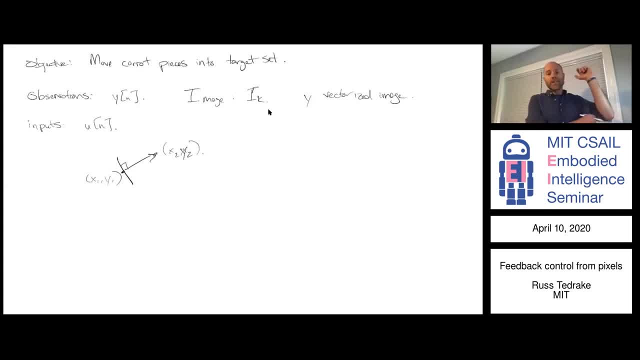 the way that we're going to write. you know, my goal is to somehow write a single controller, which is going to be um, you know you, and is some pie of YN. Now we could, in general, take the entire history of why. 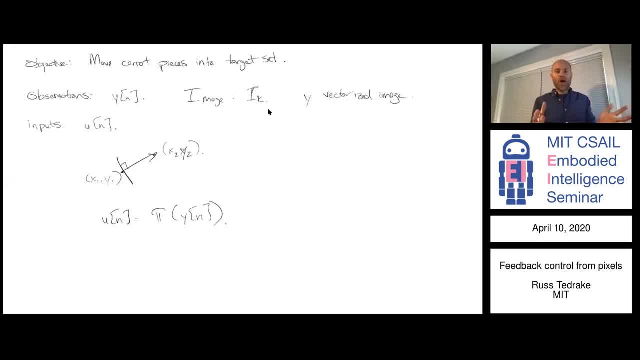 but I think for this problem there is not that. it's a quasi static problem. So the current image contains everything we need to know, And so I think it's it's reasonable to look under over this, And Terry thought it was most natural to think of this in terms of Lyapunov functions. 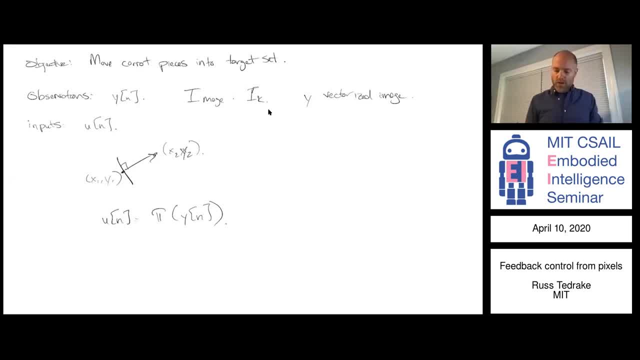 Okay, So we're actually going to write down a Lyapunov function which is somehow specifies my task. Okay, A Lyapunov function in this case? um, I could read it in a couple of different ways, but if I want to take some, 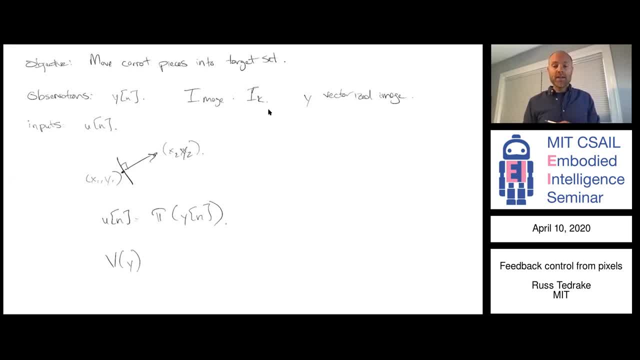 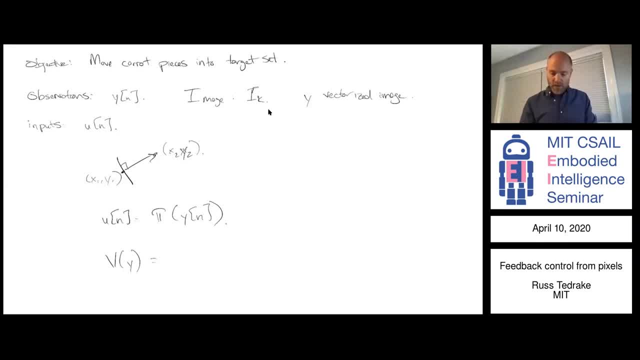 Okay, Okay, Okay, Okay. So it's going to be a sum of the distances between all of my nonzero pixels, which, which would be my, why I, an indicator sort of function of why I and my target set, which I wouldn't typically write S. 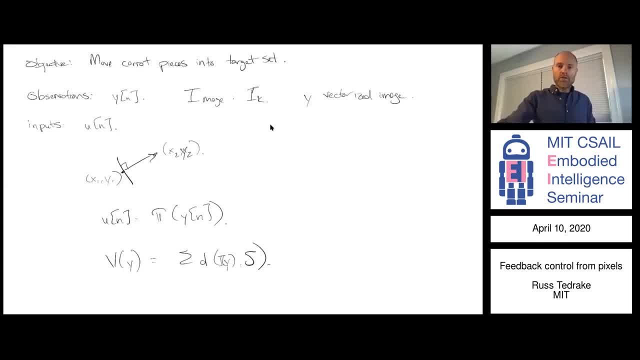 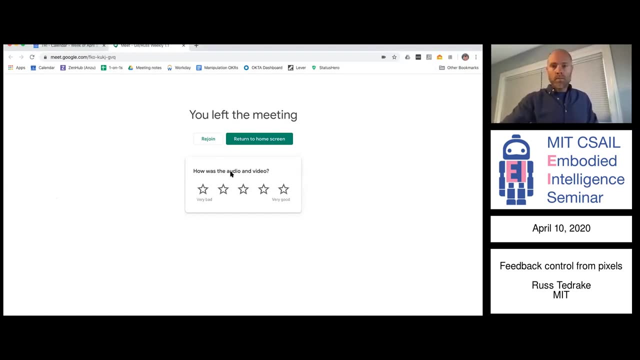 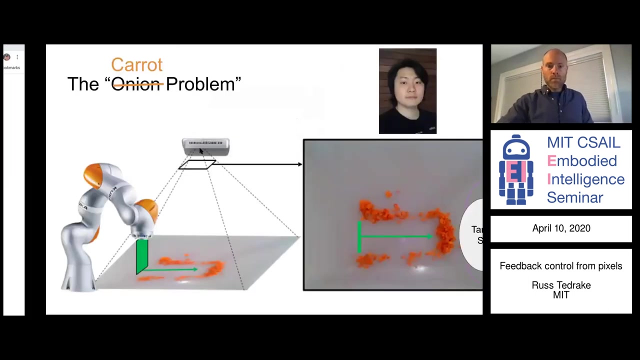 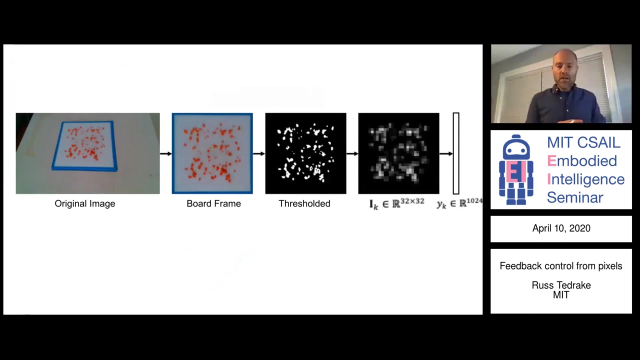 Okay, And I'm going to make a picture of that soon. I see flipping back and forth is going to stink, but let me, I'll try to do it minimally, but here we go. Okay, So the original image here from the camera looking down the board frame. I've now just 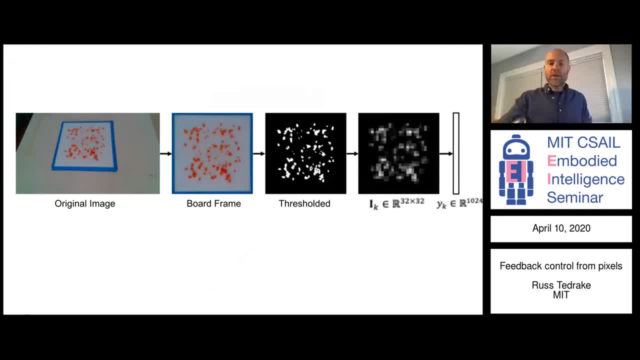 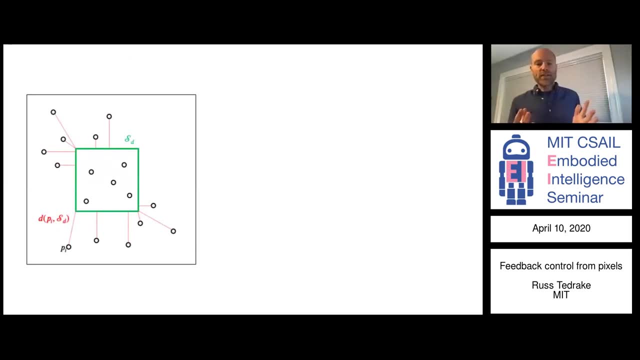 cropped it into the board frame, thresholded it. I've got my now black and white or my grayscale image I and then I can vectorize it into a 1024 vector Y. The notation, hopefully, is clear. yeah, Okay, now this is my Lyapunov function candidate here. Terry's Lyapunov function candidate. 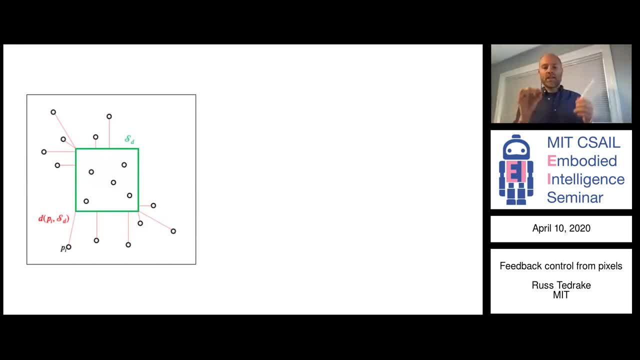 here I've got a bunch of points, a bunch of carrot pieces that we can indicate anything that's non-zero in our image, and I'm going to take the distance between some, every one of those, in the target set, The distance inside there- zero of course. 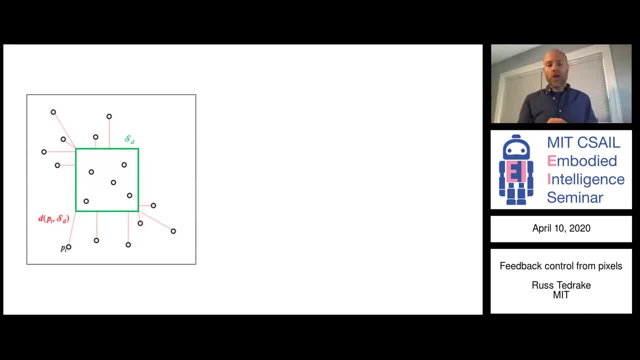 And actually I don't know. Just to take a moment to say that the target set is almost arbitrary. It doesn't have to be. we've made a simple square here. it doesn't have to be a square, but it has to be something for which it admits to control the Lyapunov function. 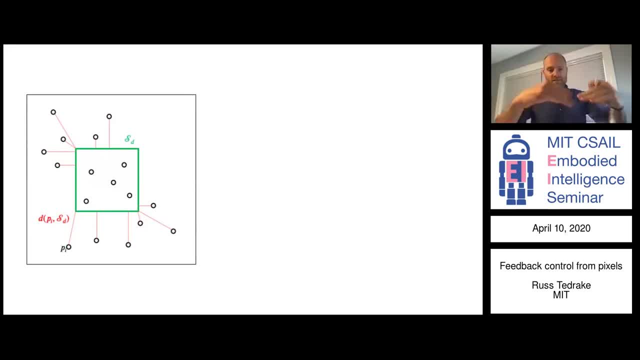 So I'm going to say: you're not allowed to make a target set. it doesn't have to be convex, but it's not allowed to have some weird corners or something such that my paddle, I must have the property that, if I can take a single, there exists a single action of my paddle. 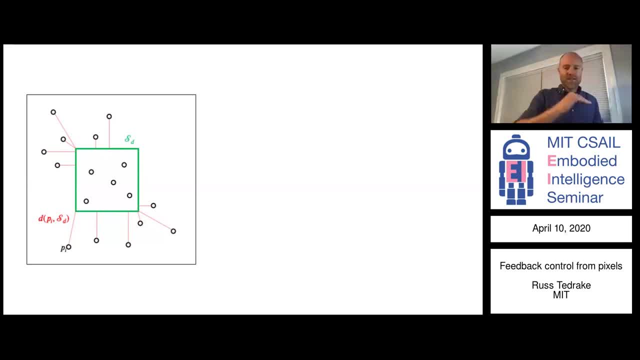 that will make anything that's outside the set go into the set without pushing things that are inside the set. Okay, Sort of a detail there. Now, this is a horribly or not horribly. this is a non-convex function, non-convex problem. 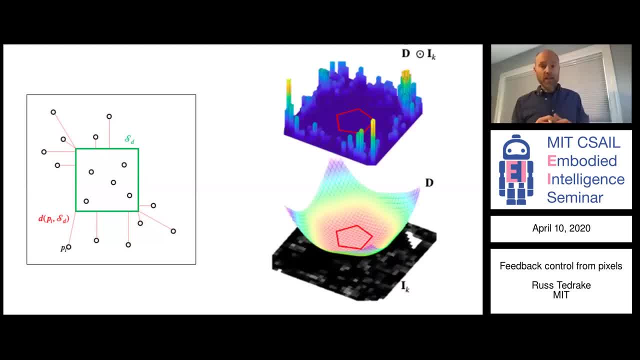 How do we go downhill? And the first observation here is actually that if you write the, instead of writing this, in sort of the space of the different carrot pieces that exist, the xy coordinates, if you write it in image coordinates, then actually the Lyapunov function becomes a linear. 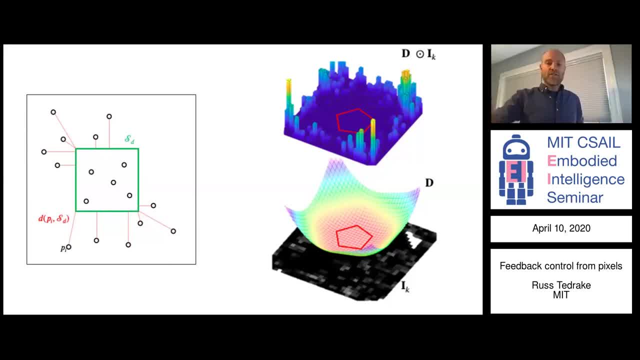 function Okay. So I can take the picture of my. I can take sort of the sign distance, I can pre-compute the distance of every point on the picture from the target set and then I can take the current image and just Hadamard, product it with that distance and suddenly evaluating. 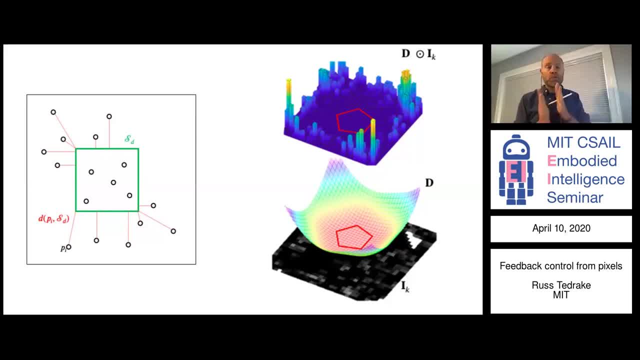 my Lyapunov function becomes just a linear function, So that's already kind of cool. That's sort of the first time somehow the image coordinates was actually easier than the state coordinates of that, And hopefully we're hoping for more here. 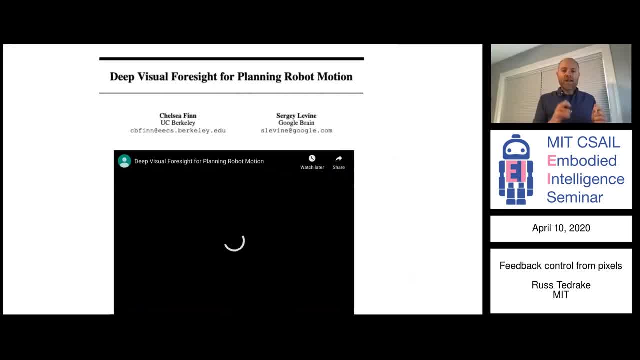 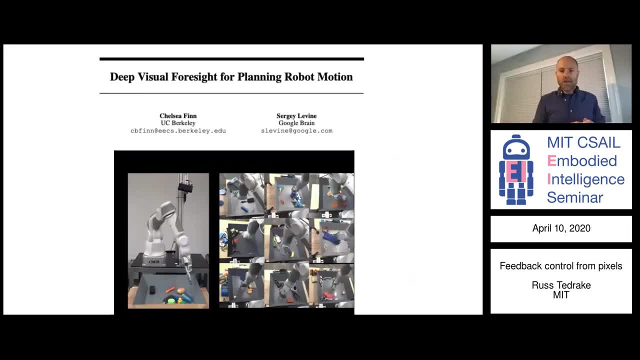 Okay, All right. So the next step is to try to learn a model. So we wanted to learn a model from one image to the next image And we took a page from the Visual Foresight. We wanted to try, sort of the, to replicate the results here. 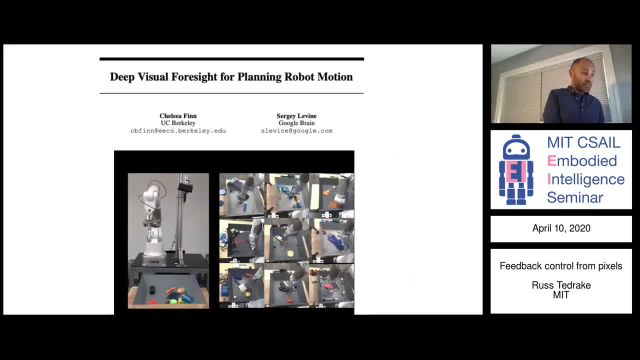 And in fact the story was pretty funny. You know, Terry came to the lab and started working on, you know, this deep Visual Foresight approach. He had a deep network And his first, the first meeting, was like: this is awesome. 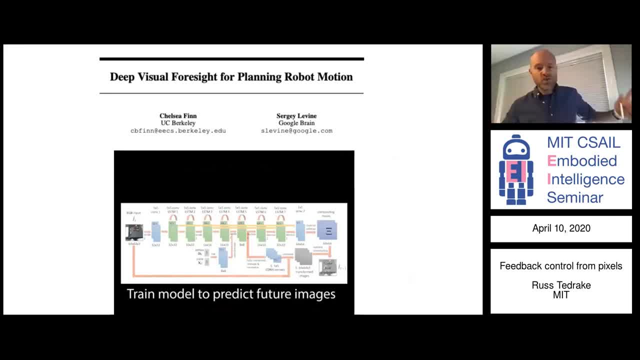 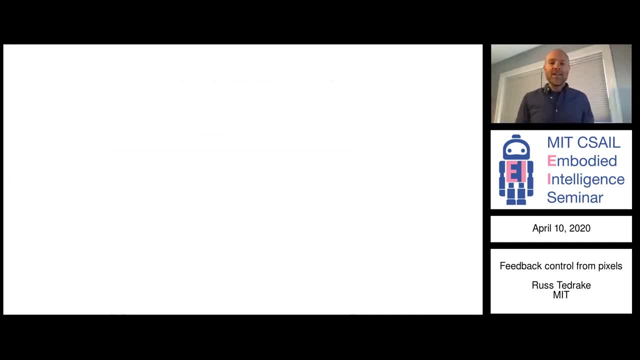 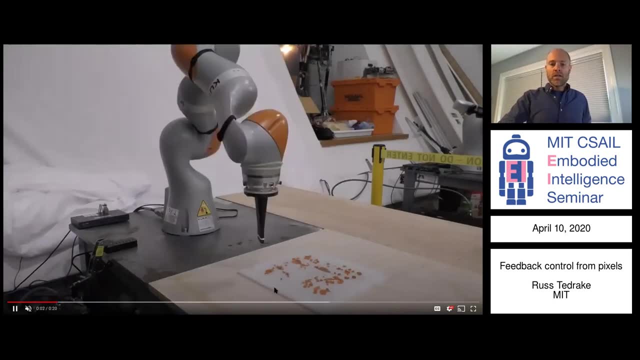 The network is. you know, my training error is like Super low. It's clearly solving the task: Image to image prediction, It just works Right. And then he goes to put it on the real robot And this is what it did. 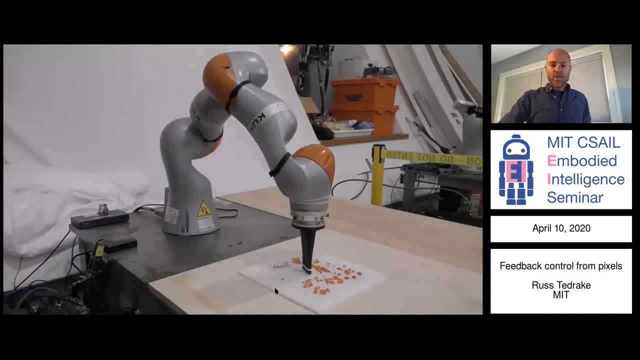 Starts pushing, Doing well, Uh-oh. So, on closer inspection, although the loss function had gone down very beautifully, there was some sort of maddening behaviors And you could say we didn't have the right loss function. We didn't have the right loss function. 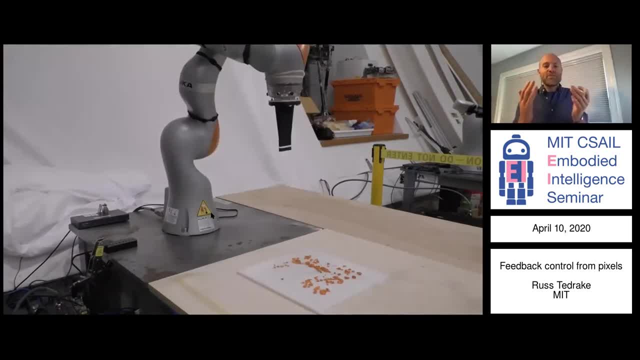 And maybe we don't. But it was sort of incredibly frustrating to not be able to encode some basic ideas into the network, to somehow say, for instance, carrots don't evaporate, Carrots don't appear out of nothing. There was- you know, you should not hallucinate- new carrots. 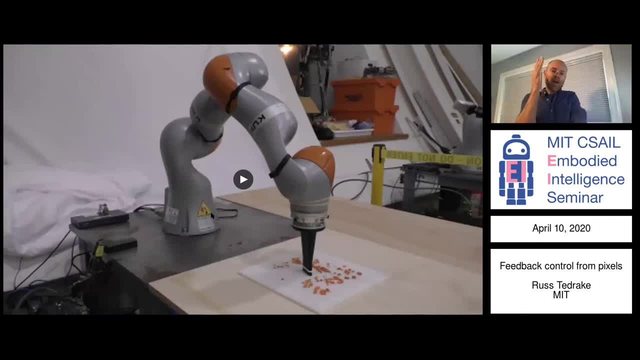 And the conversation was roughly. like you know, it's frustrating because we're struggling to figure out how to put that into the network. It would have been simple to put that into a linear model, Okay. So we stopped and said okay. 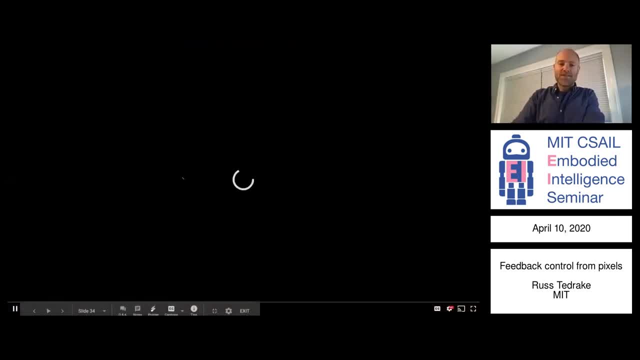 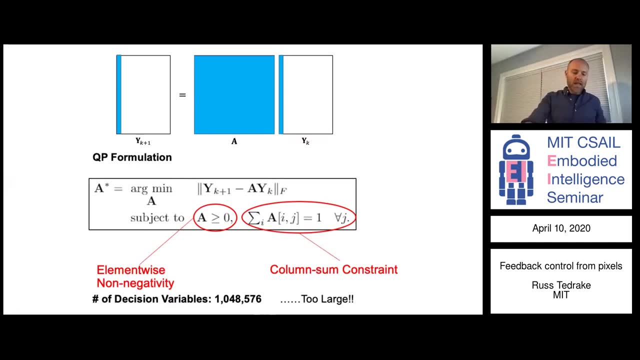 How well would a linear model do for predicting image-to-image translation on the carrots? Okay, And it turns out that it's not crazy. And the reason it's not crazy is that here's a simple thought experiment. Okay, So for a particular push, let's say, in the limiting case, I have just one carrot in the 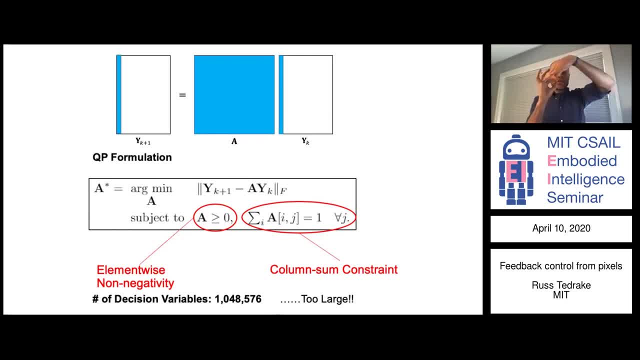 middle of my image and I'm going to do a push. Then that's the operation of pushing- is effectively relocating that carrot to the new spot. That is perfectly encoded as a permutation matrix. I've just permuted the location of my one carrot piece to a new location. 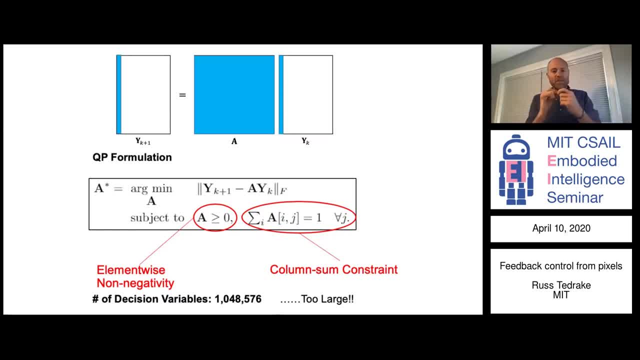 Okay, Now let's say I have a lot of different carrot pieces. If they in the case, with the assumption that they all move independently, it's still basically a permutation matrix. Okay, So I can just say I want to push anything that started off in this cell, ended up in 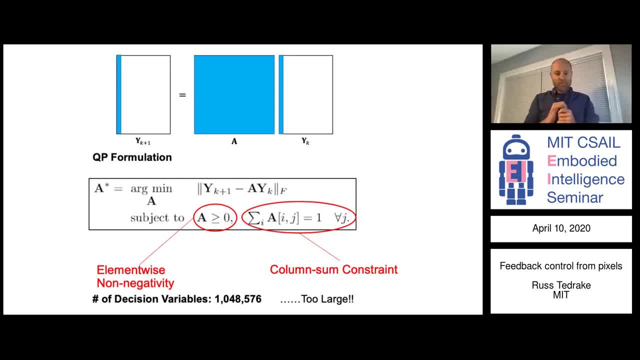 this cell. Anything that started up in this cell ended up in this cell, Right, Right. So the linear map didn't feel as restrictive as we thought it would. Now asking for a perfect permutation matrix was too much, because actually some carrot. 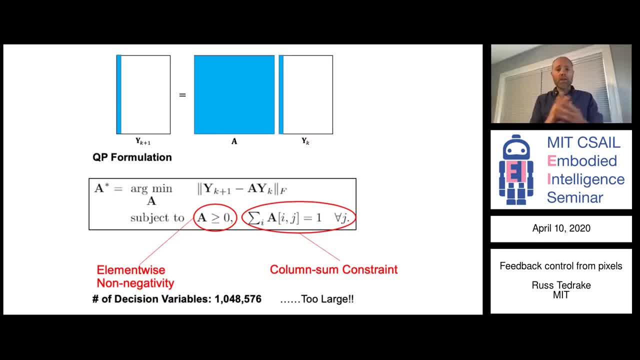 pieces bunch up and they end up being on top of each other and other things. So what we did end up asking for was that there's a. well, what we thought we wanted to do here was to, of course, say that you can't create or destroy carrots. 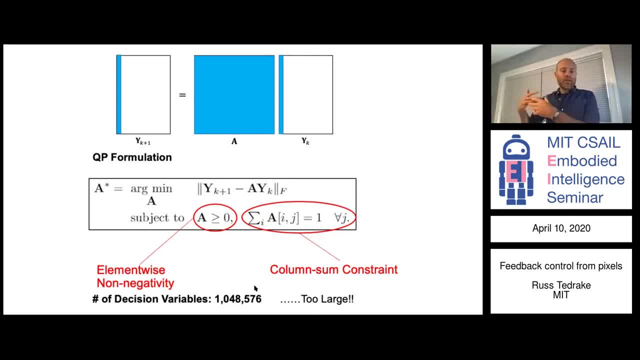 There's an element-wise positivity constraint and then there's a column sum constraint, which is again this sort of mass preservation constraint. Okay, That ends up. of course, you can do now linear. you know, you can do least, constrained least. 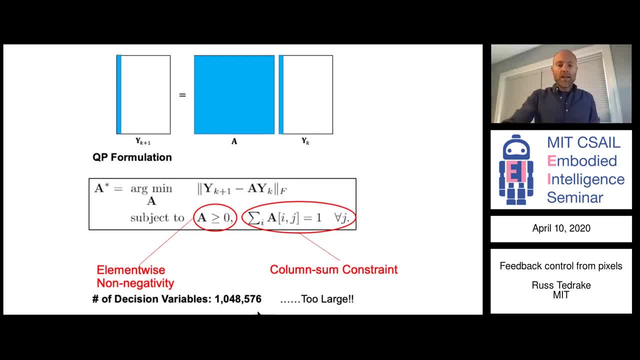 squares, which in this case would be a quadratic program, but because these are big images, so the you know if YK is my image, you know the map A to the next IK, even for a single push, is already 1024 by 1024, so it gets to be too big to be useful for QPs especially. 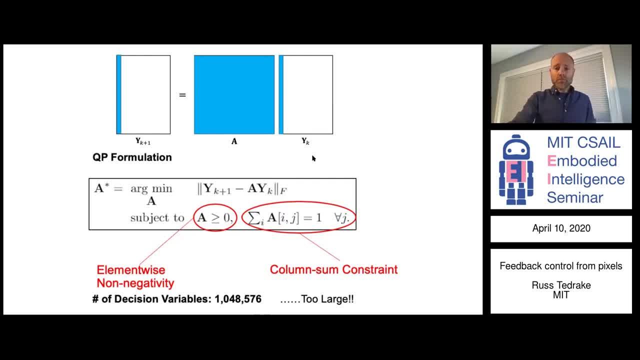 if you have to do lots of different actions. So we ended up dropping the column sum constraint and that way you can solve each row independently, okay, and just decompose the problem into a lot of smaller problems. And then we actually checked after the fact and found that in fact, even without that, 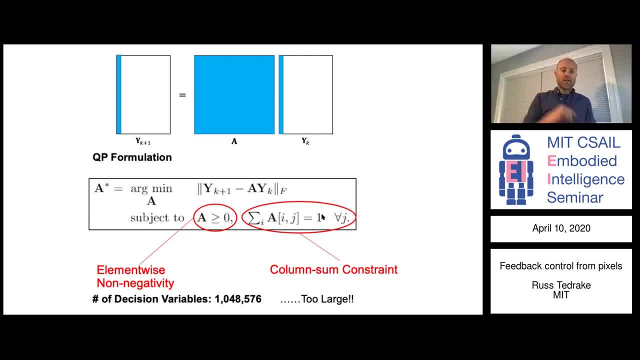 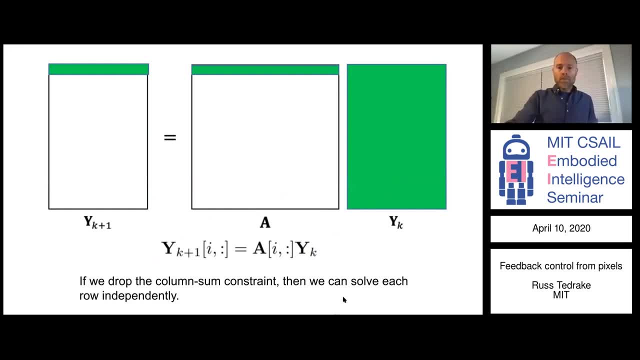 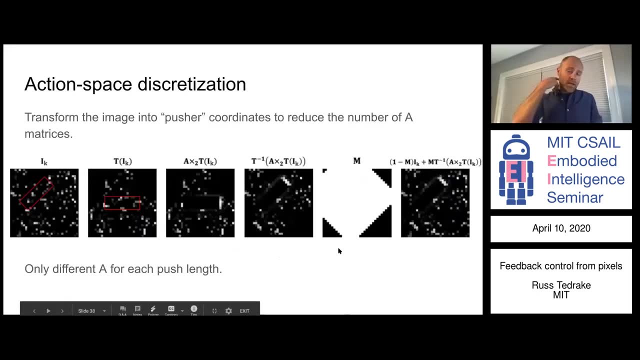 column sum constraint just to match the data and have the positivity constraint. we ended up the columns typically summed to approximately one. Okay, So we saw, In that case we can solve each row independently smaller optimization problems, But that's only for a particular action. 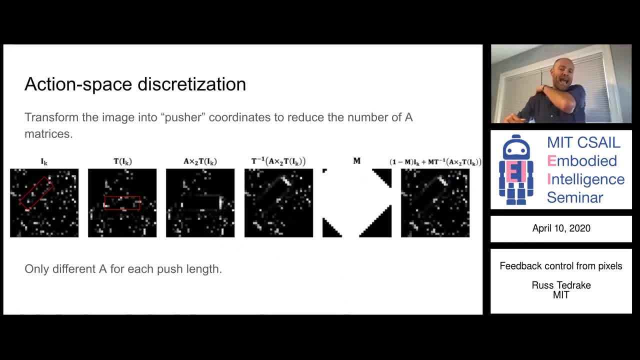 To do a little bit better. we tried to transform all of our data into the action frame. This is a standard sort of trick in the visual foresight type worlds, So you could take any particular swipe of a constant length and then basically rotate. 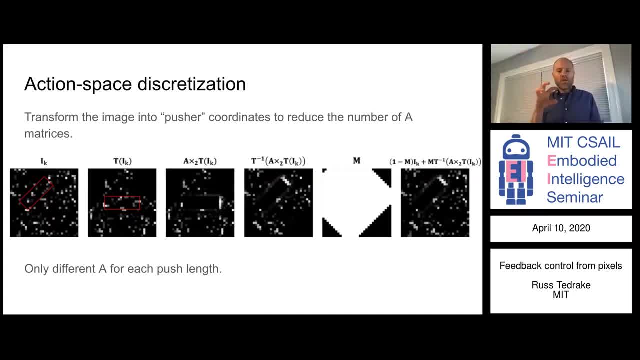 translate, fill in the background, come up with, you know, with your mask and basically reuse lots of your data in the coordinates of the push In order to for a lot of different, you know, with a lot of, with relatively small amount. 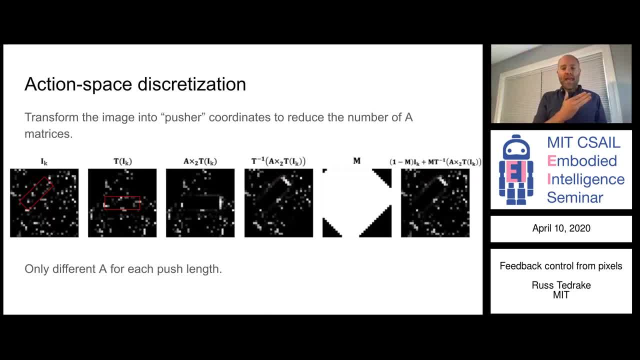 of data. we could train a good A And we actually only have to think about A's being discretized on the length of the push and not the position orientations and everything like that. That dramatically reduced the amount of training data. It was something we could have done, and we did do eventually with the deep network approach. 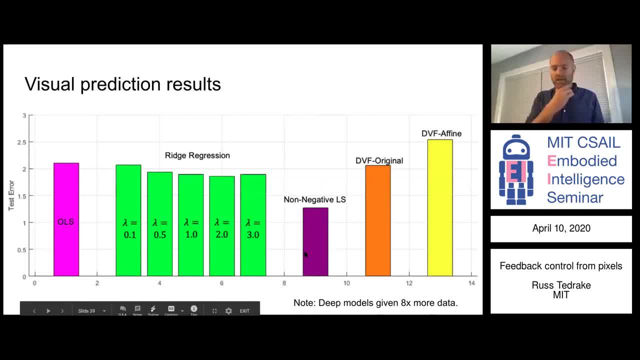 but we it was. it occurred to us when we were thinking about it in the simple case. And then what was surprising was with the amount of data we tried. Actually, the least squares models work better than the deep foresight models. Now, that is absolutely not me saying that linear models are better than the deep models. 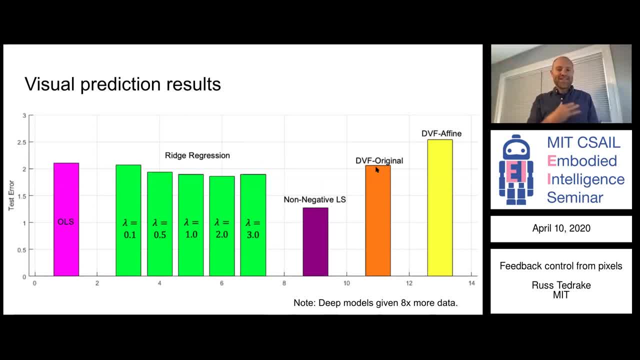 because deep models are a super set right. But I'm just saying that in the amount of data we had here, there was a sort of a stronger inductive bias on the, you know, on the linear, the constraints we were able to put on the. 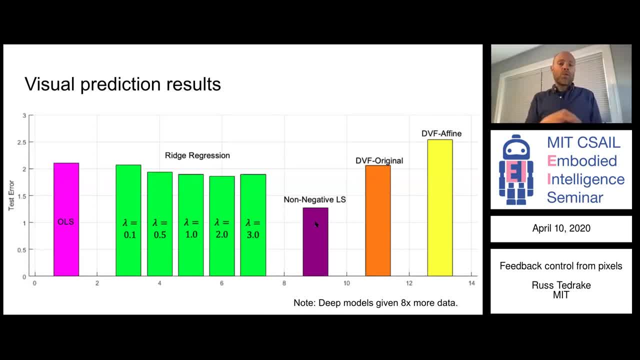 linear system that the non-negative least squares is the one that did the best, was able to match the data You know, with a lot less data actually than the deep visual foresight, the original being the one just doing it. image to image the. this is the one with the deep visual foresight. 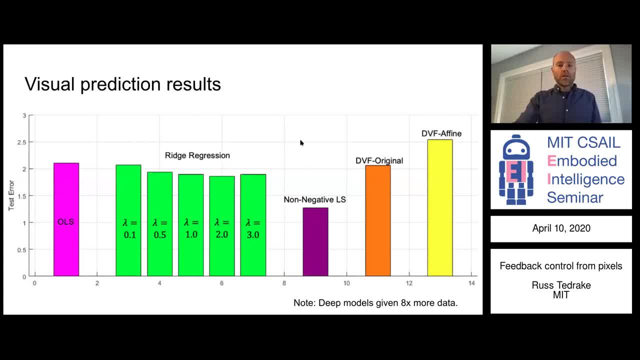 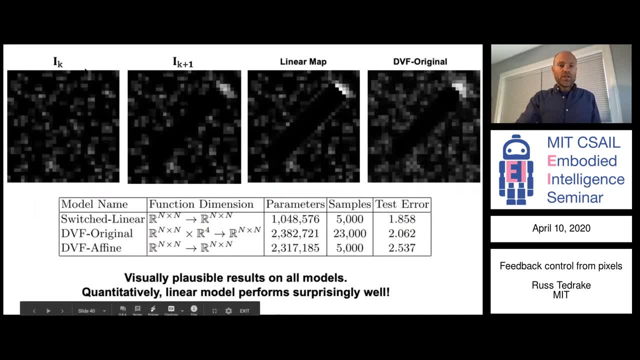 also given the benefit of doing the affine transformations for data augmentation. Okay, And you know it actually worked surprisingly well. So you know you could, you could see the, the linear map here, the actual transition from one thing to the other. the linear map would predict, you know nicely, and the the 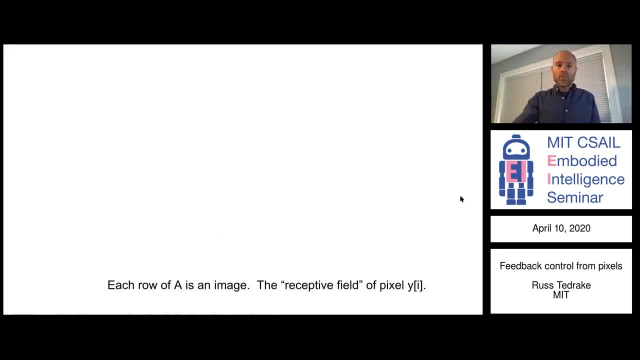 training, training and test. error played out Okay. So you know each row of A is an image, so you can actually sort of go through and look at the the same way people look at the receptive field of a neuron in the middle. you can. 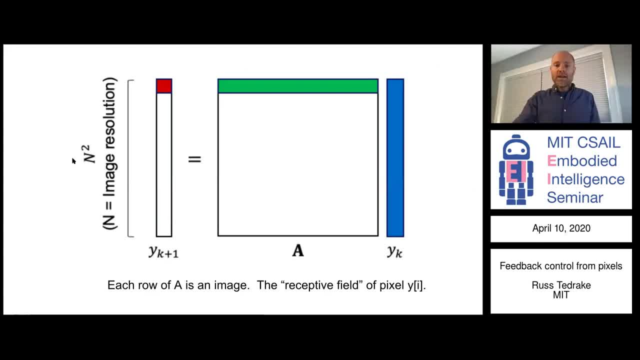 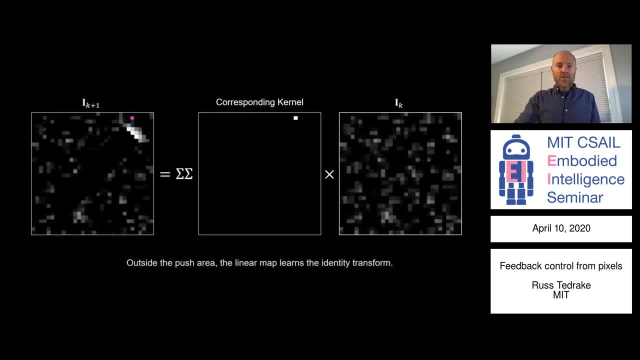 you can go and inspect how it learned in the in, in the middle, and and and visualize it and it. it's pretty compelling. It does seem to do all the right stuff. Okay, So this is now the you know. we expect it to effectively learn the identity map. 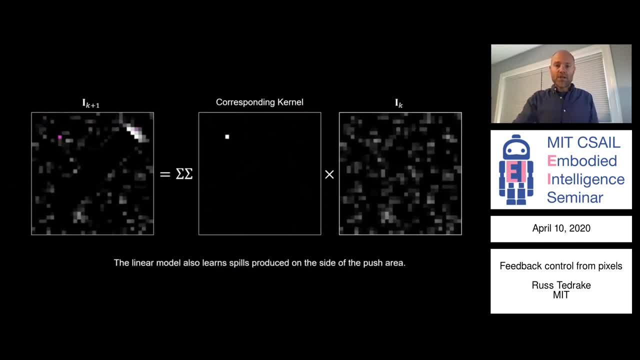 Until it goes here, this is the pre-image of of the pixels. Okay, So the pre-image of the pixels up to here is just the pixel, because it's the identity map, And then, when you get to the part where the push happens, there is nothing in the pre-image. 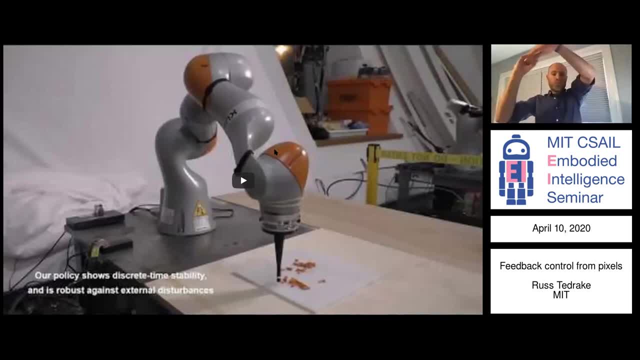 for the one that's inside the length of the push, but the ones that were at the boundary of the push have the whole sort of pre-image- is the whole stretch of places that could have landed it too. So it was doing, intuitively, the right thing. 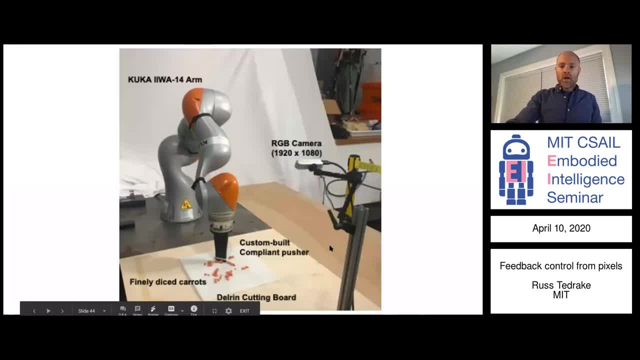 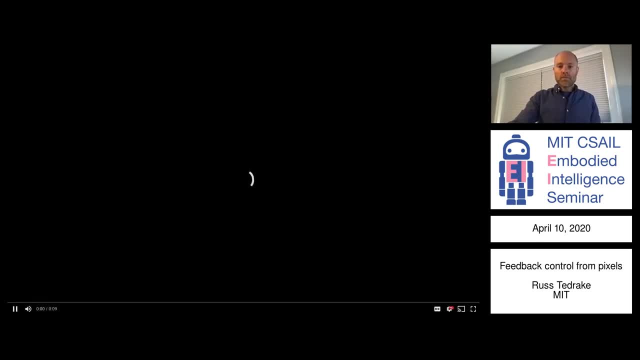 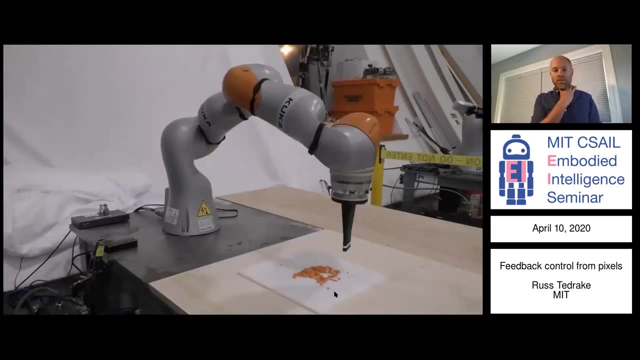 Okay, So Okay. So we put this back on the KUKA to run the experiment. Here we go. It works surprisingly well with the, the linear model, Okay, And ultimately we evaluated ourselves based on both the, you know, the image to image prediction. 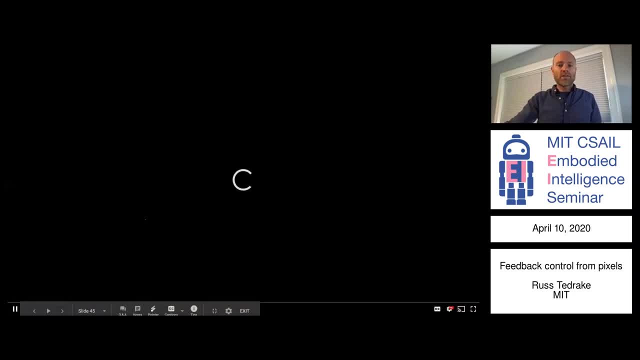 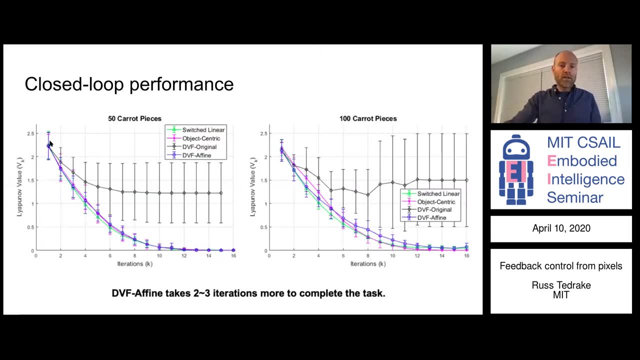 model, but also the closed loop performance of the controller on the task. Okay, So the closed loop performance, they all did ultimately fairly well, except for the maddening case of getting stuck on a hallucinated carrot, which was which the original deep visual. 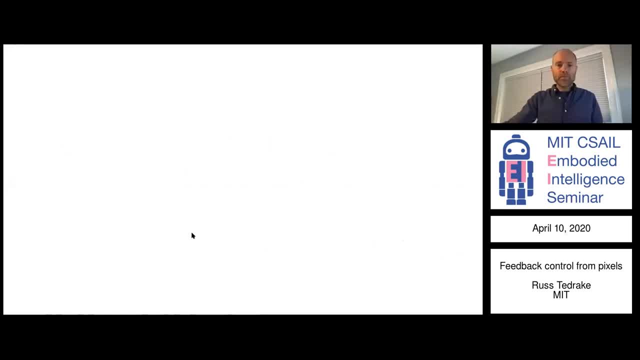 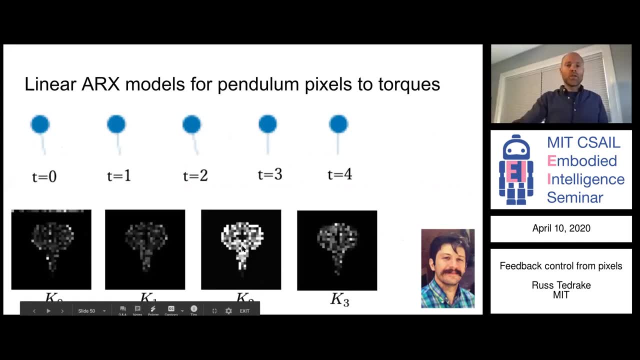 foresight model was was subject to. Okay, All right, So I know I'm running out of time. Sorry for the awkwardness with the with zoom here. So the obvious question is: how far can you get with this? And I think we know. in fact, we came from a group. 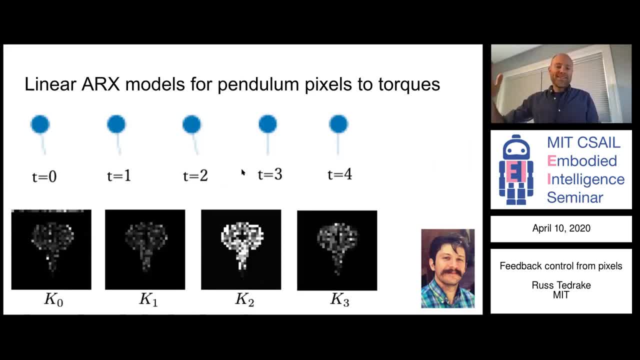 We had a group meeting like two hours ago. We had a group meeting like two hours ago in which Terry presented again and he basically spent a half hour saying it's never going to do more than the onions. And I'm like I said, Terry, I'm about to present your work to a whole bunch of people. 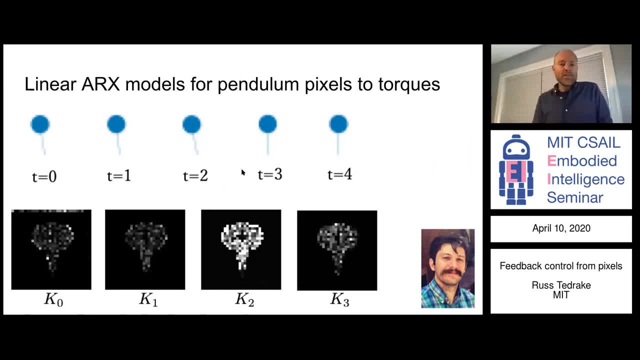 and you're telling you know, but I think we know the limitations of this. I think for now, you know, we now have, I think, a clearer understanding. I mean this is very much like sort of the Koopman version. if you will, it's a nice. 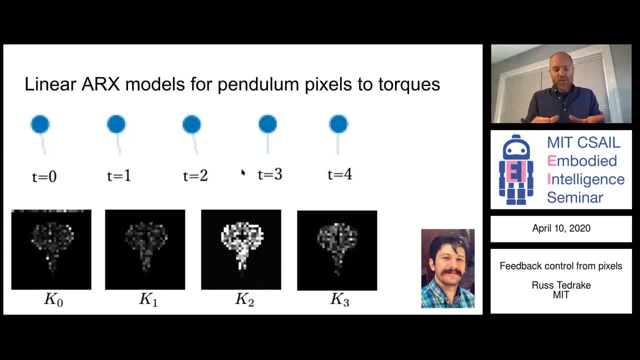 story where, If you lift the pixel, space is sort of lifting us into this higher dimensional space where, under the specific assumption that those pixels move independently, the linear map does a perfect job. in, in, in summarizing it: Okay, As soon as you break that independence assumption if those, if it's a, if those bodies are connected, 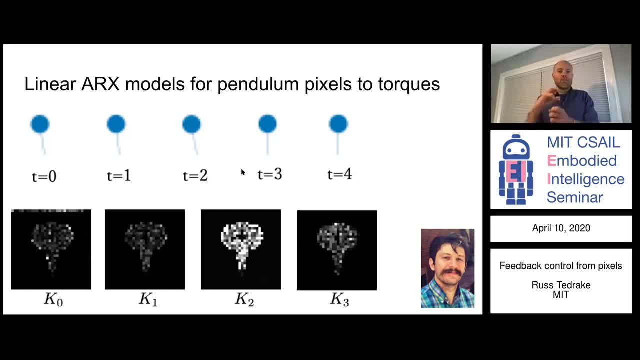 to a rigid body, then we're. then we're in a different regime, right Where the linear- we don't expect the linear model to do well, and actually well you could. you could lift it up, You could have a higher dimensional space and expect linear models to do well. but in 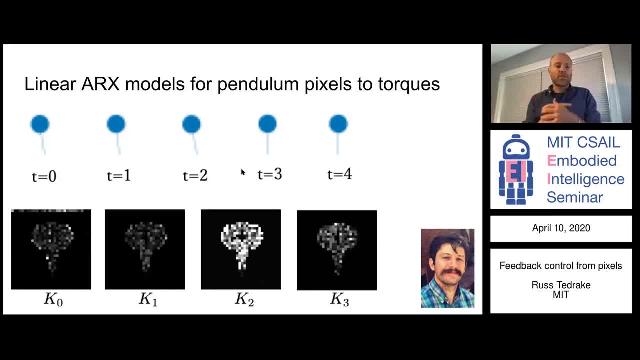 the image space. you only expect it to do well on the limit where the pixels move independently. Having said that, we can use robust control type ideas, for instance to fit approximate ARX linear models, And Sajar has been doing this nicely to try to do some of the classic tasks in image based. 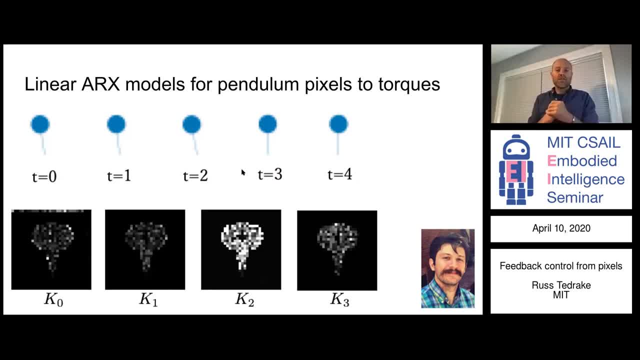 feedback. Okay, And uh, it's a story that's still emerging here. Sajar actually sent me more material this morning that I was able to slide into the talk. Sorry, Sajar, But um, but you know, this is an emerging. 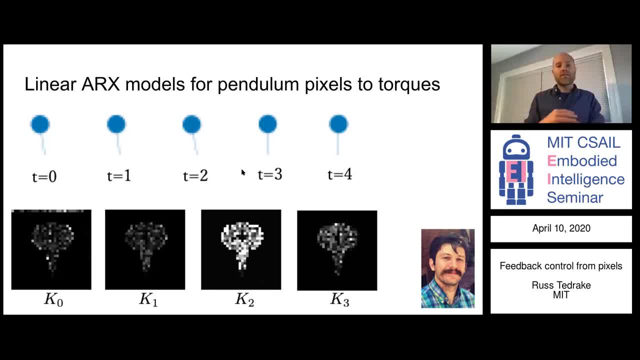 This is an emerging story of trying to understand how well linear, robust control can actually do in images, And I feel like we finally have at least sort of the what's the simple case when next time we say: you know what was the simple case? where, where vision based control is easy. 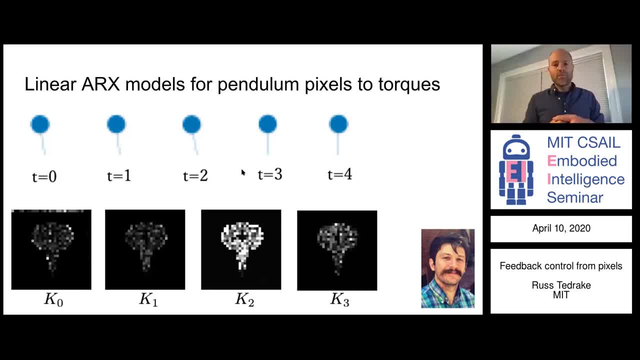 I think the answer is now, when the pixels move independently and actually carrots are the case, or an instantiation of that case, that I don't know. I mean, it wasn't, it's not my life dream, but it's, you know, it's still it's, it's a real problem. 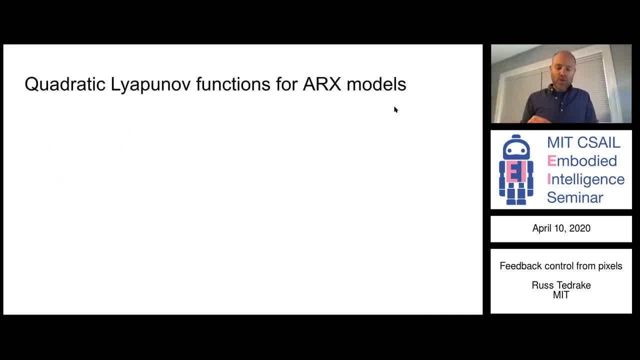 Right. So, um, and the cool thing- and I was planning to do more on the way on the board here, but, um, the cool thing is that there's a natural, there's a whole bunch of tools that open up to us from the controls community. 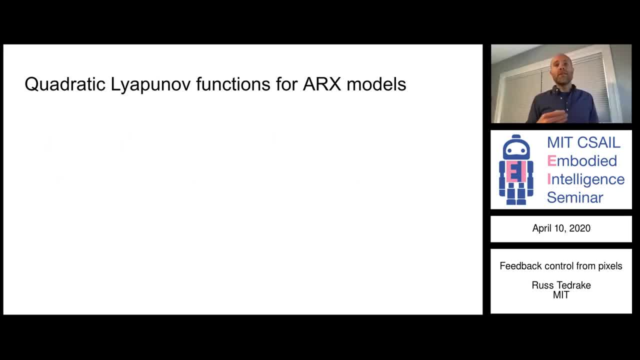 If we're in this space, especially of linear models. but even I think the next steps are going to be looking beyond linear models, piecewise, piecewise models, nonlinear models, but there's natural extensions of the tools we know and love. 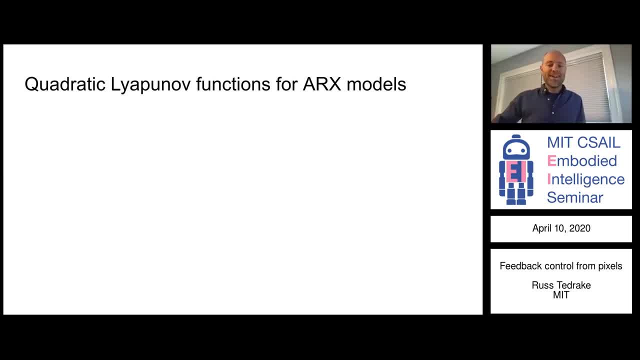 For instance, Sajar, Okay, Okay, So we're going to look really quickly at the macaroni equations for ARX models in this space and looking at the open off functions which now take. it's a quadratic function of the history of images and the history of inputs and it predicts that you could then predict: 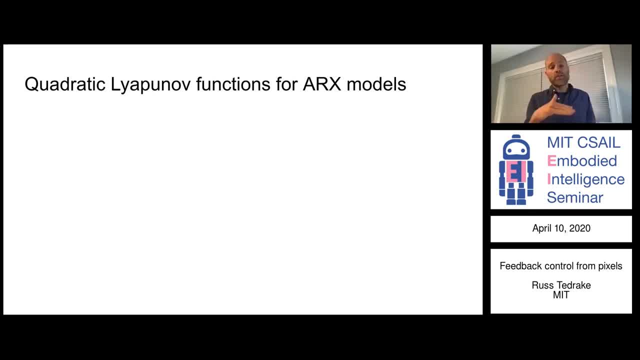 that you'd like to go downhill on that function And similarly you might be able to check, you can, might be able to monitor yourself and if things are starting to go wrong with your vision based control, you could. you could detect that quickly if your Lyapunov function starts going uphill. 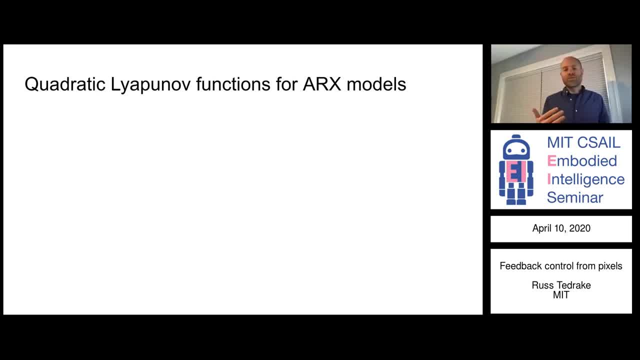 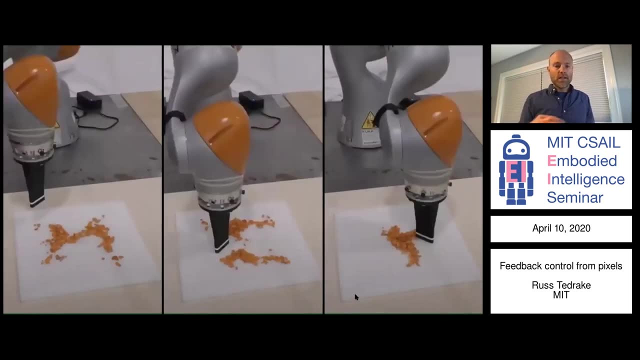 Okay. So I think we're at the beginning of this, of this really nice sort of opportunity to think more rigorously about the vision-based control stuff. Okay, so obligatory. let's move the carrots into an MIT pattern, Okay, but I'll basically wrap up there. 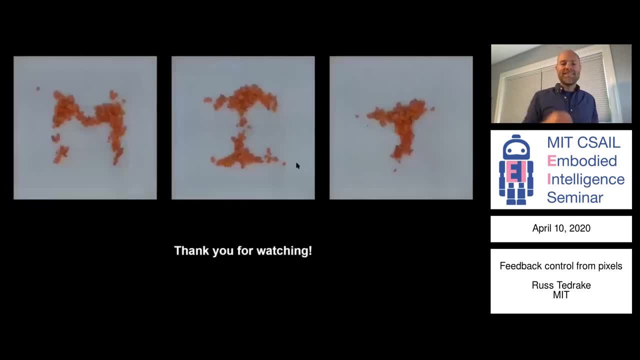 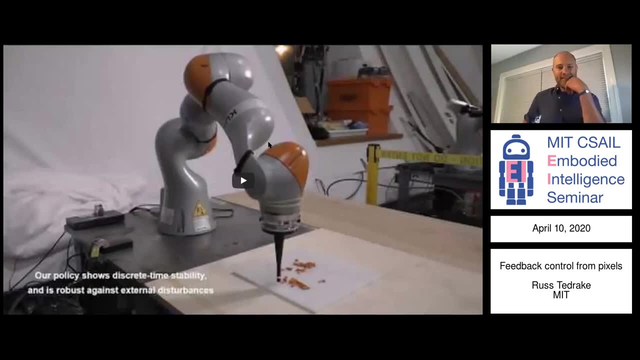 and take any questions. 259.. Maybe we have time for one or two questions. I'm happy to stay, I have time, but please ask anybody. Hey, is my microphone working? Yeah, hi, Geronimo. Hey, I was wondering, can you give? 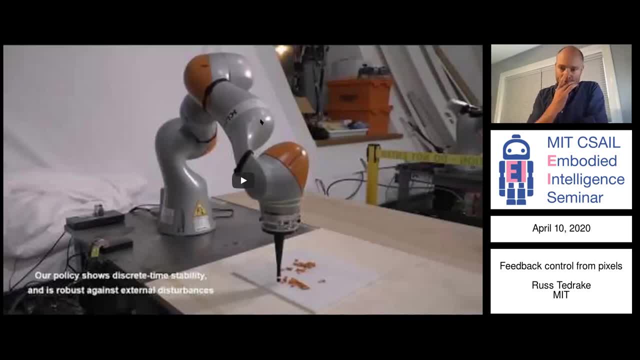 I was just trying to conceptualize when you said that basically the pixels have to move independently in the task for it to be a linear controller works. Do you have like an example of one where the- I mean that might've been one on the screen? 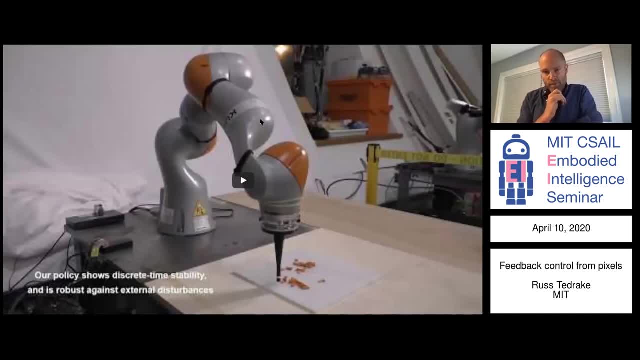 but like where one, where basically, the fact that the pixels don't move independently causes the controller. just you can't represent it. Let me say it back to you. So I think a linear image to image, you know, linear forward model can describe the data well. 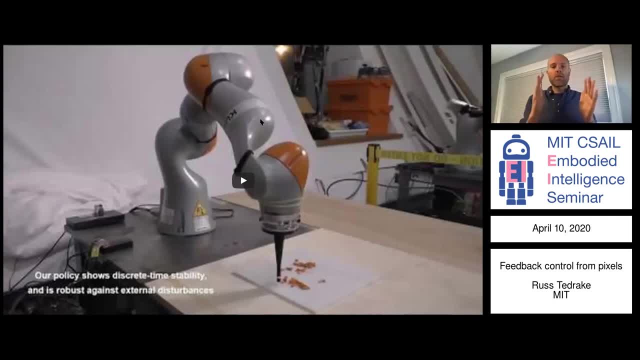 It's not a statement about whether a linear control can work well, but it's a statement about whether a linear prediction can work well. And I think, as soon as you get so, we already see it a little bit, because, in fact, when carrots do bunch up, 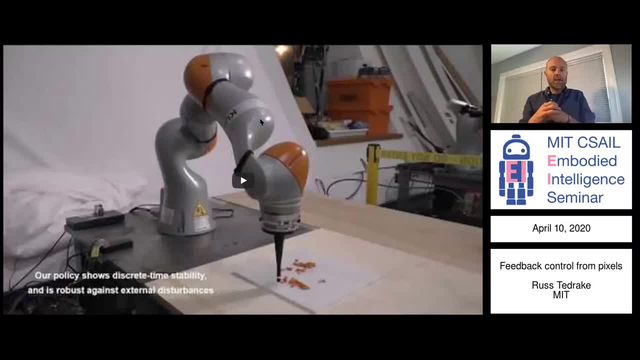 they will push each other around, And that is a violation of our basic model. That isn't captured, but it but it's captured, well enough to accomplish the task in this case. Yeah, Now that makes sense, Yeah, Yeah. And if you were to now try to push? 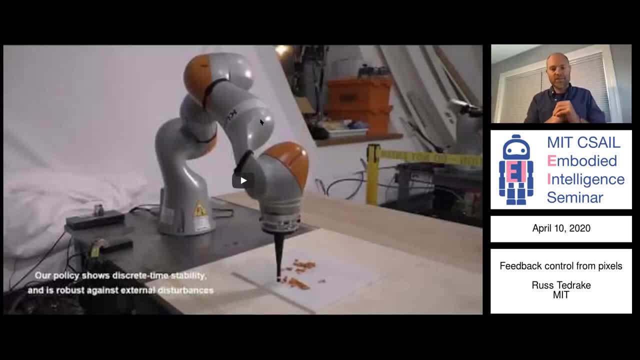 a big domino sugar box, for instance, then then you'd see that that's quickly violated because there's a rigid body assumption, that a rigid body constraint that holds those pixels together Right Makes sense. It has a quick question. Yeah, Yeah, Luca. 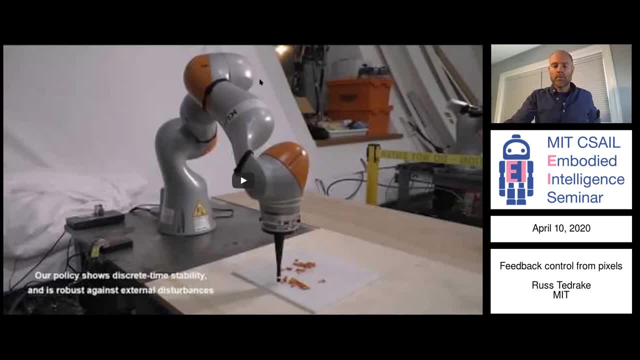 Yeah, So I completely agree. First of all, very cool talk. I really liked it. So I completely agree on the idea that somehow, like you know, the representation for the robot should be like something that is task driven Right. 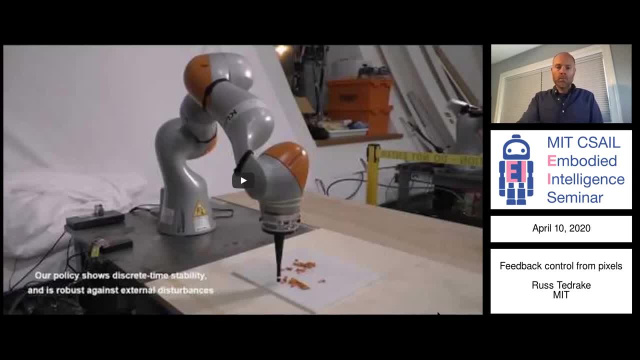 I was wondering if you thought about this. It's clear that you know, in the case in which I have a single, very specific task, you can engineer like a representation which is more clever. For example, you can get linearity out of the representation. 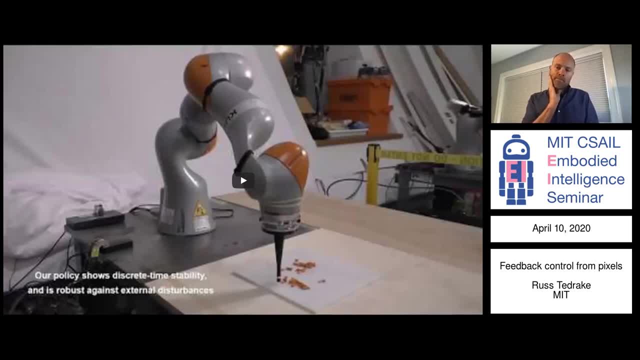 But I'm wondering if you start considering many, many tasks. you know a robot that has to do general purpose actions in the apps, for example. I wonder if, at the end of the day, to support a variety of tasks, 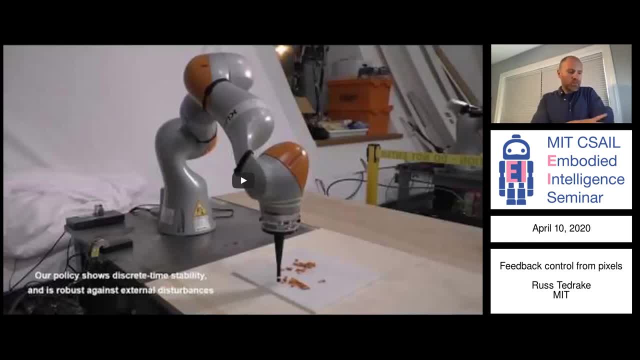 you end up going back to a full state that you have to build, In other words, like it seems that if you have to do many, many tasks, at the end of the day, thinking about the 3D representation on our objects, 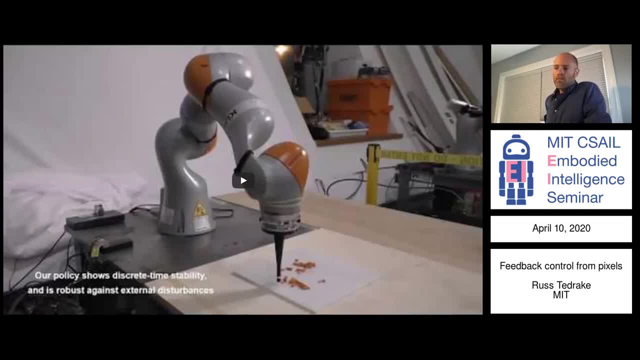 end up being like the more clever and general formulation for the state? I think that's an awesome question. I completely understand your question. I've been thinking along these. I've been questioning myself in that way, I think actually so I think the diversity of tasks. 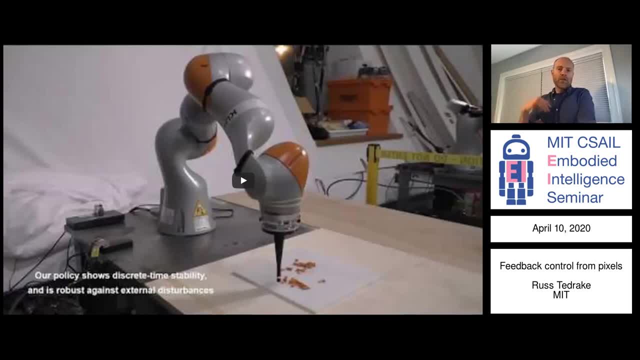 that we want our robots to do is far greater than anything we're trying right now, But it's actually probably not the case that we have to like. I don't think I ever need to know the state of the salad, right. I mean, I'm never going to ask the robot. 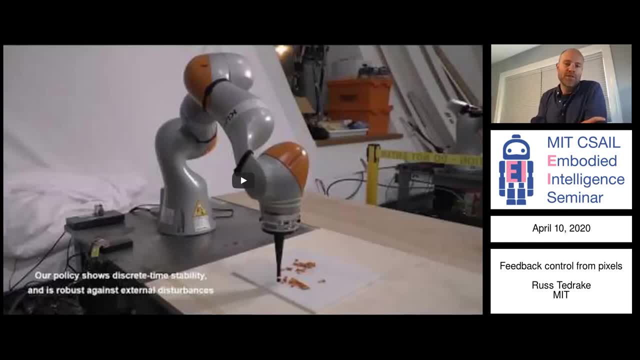 to have to distinguish between crouton 13 and crouton 14 or whatever right. So I think there's, you know, there's something there. We probably don't need the full state ever. The other, the more subtle thing though. 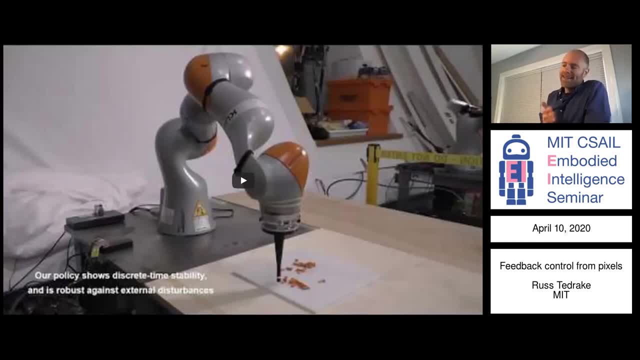 I would actually I'm of the opinion today- ask me again in a few months. but I'm of the opinion today that asking for one task to work might be a harder problem than trying to get something that works for a diversity of tasks up to some point. 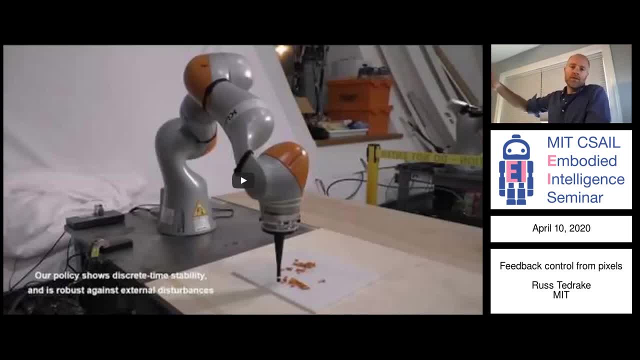 You're right that at some point, maybe if you're trying to do too crazy of a set of tasks, you have to know everything about the system. But I think we're almost possibly making the problem harder by having a very narrow specification, And maybe my analogy for that is: 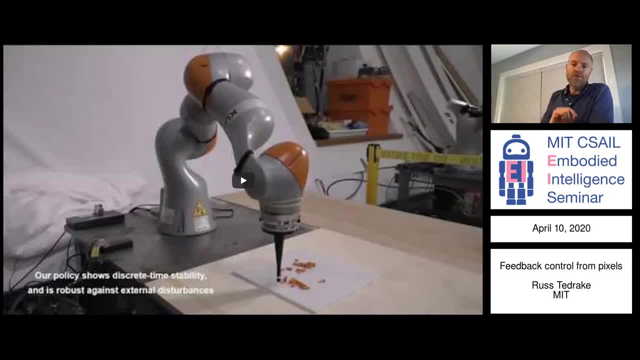 if you look at even like trajectory optimization versus stochastic trajectory optimization. if I ask my, if I give myself a particular system, a particular initial condition, you try to solve the problem. there's lots of local minima often, And if you say that the same controller. 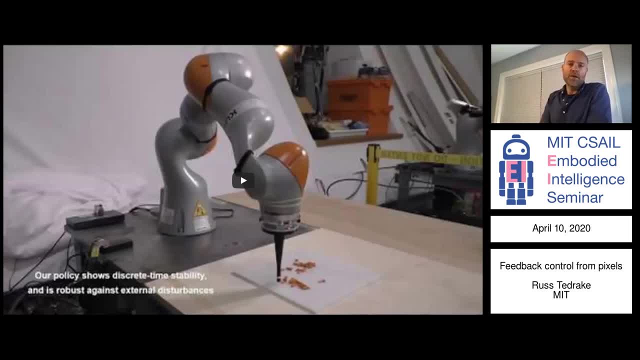 the same control inputs have to work for many initial conditions in a stochastic problem. then actually all the non-robust solutions tend to fall away and the optimization gets a little bit better. And I wonder if that's going to happen in the task place too. 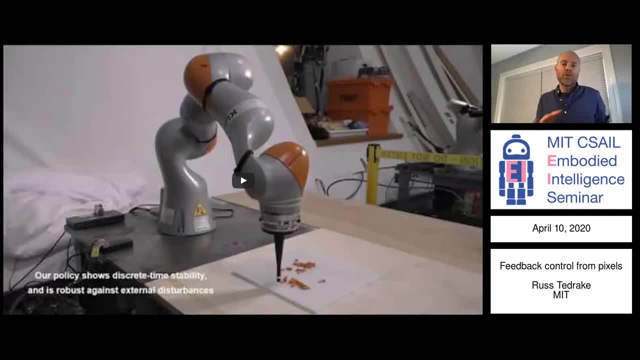 that if you ask the system to do many similar things, it might actually help us discard the quirky solutions that happened to work in a narrow case but didn't make sense, and it might actually make the problem better. So I'm hoping to look into that sort of first step. 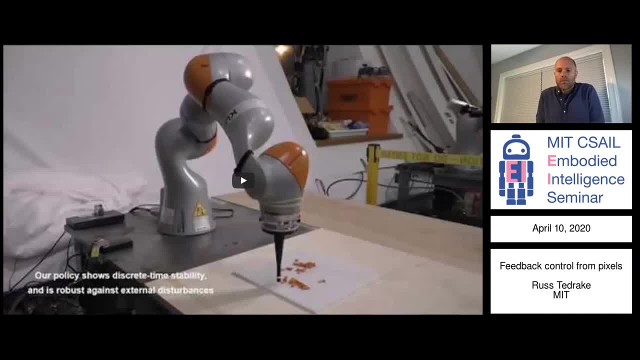 Good Thanks. Any other questions? Okay, then let's leave it here, since it's past 3 pm. Thanks a lot, Doros, for a great talk. Quick question about the There you go. I think that might have been Katie, yeah. 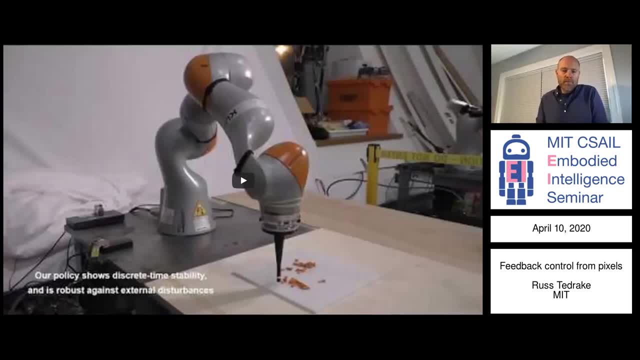 Yeah, go ahead, Katie. Hi, That might be a little unstable. No, it's just a question about the 3D nature of the problem, The pixels that you take. do you see any shadowing Is there You talked about? 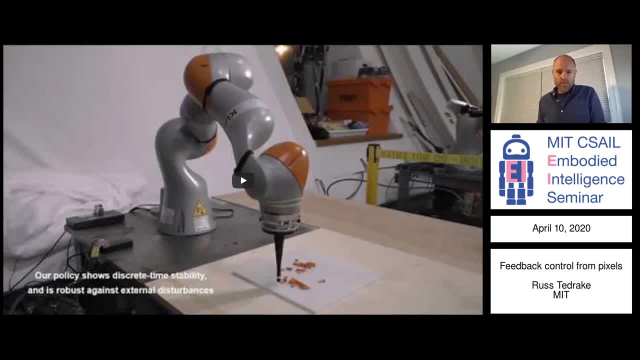 I think you talked about column summing to sort of a containing of everybody having their own location that isn't stacking on top of each other, isn't occupying the same pixels, that kind of information Do you think you could actually tease out some information? 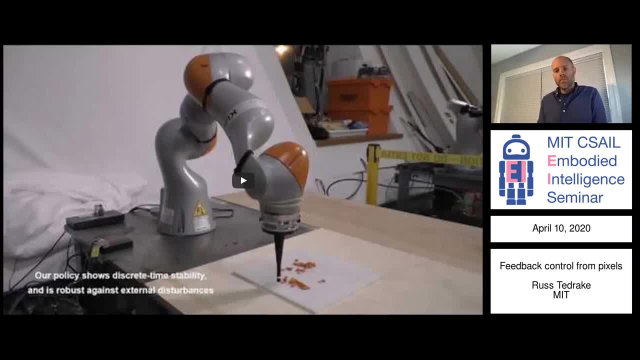 from the shading of the pixels to give you that more 3D information about interactions? It's a good question And is the linear thing still hope of working, Even when you do have those interactions. kind of going back to questions, to draw on most questions. 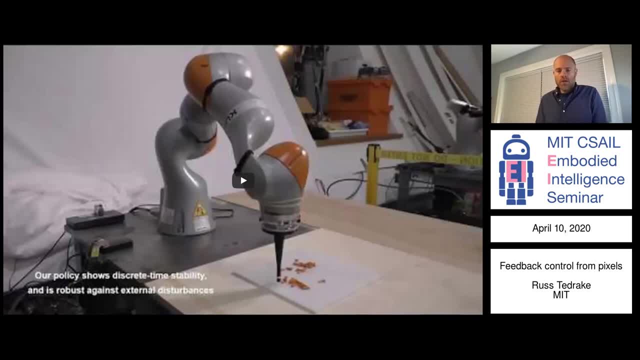 building off of that, following up: Yeah, yeah, thanks. So I think it is actually doing that to some extent, which is why, actually, we couldn't ask for it to be a permutation matrix. Having the rows summed to one didn't actually work. 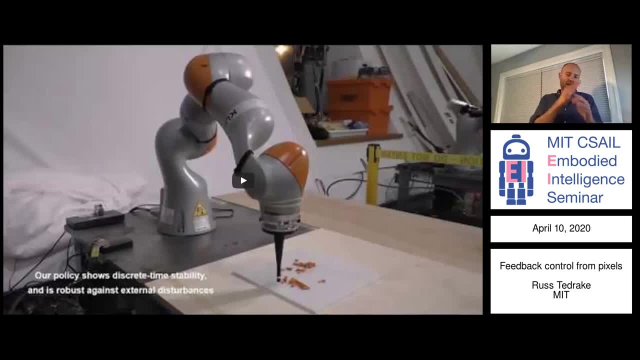 because almost every case, in fact, if there's two pixels or two carrots on the same line, then they will both end up in the same place, and we have to allow the system to have a value that was greater than this. Somehow, it was the sum of those two values. 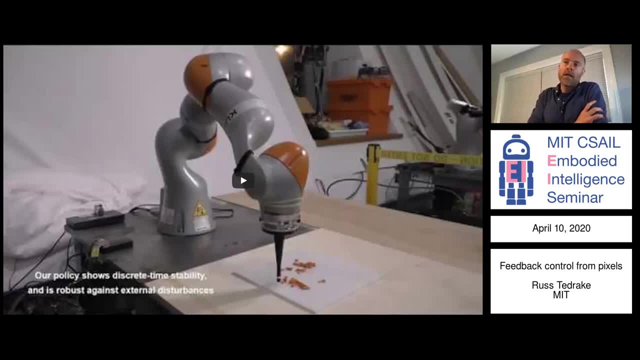 So we actually saw that in the data, that we had to allow that and it supports that. But the thing that it really can't support is that if the interaction between those two particles caused any one of them to land in a different cell, that's the part that the linear model cannot capture. 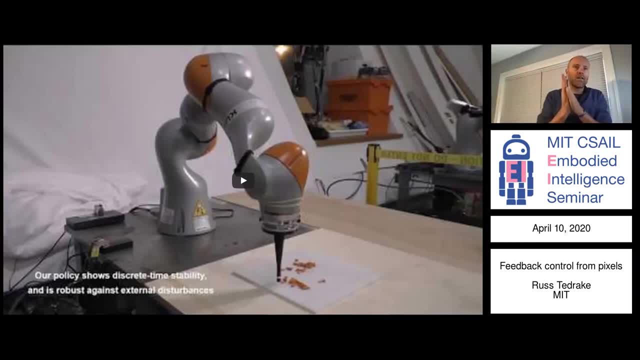 So summing them up is fine and to some extent the 3D is roughly a sum. I mean we're approximating it, but the data is approximating it that way. George, you also had a question. Yes, 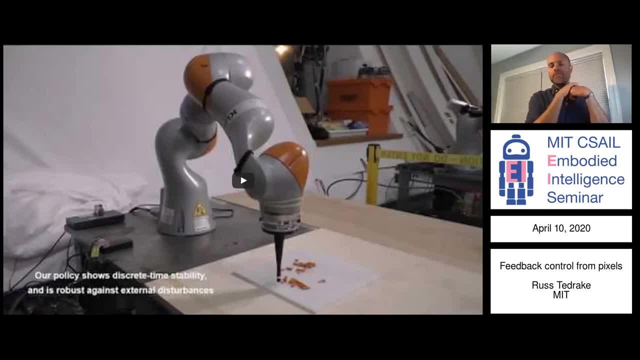 I had a question on. it seems that in this specific case, with the carrots, you've more or less chosen a state representation such that a linear model can predict it. well, but you also talked earlier about learning or not. state representation maybe, but some sort of representation. 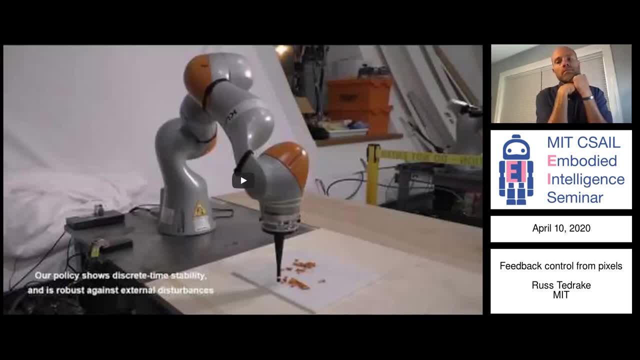 You also talked about a representation being sufficient to do the task as a way of learning it. Do you have any ideas about combining these two sort of things? maybe Awesome. So in my mind, the ARX model is powerful in the sense you don't have to name a state representation. 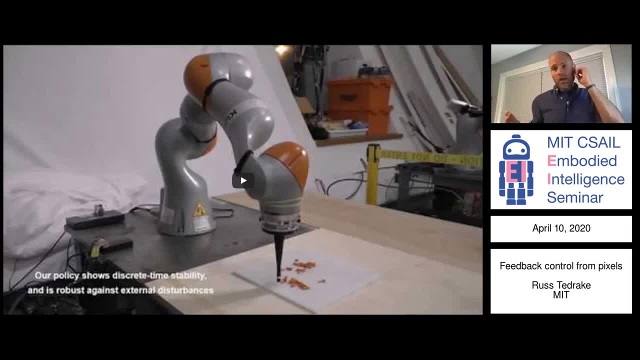 It's massively inefficient in terms of data right, And the size of the matrices we're learning are enormous right, Which means we're- I mean I could say we're- over-preparated, and maybe that's what makes it sound good. 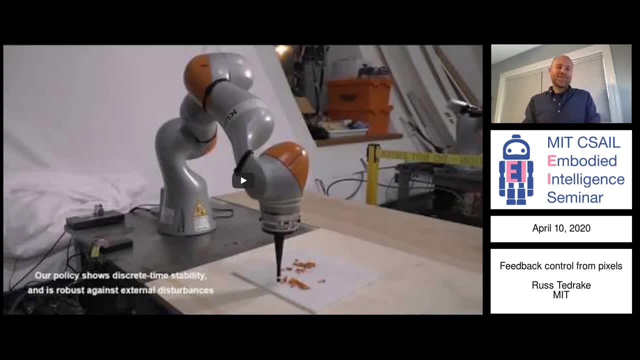 but we also just need tons of data to feed it. So, to the extent that linear models work well, there are well-known techniques for output feedback: output system identification, input-output system, identification- where you do subspace identification, and there's rigorous approaches to defining the latent space. 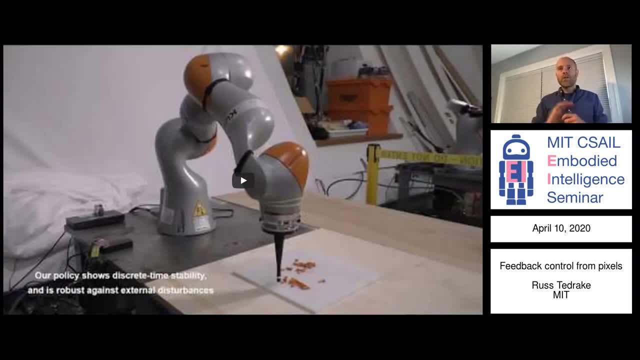 Right. So I think there's a big question of I think we know that the linear models are going to taper in what they can handle, but there's a whole world of linear, robust models where you're saying it's linear plus or minus some bits. 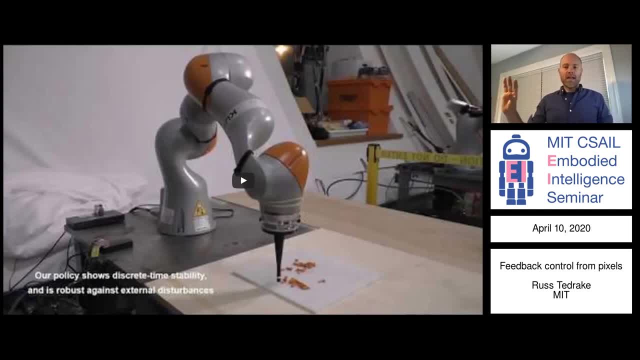 and I don't know if we. I don't know how much to expect out of that yet, but I long for the ability to bring in some of the more mature models in system ID and state representation tools that we have from systems theory into the problem of like images. 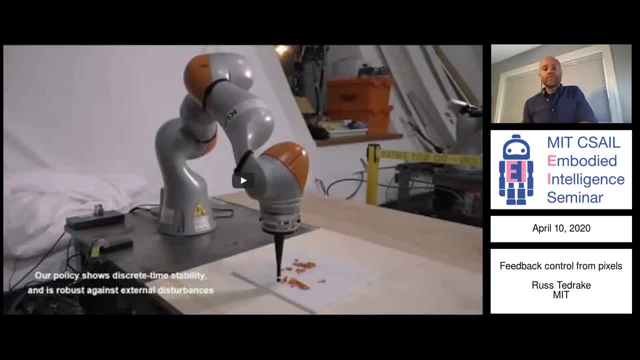 So there is a route, There is a route forward. Sounds good. Thanks, I think you also had a question. I think You're muted. Isaiah, There you go, Got it. Thanks for the talk, Russ, Really interesting. 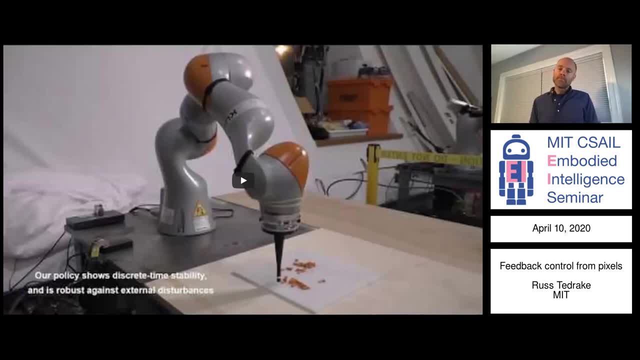 So you were talking about potentially acquiring representations that were not representing the full state, as in for certain tasks. we don't need to keep track of different things, but obviously, if we want our robots to become very general, maybe there will be tasks they encounter someday. 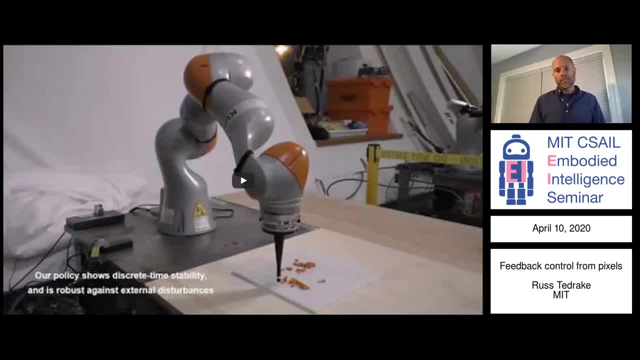 that require them to have access to part of the state that they weren't previously modeling. So do you think there's any room for sort of a goal-conditioned state representation? Is that something that's worth addressing, or is that just too far down the road to be planned? 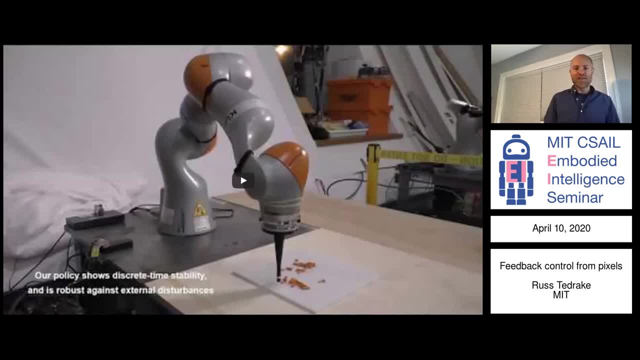 Oh, no, no, Now's the time. No better time than maybe is yesterday. Today is better than yesterday, but Yeah, I think that's one that I really like to think about. I don't know exactly, I mean, I've got. 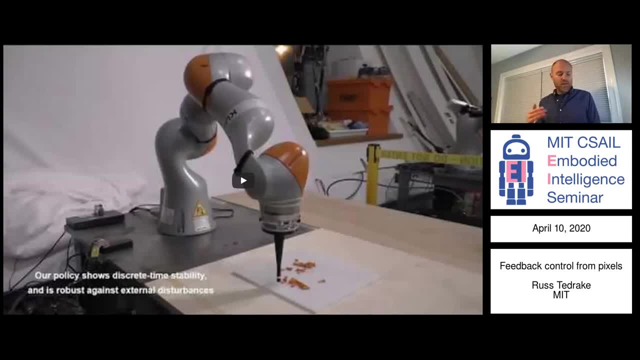 Yeah, so when I'm walking through this room, right, I probably don't think at all. The pencil on my desk doesn't enter my state representation at all, until I go to write something down and then suddenly boom, it's like the most important part of my state. 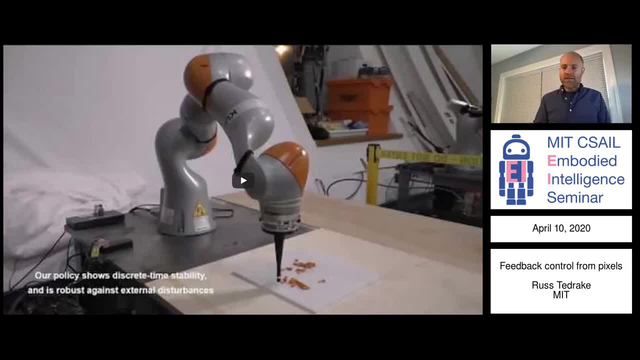 And how do you build these like hierarchical models- This is something that you know Leslie and Tomas have talked about for a long time and you know I am very interested in that- And how do you flexibly go up and down those hierarchies?